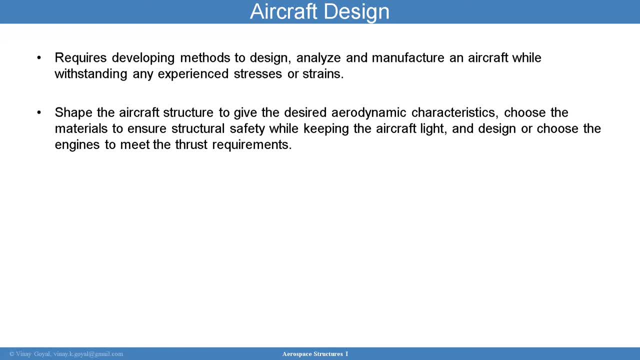 Shape of the aircraft structure is usually given by the aerodynamic characteristics and typically you're really using wind tunnel testing to really validate the loads you'll be using in your design And you want to choose materials, then that will ensure the structural safety while keeping the aircraft light and designed, or choose the engines. 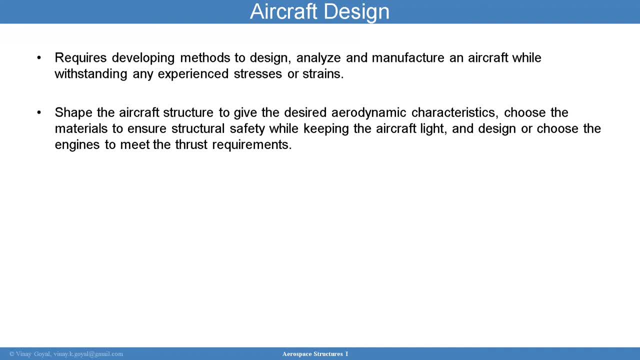 You also have to choose the engines that will meet the correct thrust requirements, So it takes A combination of a multidisciplinary effort, very similar to what we discussed to launch vehicles, where you need a combination of a team that can achieve the desired goal. 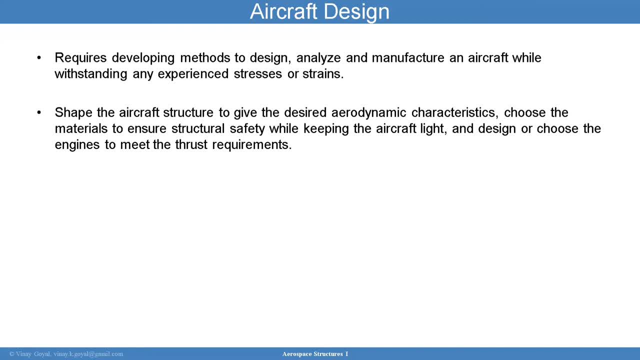 And you're usually going to need the propulsion team, the structures team, the fluid mechanics team and then the avionics team, All of them working together with the systems engineering in combination with the manufacturing team and the designers. Again, All that is required, because if one expertise makes decisions, it will affect other areas of expertise. 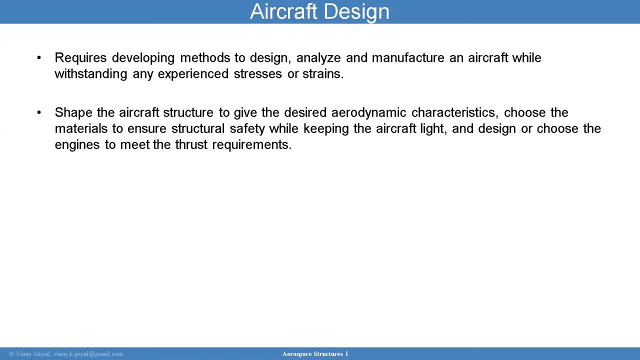 In the aircraft design. what you're looking for, then, is you're trying to set the design goals. So, for example, do I want my aircraft to be a small passenger aircraft, or I want to have a large number of passengers. 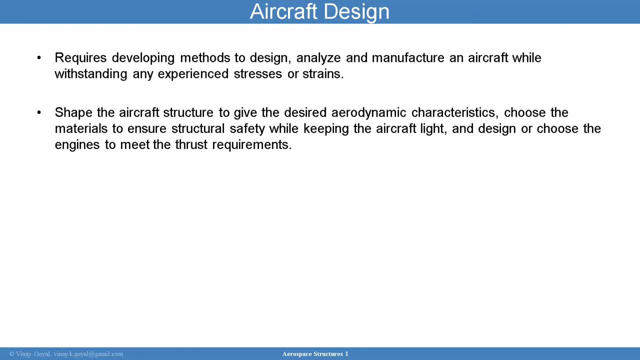 And then, when you're going through that process now, you're looking at really trying to understand the costs and benefits of short flights versus long flights, How many passengers you want to have in that aircraft and you know how many times you want to fly a day. all that plays a role in coming up with a big-picture perspective when it comes to aircraft design. 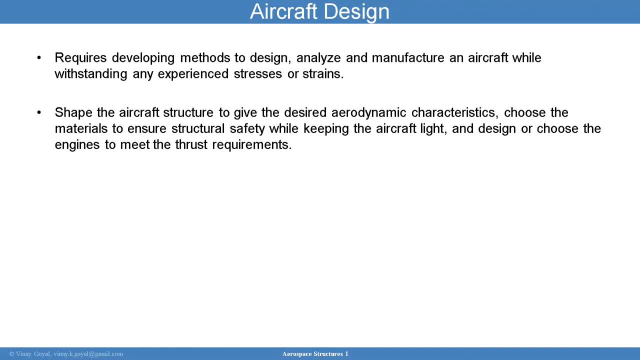 Number two. there then it becomes more about performance. You want to get the best performance because, at the end of the day, the airliner wants to save money on fuel And you also want to then optimize your performance. You want to optimize the patterns for flight across the world and you also want to make sure that you have optimized it per passenger, the cost per passenger, because it's really that that's going to give you the profit. really trying to understand that profit margin. 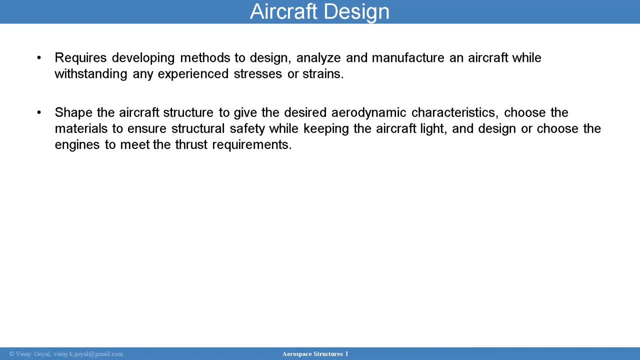 And so that's why it's not just a structural thing, It's not a proportion thing, It's a combination of factors that's going to help you really understand what is required in that design. The ingredients are: It's what you want to have there. 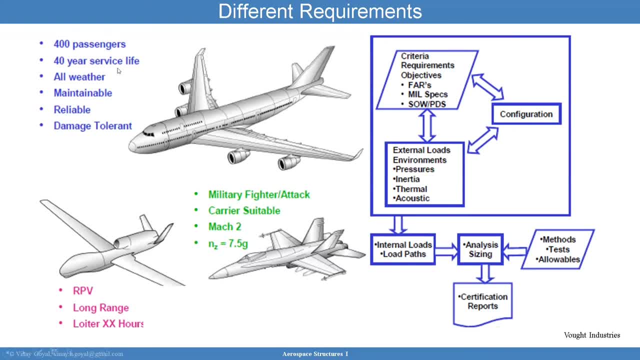 And so here's an example of different requirements you're going to have Here. I have a 400-passenger aircraft that I want to design for a 40-year service life and an all-weather condition aircraft, meaning I can land this beast. 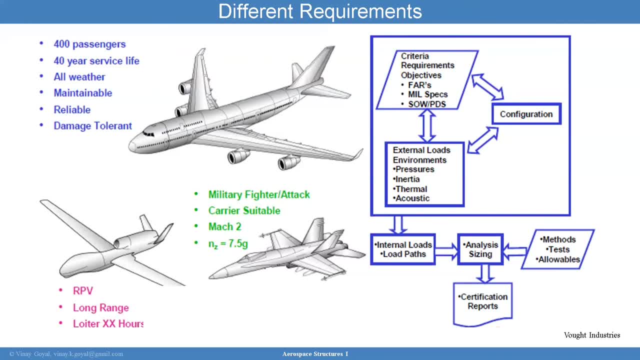 I can land it in Alaska, I can land it in the Death Valley, You know. this aircraft then has to then be designed to weather conditions that could be significant. All weather also means- and we talked about that before- When you want an aircraft to be able to pass water ingestion tests, you want this aircraft to survive a number of conditions that may be not necessary for other type of aircraft that you may design. 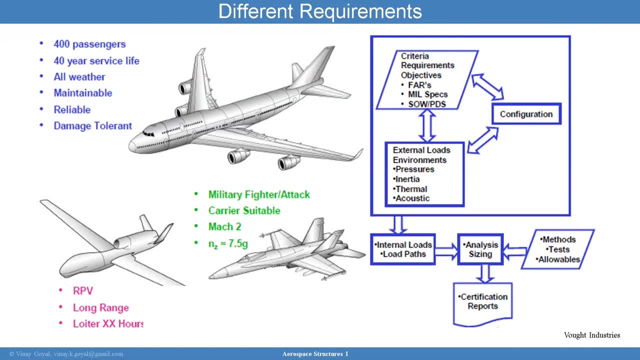 It needs to be maintainable, reliable and damage-tolerant. Then you may have another type of aircraft. It could be a military flight fighter attack system. But then there you're looking for speed or Very low noise reduction at a very high Mach number, with maybe a load factor. 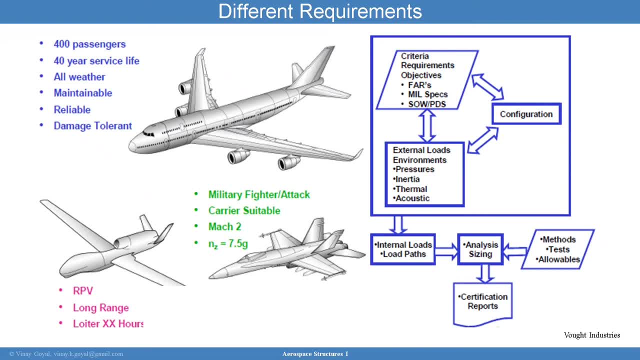 I'll be discussing load factors today, a 7.5 Gs, for example. Or you have a unmanned vehicle, aerial vehicle there. that's a long range. Whatever it is, those requirements need to be put in place first, so you can then design an aircraft that can meet. 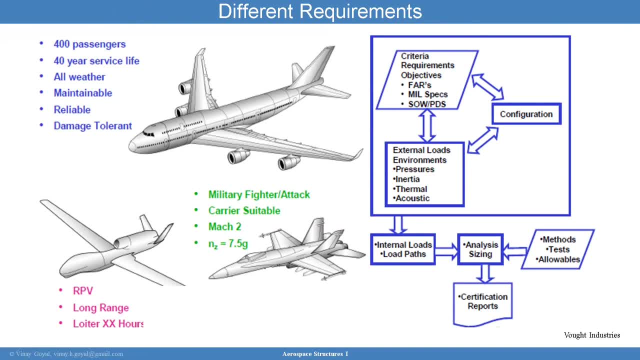 Requirements that we covered in the previous lecture: the federal aviation requirements, regulations and whatever meal handbook specs you need to meet. those criteria need to be designed, But you have to design against those criteria And that means that I need to really understand the loading environment, the external loading environment. 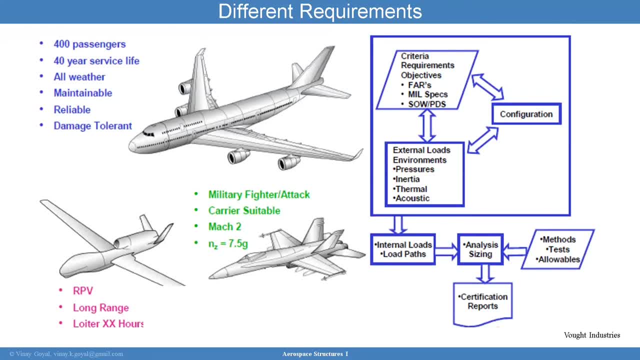 And those external loading environments- I'll be covering that today- will drive, then the environments which are pressure, the fuselage pressure, for example, And then you also have the inertial load, Because every loading condition you have acting on the aircraft is getting balanced by the mass times, acceleration. 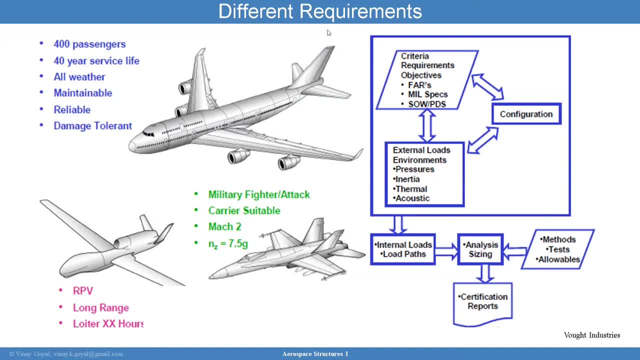 Very similarly to what we saw with the launch vehicle design. We saw that there. We saw how the mass times acceleration really balanced all the loads. When you're landing the aircraft, then you're going to also have external loads From the ground pushing against the landing gear. 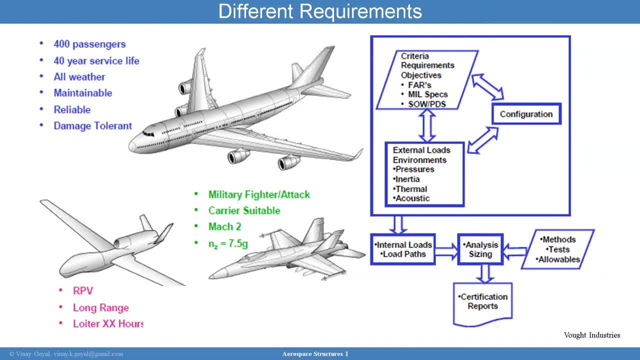 And we demonstrated how those tests can be quite significantly challenging to perform And they're really stressing those landing gears quite a bit. Then you have the thermal conditions, And the acoustic loading is going to cause vibration environments on the aircraft, And so what I really want to do is to characterize the external load environment. 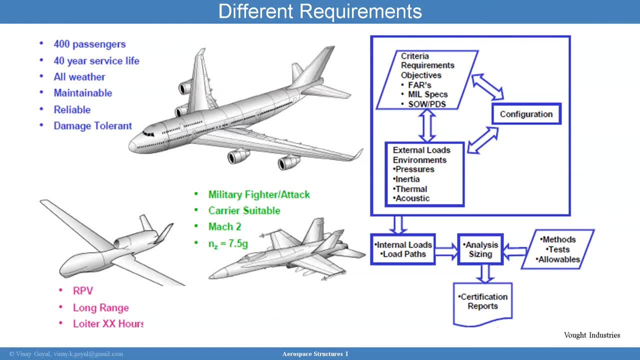 And then determine the internal load paths within the structure, Because those internal loads- And when I say internal loads, what I really mean here- is a free body diagram. We showed you how to do the free body diagram for a beam in mechanics and materials. 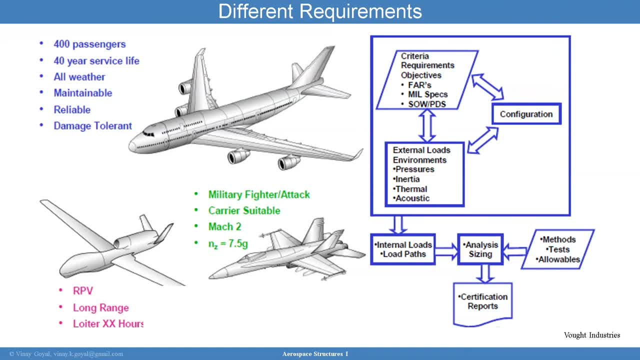 We showed you how to do the free body diagram for creating section cuts on a launch vehicle design And you saw how those internal loads were really generated by the external loads acting on the surface of the launch vehicle And that was really driven by the angle of attack. 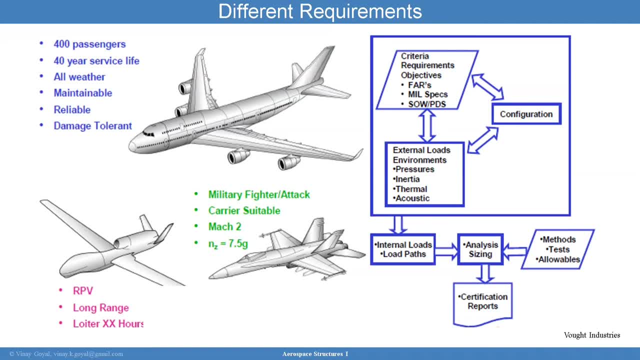 The thrust And then the gimbal loading to balance the fact that you don't want that rocket to start rotating with no purpose, Right, And so those internal loads are going to then help you size the fuselage thickness, the number of stiffeners that you need and then other elements in the design. 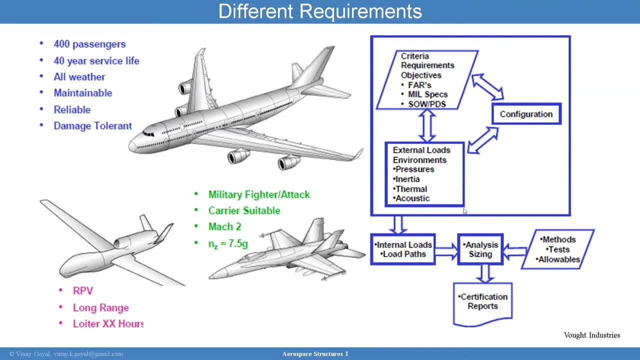 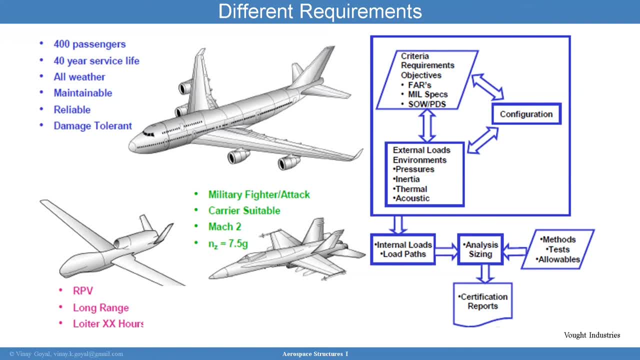 We talked about that a lot, Your allelables. You're going to perform your testing And then you want to then compare your analysis to those tests, to validate those analyses. They're going to help you size the design finally, And then, once you have confidence in that analysis, with the margins of safety factors. 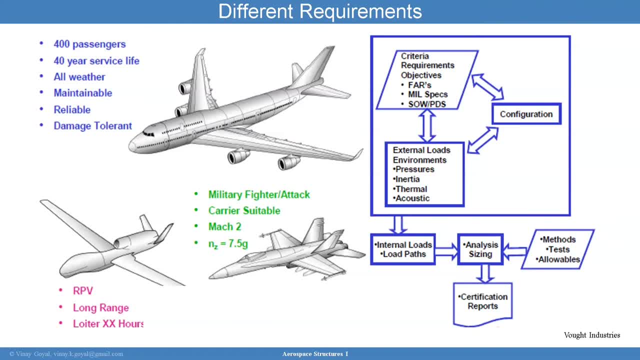 of safety specified, the A basis or B basis, allelables specified. A basis for single load paths, B basis for windows, for all the elements, structures and then with the highest expected loads, which I'll be discussing today, which is differently, if design is specified very differently here, compared to the launch vehicle and launch. 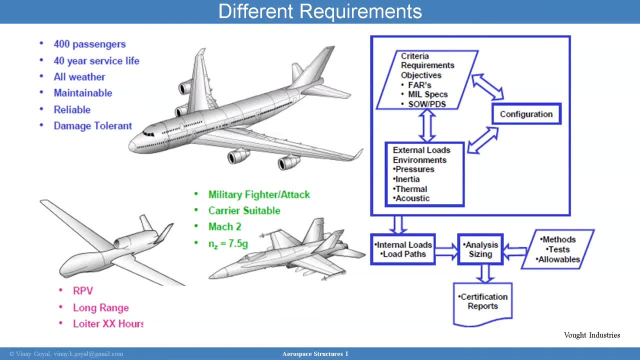 vehicle designs. you're developing that for a 99.90 statistical basis for the loads, and the aircraft design is more driven by the federal aviation regulations which I already covered. but I'll be showing you some of those tables later and then you take that analysis then. 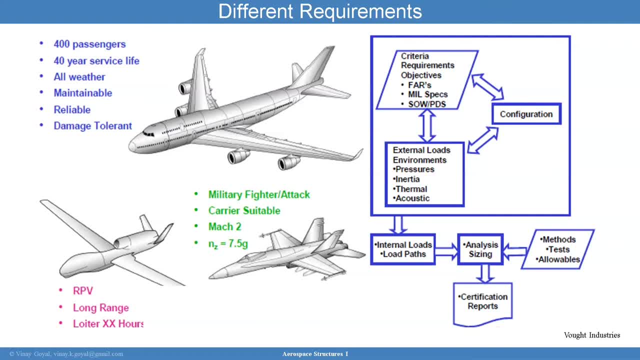 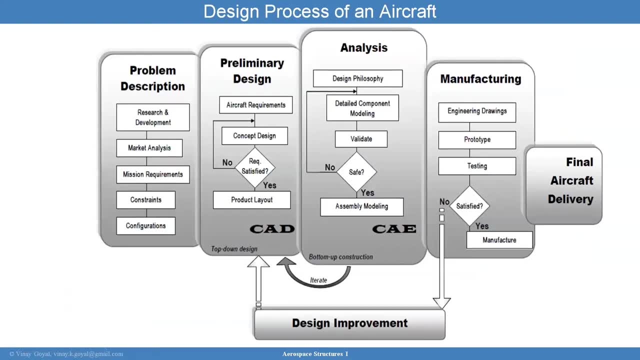 and develop the certification reports that are required. so that's what we got there for, the kind of the big picture there, and then and then. so here the final. the process goes from left to right here and you have the problem description, which typically requires some amount of R&D. you definitely want to keep advancing technology. 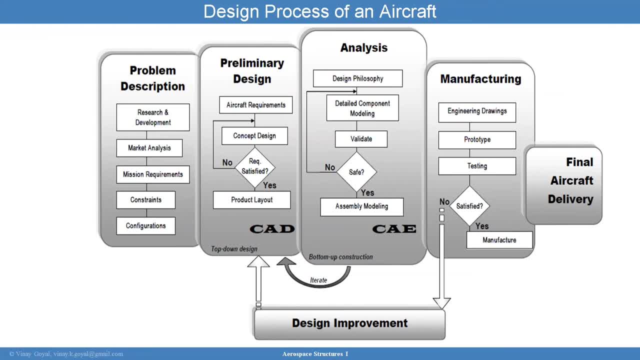 perhaps you have a better wing airfoil cross-section or you have a better profile for your fuselage. maybe the nose design is different, because maybe the nose design will reduce drag. maybe you have a new material system they came up with and that material system can now help you with with reducing weight and giving 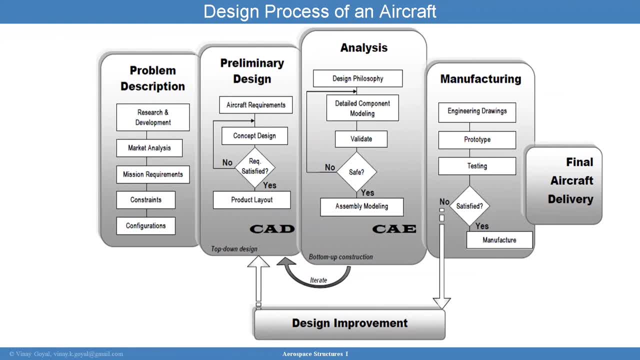 you higher strength and lithium. aluminum is one of such metal that people have been looking at. for example, we have the composite fuselage. design could be unique in the sense of maybe I'm using very, very new fiber systems or metric systems, but that's, that's what we're talking about here when I say R&D. 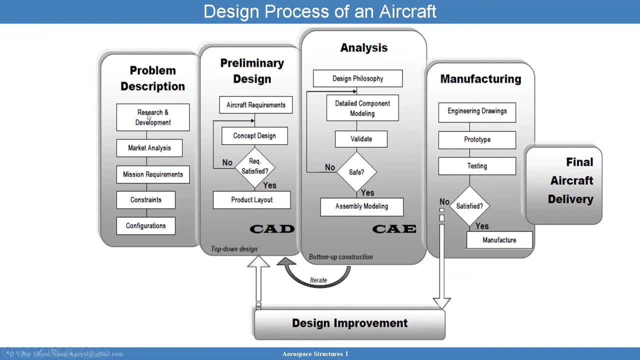 is: what can you do to continue to compete? you know, for example, the competitors. for example would be: for example, you have Boeing and then you have Airbus, and then you have many other competitors, Embraer, for example, or the Canadian regional jets. all these companies are competing. 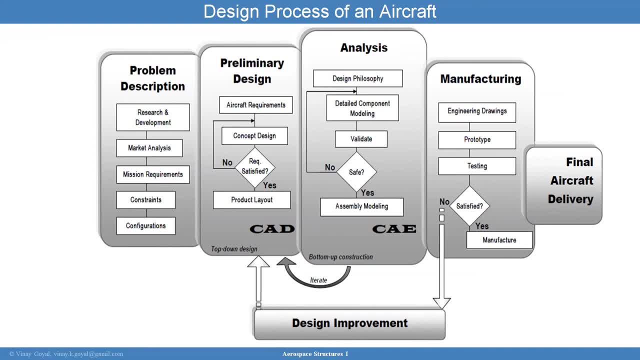 against each other and for you to be so, for you to be able to survive, and you definitely want to invest money on R&D, to keep pushing the technology, to keep reducing that weight, and a lot of people say, well, you know, I don't see how we can keep improving. 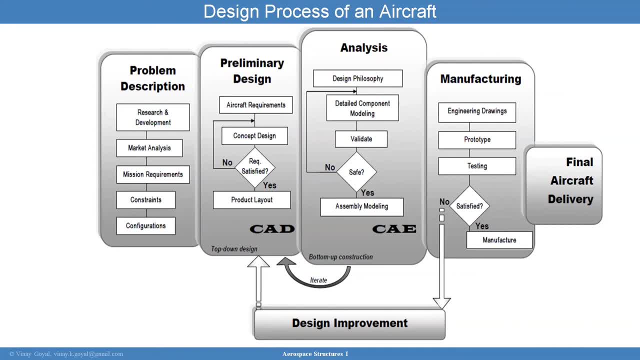 but no you. you can continue to improve, and the ways you can continue to improve is: perhaps your technology has advanced to the point that you can reduce weight, for example, or maybe you can even drop. I'm not suggesting that we drop the factors of safety, but you've increased your confidence in. the in the analysis and the test appreciative way. Okay, Okay, All right. OK, Throughout the program, All right. Well, that's really the point. $49, you're welcome to watch. Here we go. I'm gonna take aренve Olympia, blast button many weeks, which is the blooming yolk国 in therian Mioreo. a ph meant very surgery-influenced donor, our first project next time. 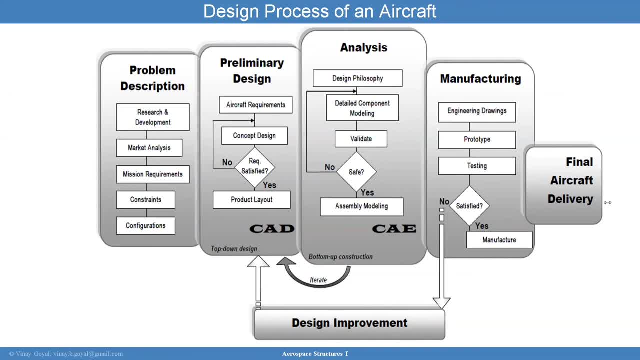 approaches to the point that you feel like you can now basically do that okay. and then you have the mission requirements I talked about. you know you want your aircraft to go from here to Europe long distances or you want to go short distances, and then your constraints and configurations, all that. 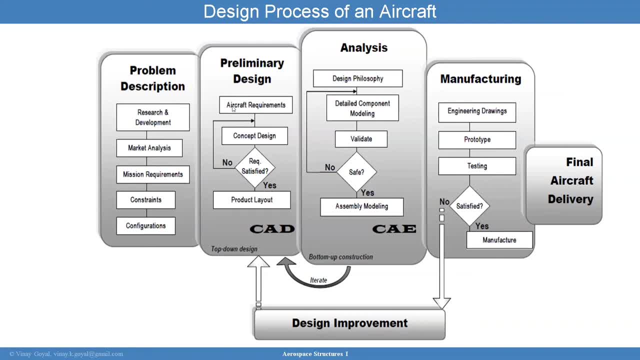 goes into your preliminary design. you have your aircraft requirements and then you want to make sure that your concept design, initial concept design, preliminary design, will then meet the specifications, at least at the first level view, and then you can outline your layout, your product. that means you know. 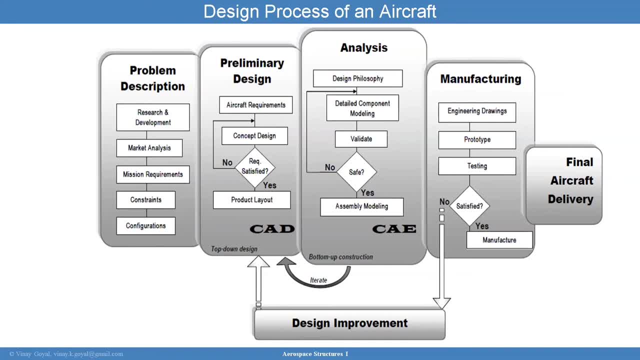 the seat, spacing the aisles, you know how, how space they are between rows and things like that- the pitch they call it. and then you go into your design philosophy and does your analysis. there you do detail component modeling, your validation and, if it's not safe, based on the 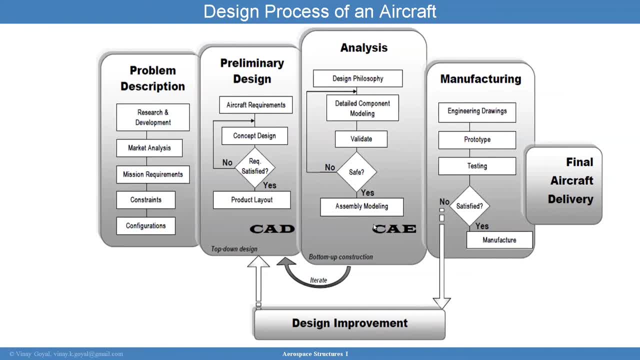 analysis in itself. you're gonna have to make sure that your design has a standard you've done, you have to kind of redesign and then go into assembly modeling. Once you have this going through the critical design review and you've gone through some amount of testing from the building block approach we discussed earlier, then you can. 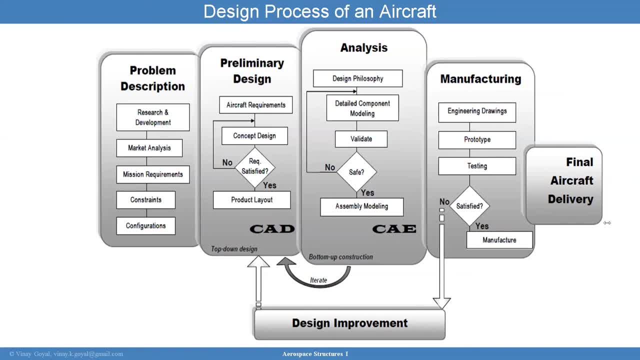 take that information and you can now plug it into your manufacturing And the idea then there is to then manufacture your components and hope that your manufacturing after I go to the test program, that that testing is looking good, Because if you're satisfied you're ready to manufacture for aircraft delivery. 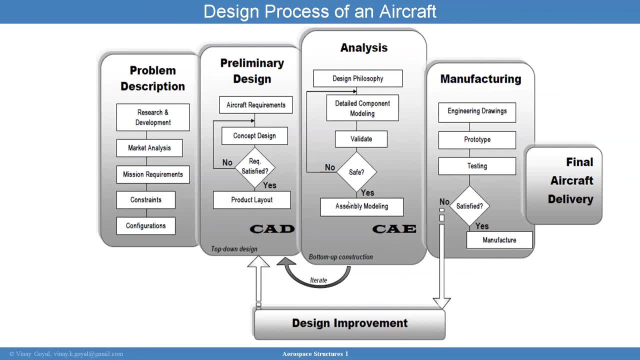 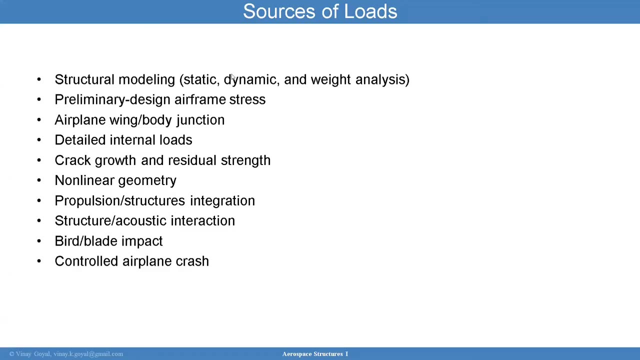 But if you're not satisfied, you need to start looking at a design cycle. that can sometimes be significant And it's going to take you from manufacturing to analysis in several times until you get it right And so, moving along, here we have the sources of loads that we want to discuss. 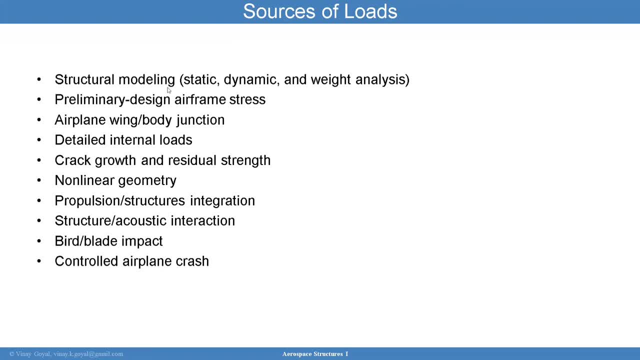 And the sources of loads can come from static dynamic weight analysis And then you have the preliminary design of the airframe stresses. That's going to you're going to have to consider additional sources of loads when you do that preliminary design. 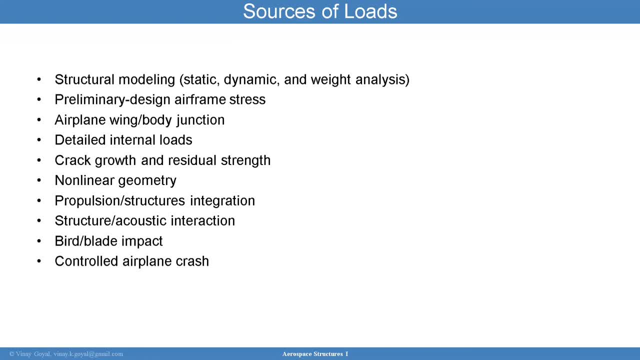 The airplane wing body junction. that location where the wing connects with the fuselage is actually one of the areas that's very challenging And we've already discussed some of that. But I just want to point out detailed internal loads are very important. 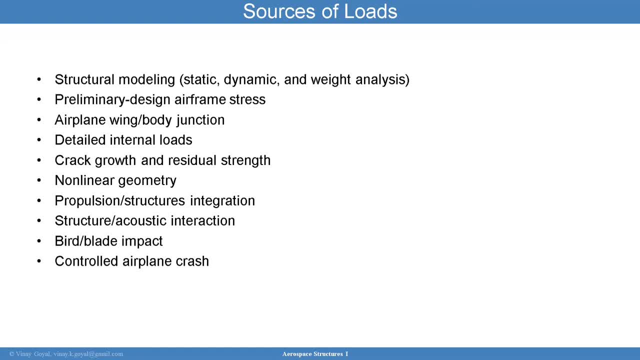 Crack growth and residual strength analysis, nonlinear geometry, And you have to account for the proportion, structure interaction, potentially the structure acoustic interaction and the potential for bird impacts onto the engines. And then you want to definitely want to prepare yourselves And you want to make sure your aircraft has a good, good design philosophies when it comes. 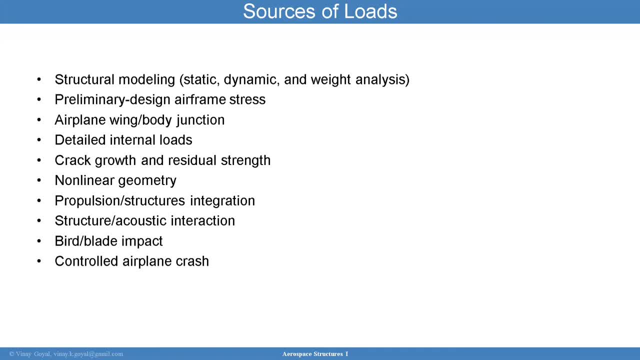 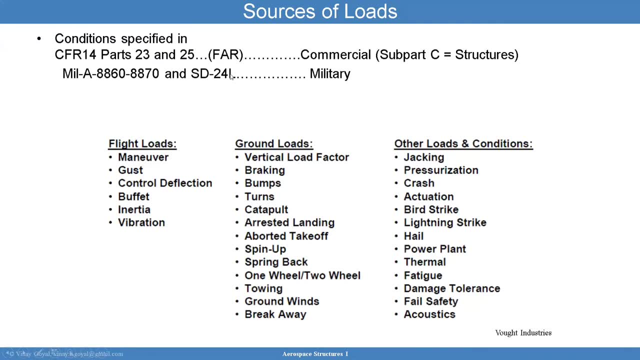 to airworthiness, crashworthiness. We want to make sure it's good for crashworthiness requirements And so the sources of loads, the certifications and conditions are typically provided in the CFR 14, part 25 and part 25, for those regulations. 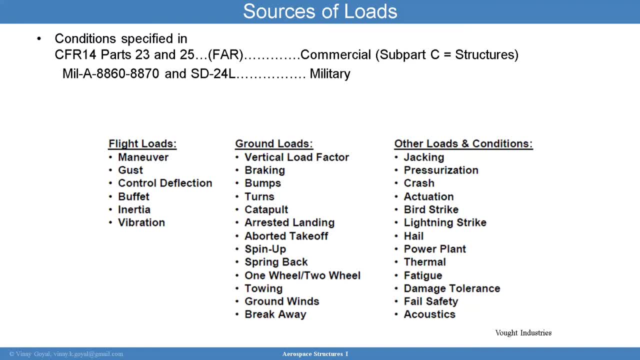 The commercial here. when you see C, that means subpart C, That means commercial, That's structures. And the middle handbook- 8860, 8870, provide the additional recommendations For military applications. But here's the loads, how you can break them up. 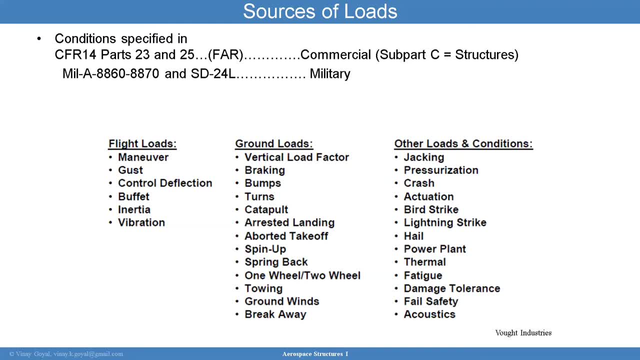 And I'll group. I like to group them into three groups: One is flight loads, One is ground loads And the other one is other loads and conditions For flight loads. you're looking at maneuver, gust control, deflection, buffet, inertia. 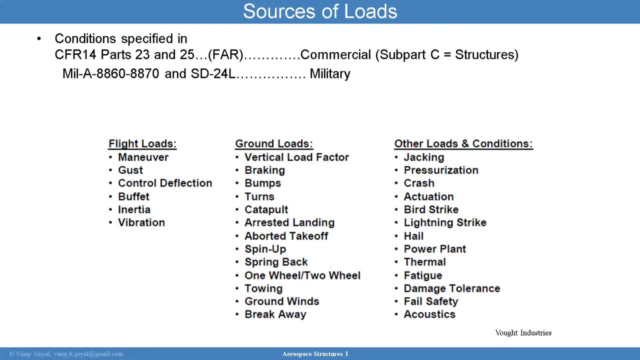 and for vibration, And then for ground loads. you're looking at vertical load factor, the braking, the turns. when you're turning an aircraft you're going to put a lot of load, catapult, A rested landing, a boarded takeoff. 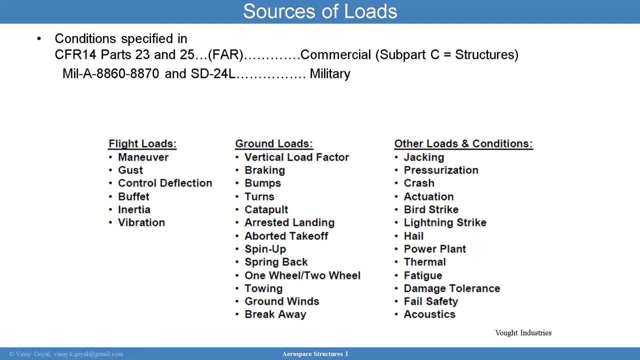 By the way, I experienced an aborted takeoff. It was not fun. It was a LAX Spin up, spring back and I'll be covering the one-wheel and two-wheel landing coming up towing ground, winds and breakaway. 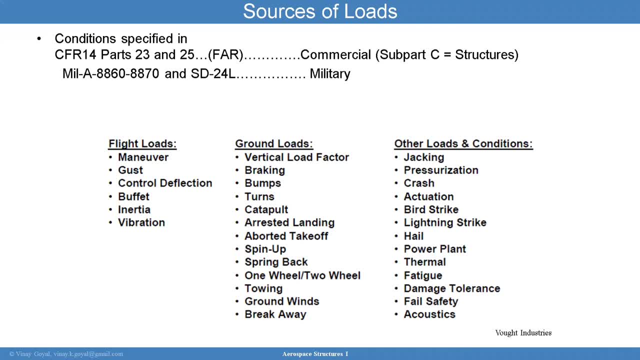 And then you have these other loads that need to really be considered. that can be extreme. You have jacking. pressurization is not extreme, is going to be common crash actuation, bird strike And bird strike. what you want to do there is: do a lot of testing to see if your structure 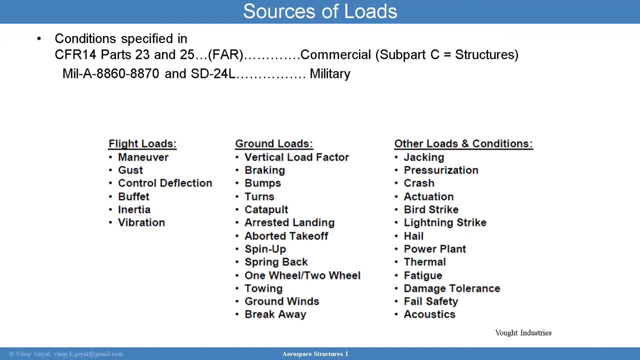 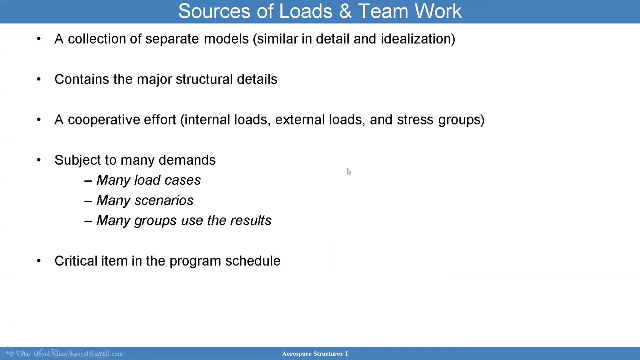 can survive those conditions: Lightning strike, hail, power plant, thermal fatigue, damage, tolerance, fail safety and acoustics. Okay, Okay, Okay, So a collection. so how does this work? It does require teamwork, because you're going to have a collection of separate models. 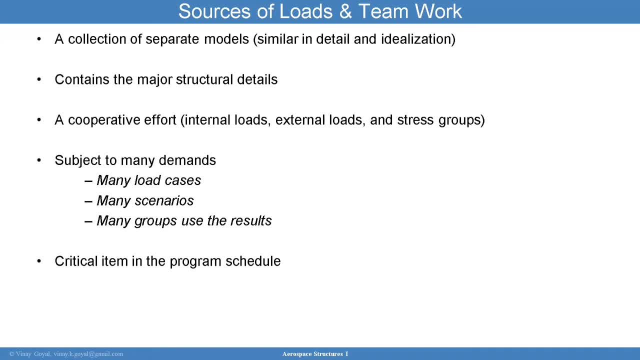 It will contain major structural details and it's going to require cooperative effort- internal loads, external loads- and it's going to involve stress groups And there's a lot of demands here. You're going to have at least 100 load cases, a lot of scenarios, engine out landing. 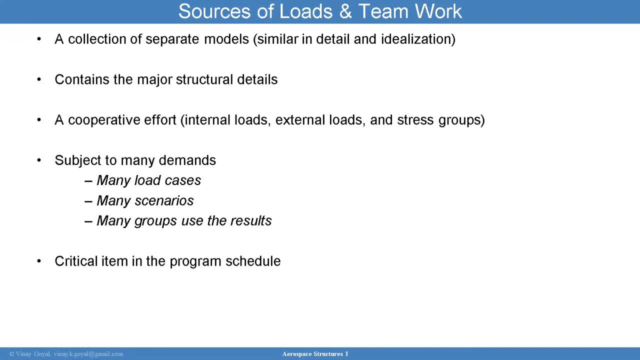 loading pull-up maneuver and so pull-down maneuver bank. So a lot of different load cases need to be looked at and many groups have to use those results. So you're looking at a major organization required to really be able to keep yourself. 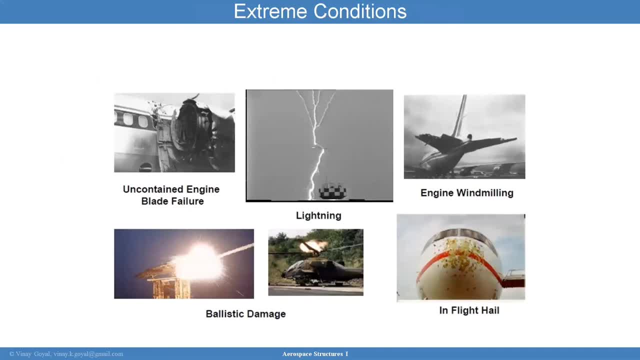 in the program schedule that's required. The extreme conditions I was talking about you need to be prepared for and for which testing is actually required and covered lightning and the federal aviation regulations already. But you have the contained engine failure so you can have a blade. 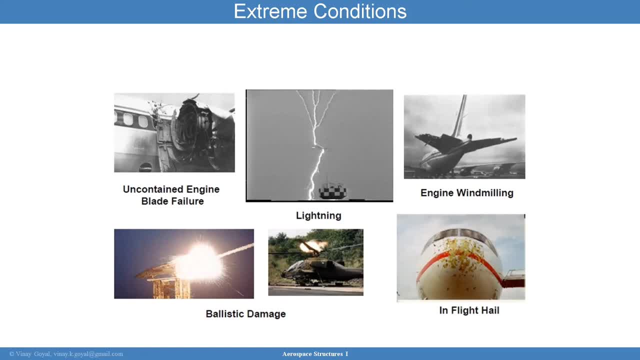 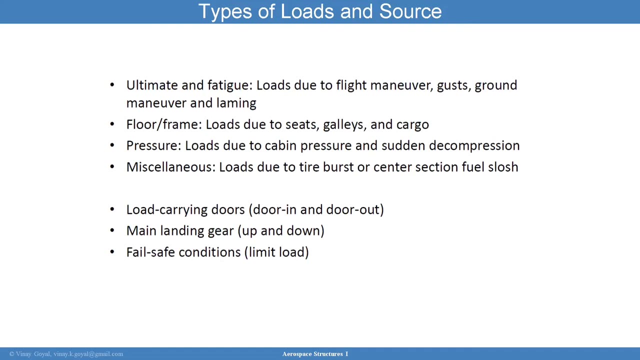 that basically goes flying and hits the fuselage. You want to make sure that the fuselage can survive those conditions: Engine, windmilling, flight, hail and then ballistic damage, Types of loads and sources. again we're looking at ultimate and fatigue. 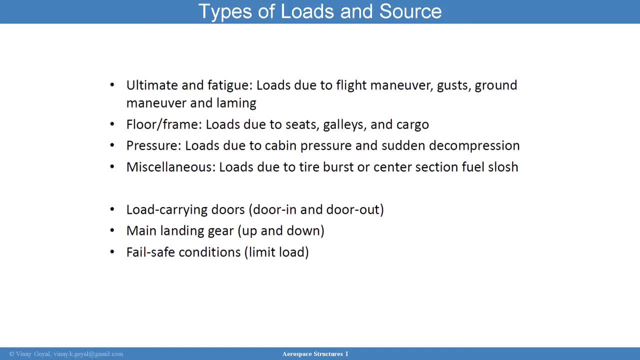 You're going to have the floor and frame, for example. there you have in the floor and frame, you have people walking, you have the seats, you have the galleys, you have the cargo, and then on top of that you have to add the G loads. 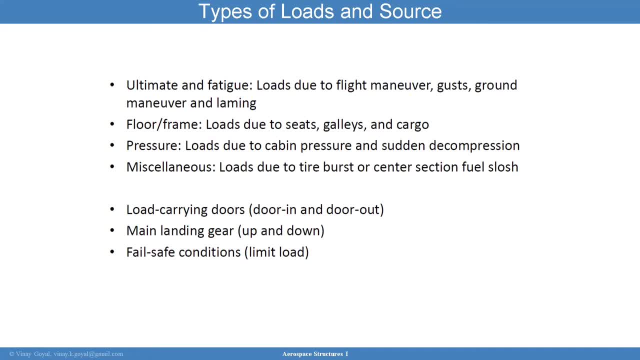 Because when you're flying a cruising altitude and everything's great, you know no turbulence, nothing. that's 1G, That's your load factor. When a lift equals weight, that's your load factor is 1G, But in reality, in reality, you're going to have a situation where you may have extreme load. 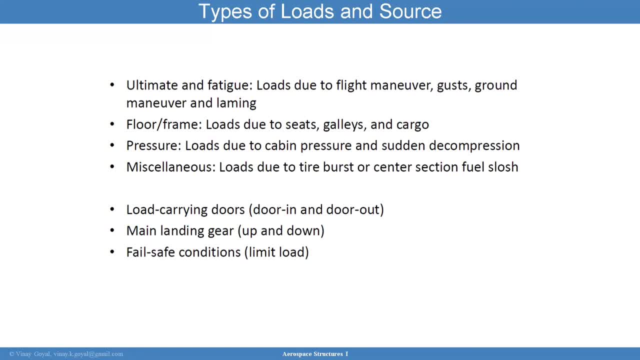 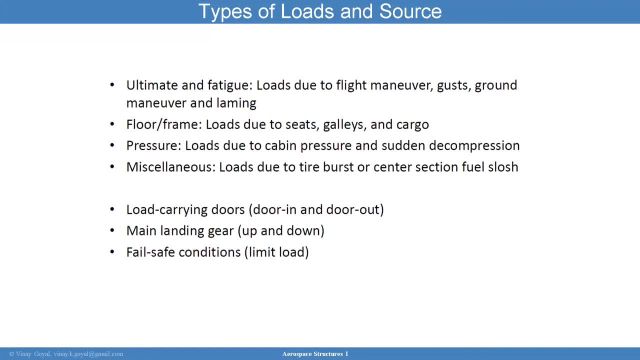 And that can happen. say, for example, the aircraft has to descend very dramatically down from 35,000 feet down to 15,000 feet. Well, you're going to feel a lot of G loading. Well, that flooring needs to be designed with beams that can take those loads, including the G loads. And when I talk about ultimate fatigue, I'm really talking about including flat maneuvers, gusts, ground maneuvers and landing. The pressure loads also fluctuate Every time you take off and land. you have one pressure cycle And the loads do provide a lot of stress onto the fuselage skin due to the cabin pressure. 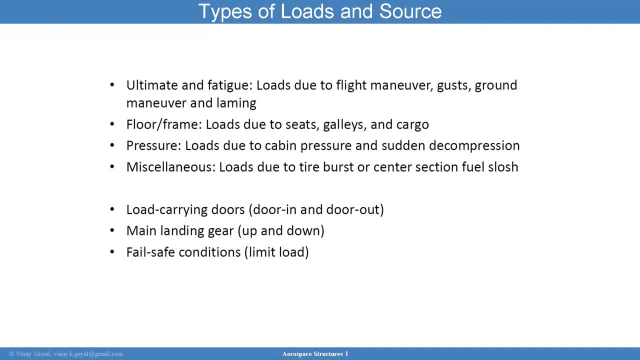 And then you also have to design for sudden decompression, because you don't want the whole fuselage to basically collapse due to this sudden decompression. So it's very important Those stiffeners around the aircraft are really providing that shape so things don't collapse on itself. 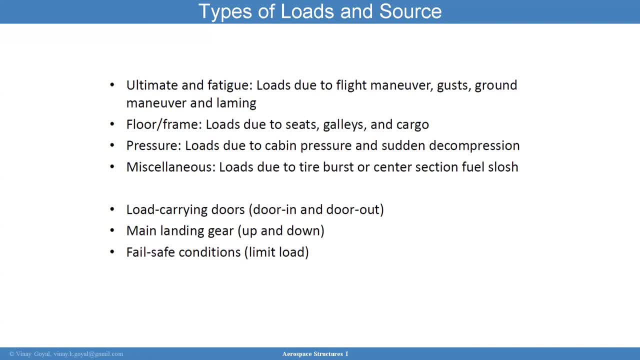 You also need to make sure that you can survive tire burst pressure. So if one of the tires blows up or we have a burst of the fuel slosh center section, that you can still land successfully with no issues. Load carrying doors you're going to have- we talked about that before- main landing gear. 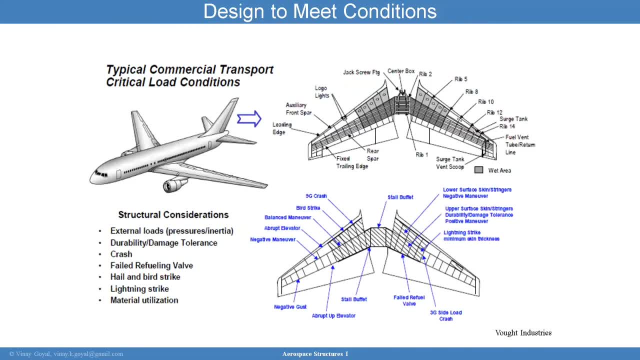 And then you have the failsafe conditions we talked about, And we also talked a little bit about the structural considerations, And these are more of a reminder: you need to design to meet certain conditions. So you have the external loads, you have the debris and damage tolerance, you have the crash. 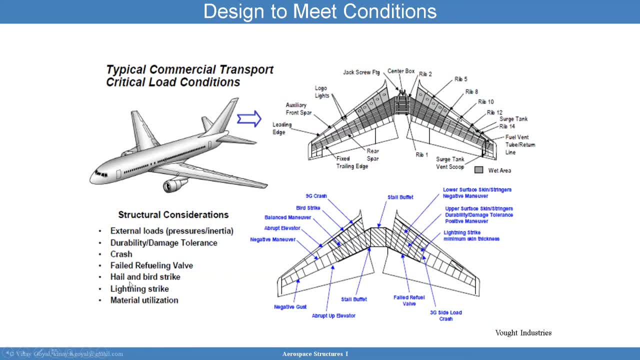 And then you have the failed refueling valve, And then the hail and burst strike, lightning strike and material utilization. So these are the considerations that you need to take into account, And a lot of this needs to be taken into account in relationship with what your design looks like. 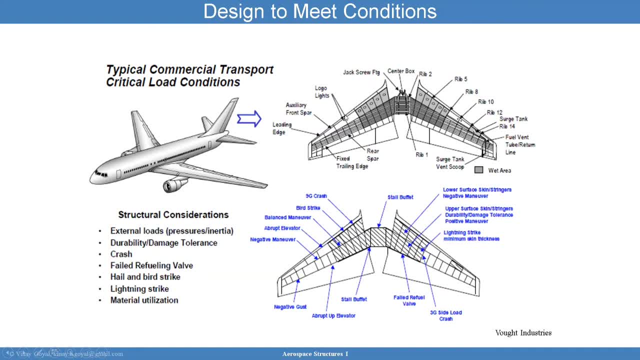 For example, you have a rigorous part here, You have the logo line, You have the lights, You have the auxiliary front spark, You have the leading edge, And all those components here need to be mapped against the failure modes of concern like burst, strike, crash, lightning damage and so forth. 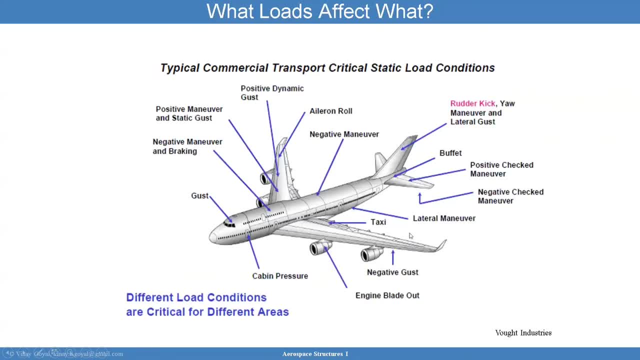 I already covered a lot of this, So again it's just a reminder because it's been a while since I last covered it. And then here is what loads affects what We talked about: the aileron causing the roll. You have the negative gust. 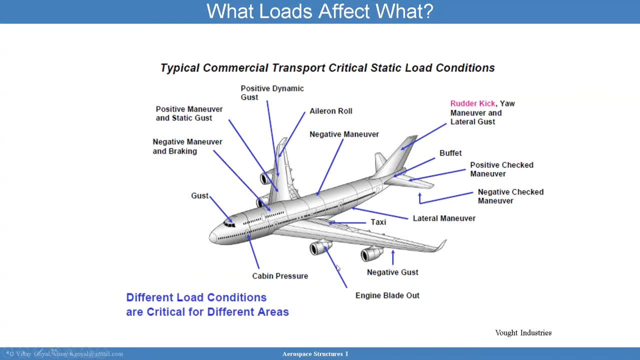 And I'll be covering gusts today. You have your engine blade out, You have the cabin pressure. Your gust also affects this front section. here You have the rudder kick the yaw maneuver and the lateral gust will be a problem. 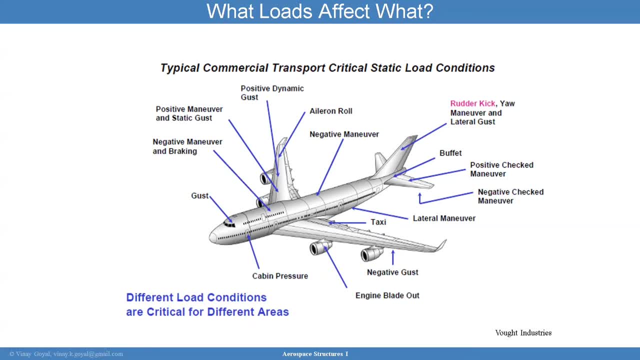 And in fact that's one of the things that may have brought the American Airlines aircraft down. when the tail broke, for which Dr Raju and his team performed a significant, he was part of the fatal investigation. They helped resolve it. Buffet loading. 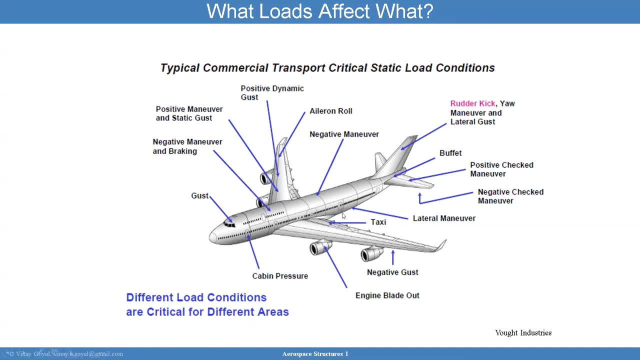 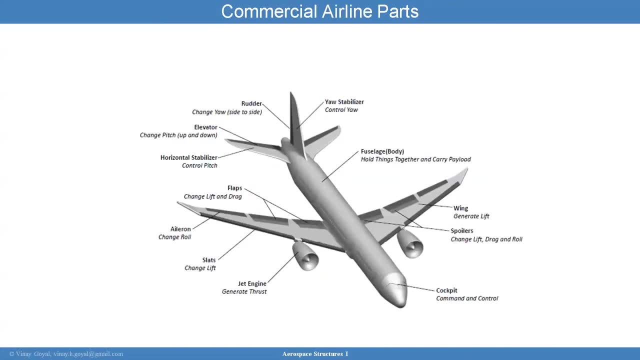 And then you have your negative and positive maneuvers. All that needs to be accounted for in your designs And I'll be covering some of that today. Just a reminder: what are the inputs? So you have your inputs here. The spoilers here are changing the lift, drag and roll. 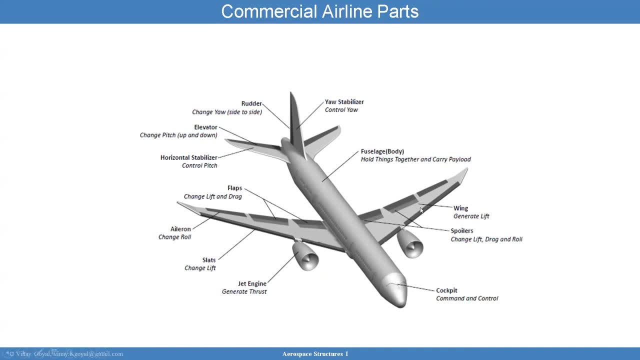 And the wing here will generate the wing. Sorry, the wing generates a lift And the spoilers. By increasing and deploying the flaps, I can now increase lift at lower altitudes, Because when you go to lower altitudes you have to go slower. 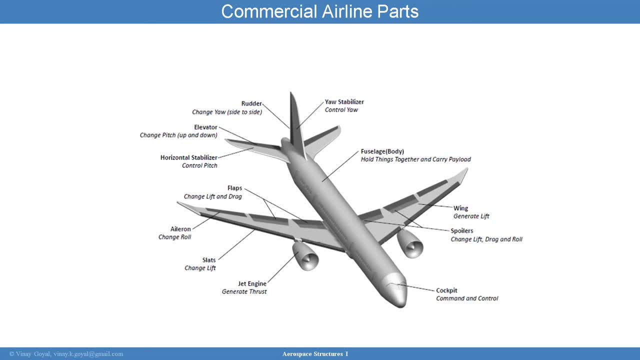 And if I go slower, I have smaller lift for the same wing area. So I really need to increase that wing area And to do that you can either use morphing technologies or just deploy your flaps to be able to account for that. 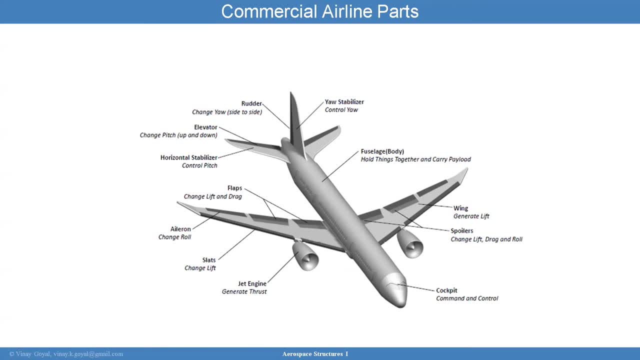 The aileron will provide that roll that you need: The jet, The jet engine provides the thrust, And then you have your horizontal stabilizers that provide the control pitch and the elevator as well, up and down, And the rudder provides the side, the yawing right. 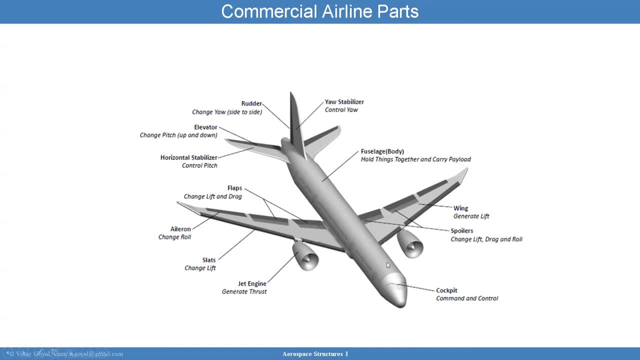 And so then, these are your controls, And all that is providing loading into the structure. Now, the good news is, in a major aerospace organization, they're going to have experts in the loads arena, in the fluid mechanics arena, So you're going to know exactly what conditions to design for. 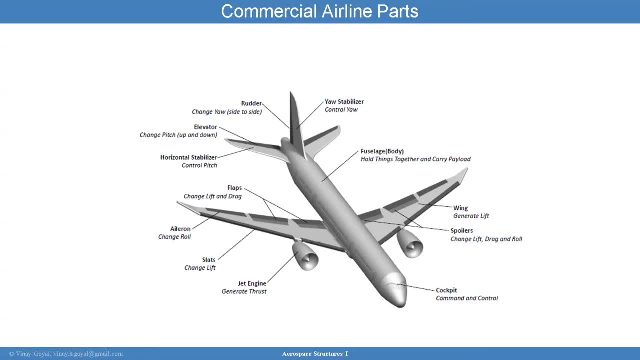 You're going to know what conditions to design for And you'll be able to tell: okay, well, these are the loads I need to apply to this rudder. These are the loads I need to apply to this horizontal stabilizer, and so forth. 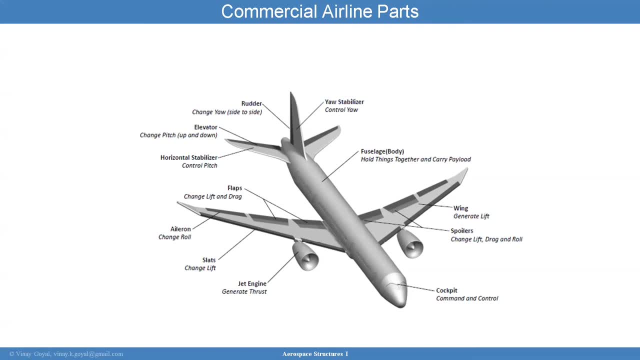 And then you can then use the free body diagram approach to then go in and design that. I'll be covering that in the next lecture that will be posted in a couple of days. How to do that. I'm going to do that in a deeper level, top level view, but deeper level enough that covers. 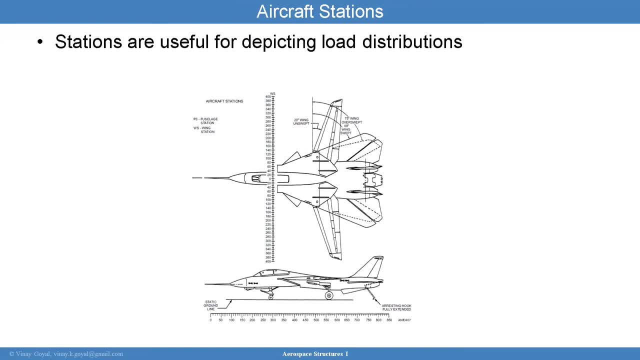 the equations in the book. Here is an example of what people typically use in the designs. We like to have aircraft stations because typically aircraft design is not. the analysis is not done by a single person, Typically is the responsibilities for the analyses are typically distributed across. 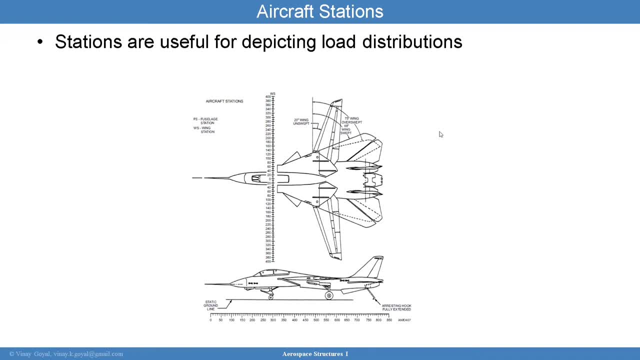 multiple people, It typically will work, And so, therefore, you need to have the stations defined so you can tell people what they're responsible for. It also helps you with plotting free body diagrams, and everybody knows well, okay, the highest stress is about this point. well, that's about 500, I forget the units here. 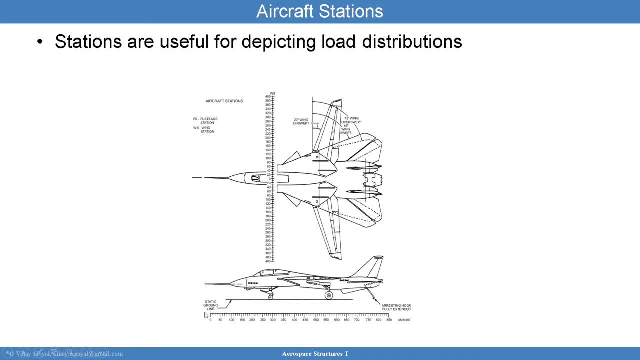 but it's about 500 away from the tip. So that's where that becomes important in the design. Let me tell you a little bit about this. Let me tell you a little bit about this. Let me tell you a little bit about this. 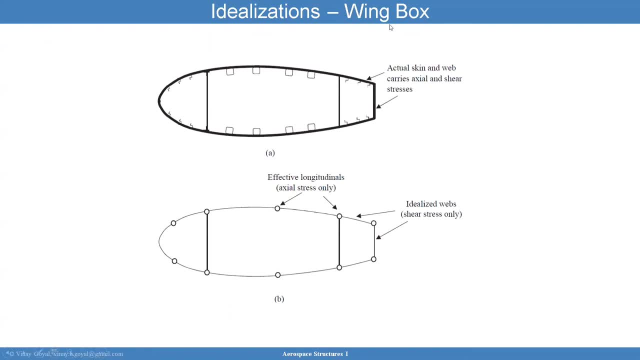 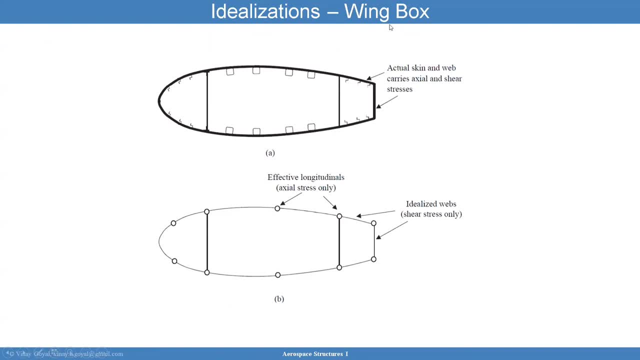 And we'll continue. Thank you, Thank you. And so you can idealize a wing box. Typically, a wing box is going to be comprised, for example: this is a wing box here And this will be a part of your design to make sure that the wing can take the loading. 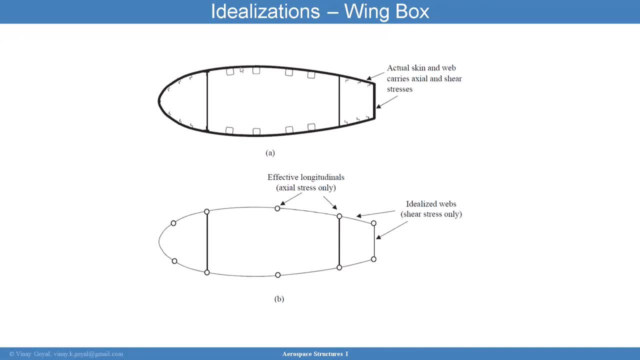 conditions that it will experience, And typically you're going to create a free body diagram of that wing, and those free body diagrams of that wing will give you shear moment and that's what you're going to then use to analyze this cross section. 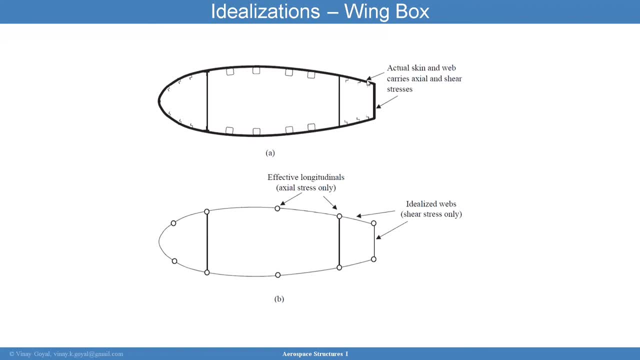 The actual skin and the webs typically carry the axial and shear stresses and in some designs, what you will do, in some analysis, what you will do, you will simplify the design that's covered in my book quite a bit. you'll simplify this and there's even an example. 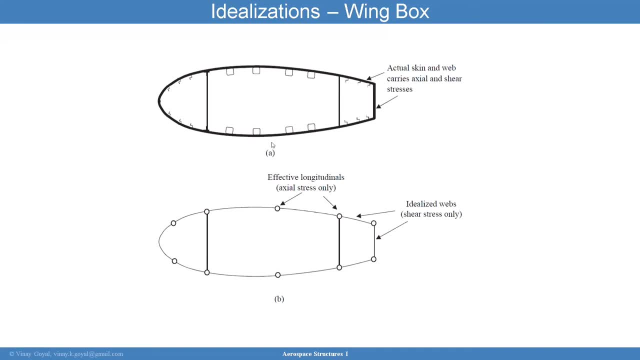 on how to do it. You'll then take this design and simplify, and then here these locations take only axial stresses. So I'm basically simplifying the model a little bit more, And then here the walls take the shear stresses only. 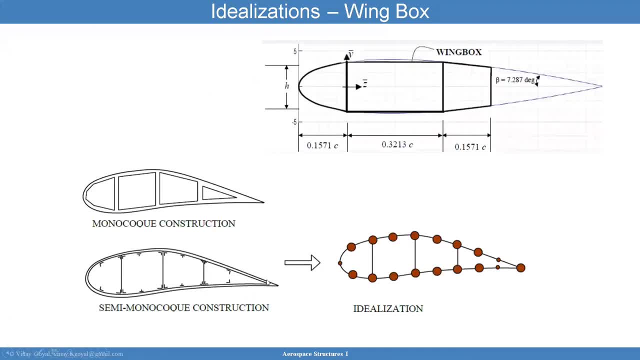 So that's typically the way you approach it. You can see wing idealization. This is straight from one of the books and you can see. you know the design looks very complicated: Semi-monocoque or monocoque construction Typically. the design will look complex, but you can idealize it in a way that, where these 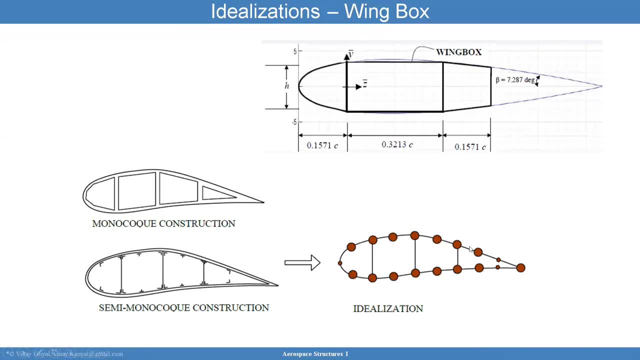 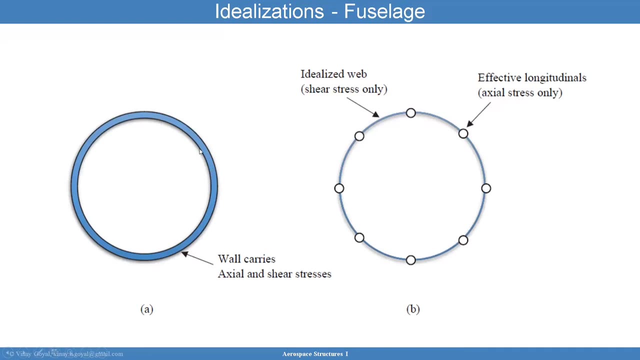 booms can take the tension or compression loads, and then the skin takes the shear load And you can quickly calculate what the stresses are in the skin versus the booms. Okay, So for the fuselage. very similarly, you're going to have the fuselage with the stiffeners. 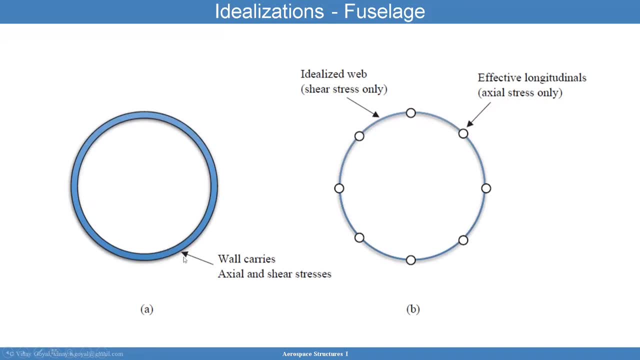 in them. The stiffeners are not, are missing here, but the wall will carry the axial and shear stresses. And what the modeling simplification is? typically that you will go ahead and model it with booms again, And these, these booms are taking just tension and compression, while this can only take shear. 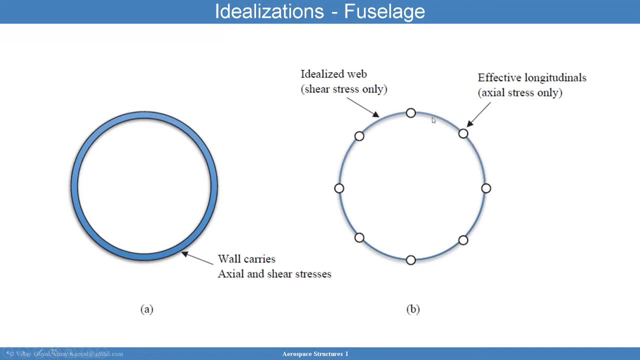 stress. This is typically the approach. And then in top of that, on top of that, not only have the skin stress from shear. then you have the fuselage pressurization of the Delta P across the fuselage, because as you ascend right, the internal pressure, the cabin is pressurized to 78 PSI. 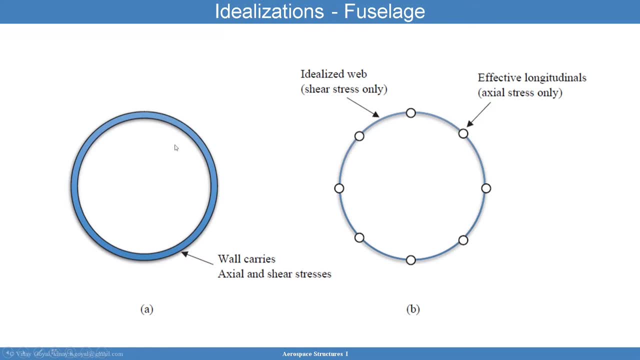 So you have a pressure differential across a wall that causes the, the, the fuselage, to expand. So when you combine that with the shear stresses from the section loads, Okay. So when you combine that with the shear stresses from the section loads, those need to be considered. 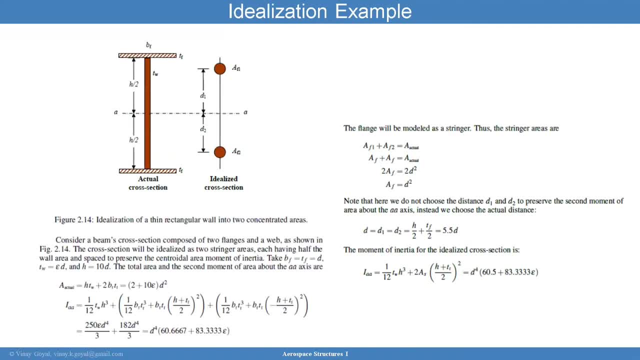 in the analysis. Here's an example in my book and it shows an I-beam cross section and the I-beam cross section in the figure 2.14 of the book has been simplified so that it only has two booms and then this section here. 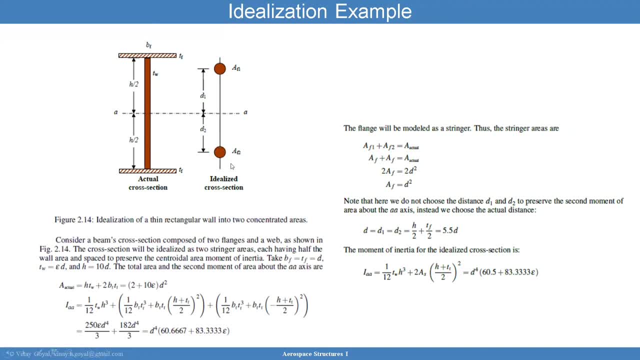 And what you're trying to do really is to come up with an equivalent model that gives you the same response as the actual cross section. You can see here that with the modeling simplification, if you follow this, I don't want to cover this. 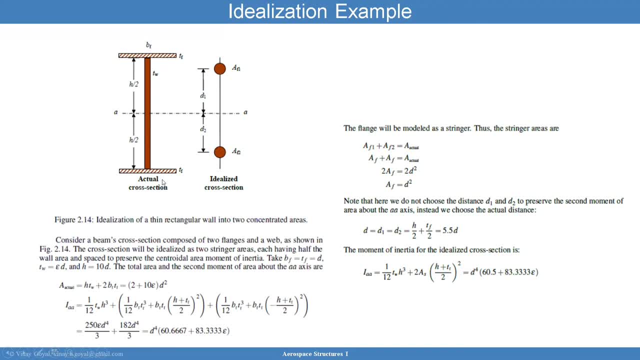 in extensive detail, because you don't have to calculate the inertia of an I-beam. All this should be fairly simple, And to calculate it using the approach that I'm showing here- this idealization- is not very difficult. Just come up with a equivalent area that should go here to give you the closest answer as. 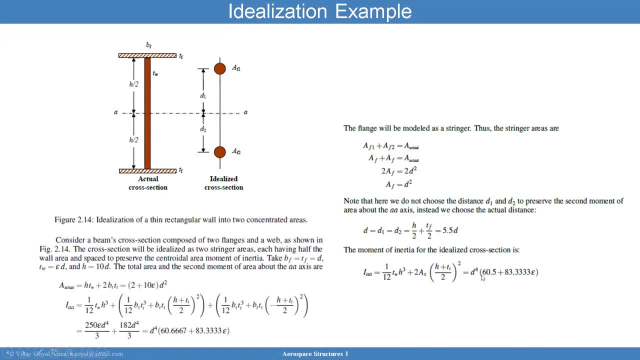 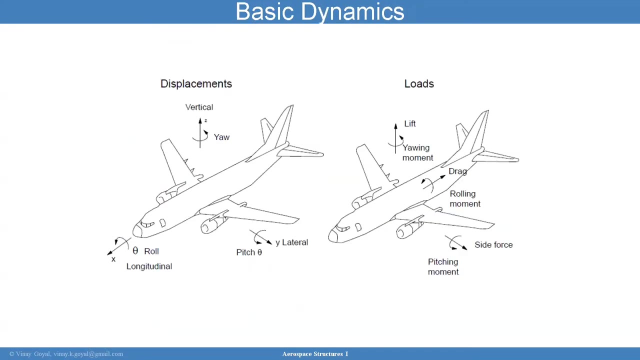 the inertia here And you can see here that you get really close: 60.5 versus 60.67,, 83.33 versus 83.33.. So the inertia calculated with this method versus the ideal cross section method gives you very similar answers. 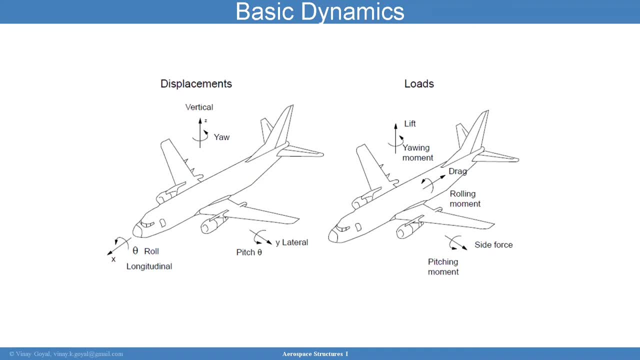 And these are the basic dynamics. I'm just showing you more of the corresponding displacements and loads. You have yaw That goes with yaw moment. You have vertical deflation: That goes with lift. You have drag That goes with the longitudinal direction. 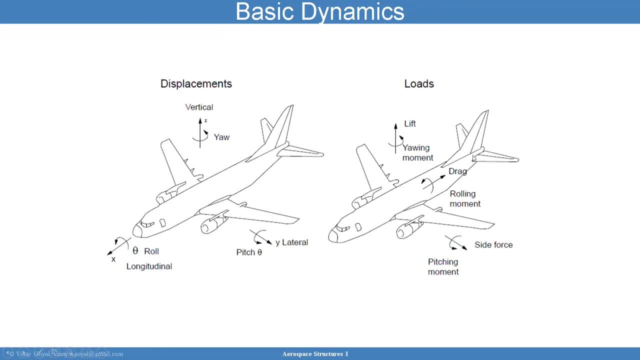 You have theta That goes with the rolling moment, And then you have the rolling moment goes with the roll here theta, And then the theta goes with the pitching moment And then you have the yawning moment already covered. So typically that's what you're going to see in different books. 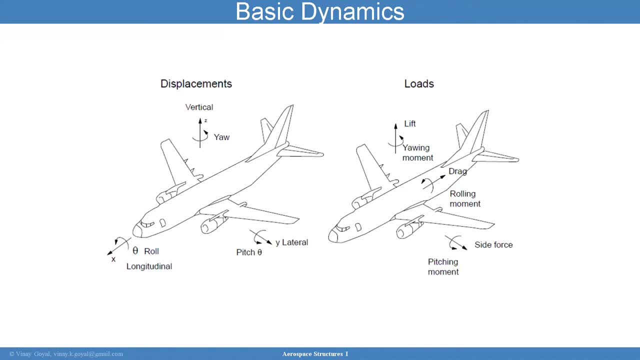 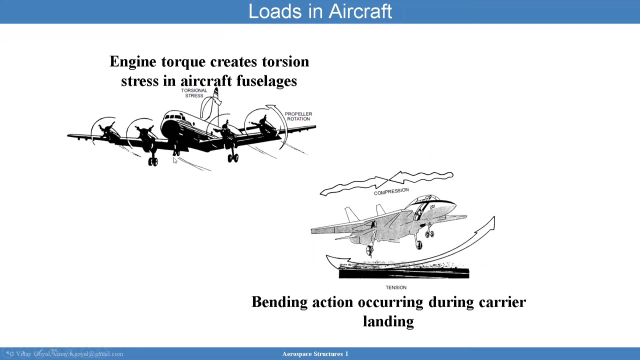 And you're going to have a coefficient of lift, a coefficient of drag, And then sometimes you have coefficients of moments as well, And those are really all calculated, And they're calculated through wind tunnel test data. So more loads on aircraft, The engine torque creates torsion. 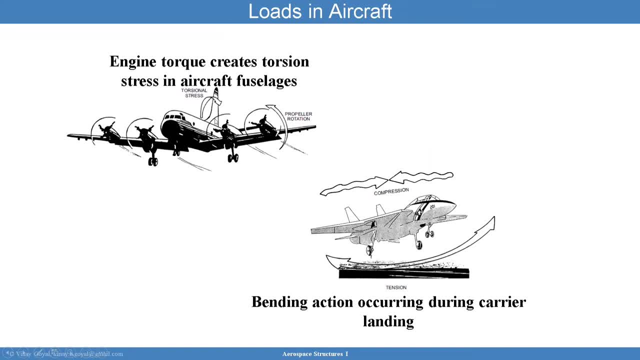 When you have these engines operating you'll get some amount of torsional stress. And then when you have an aircraft, say, you have a pull-up maneuver: 60.5 versus 50.88.. in those situations you have compression at the top and tension at the bottom. 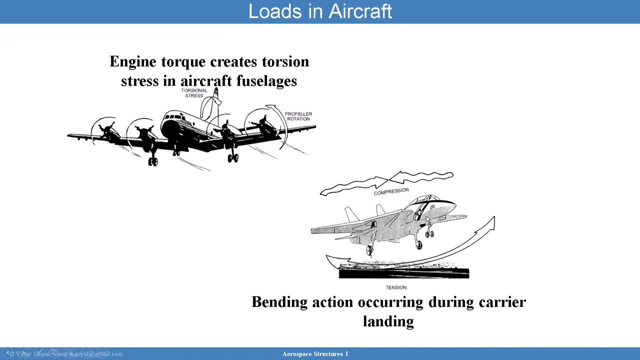 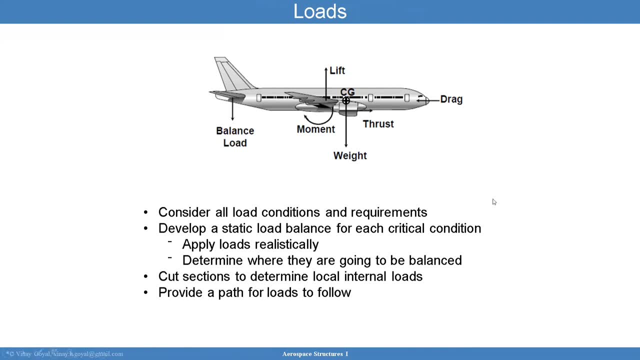 So you get bending, loading across the vehicle And again you can characterize that through a free body diagram, which you'll be doing as part of the homework. Here's an example of the loads And it's kind of nice. It's kind of nice to see everything together. 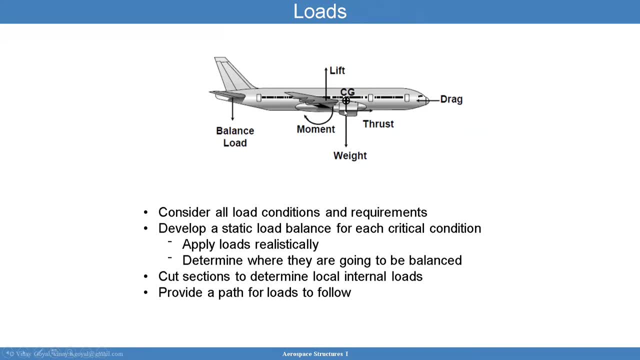 So here, side view is very nice. You have the drag, the weight, the thrust, the moment, the lift and the balance load. So that's the side view, Top view. you're going to have other loads as well. 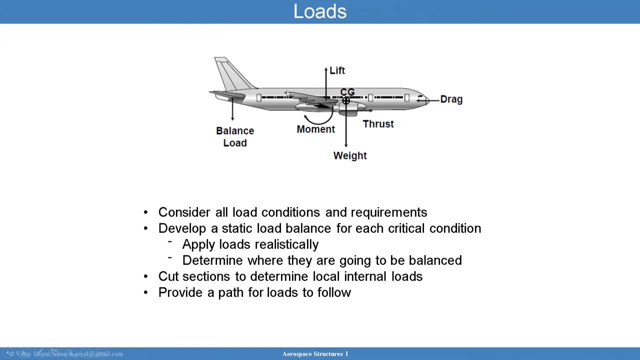 I'll show you later, But you can see very quickly here that if I know the lift, the drag, the thrust, the weight, the moment and balance load, I can just do section cut, Just treat this thing as a beam, cut it and then do a free body diagram. 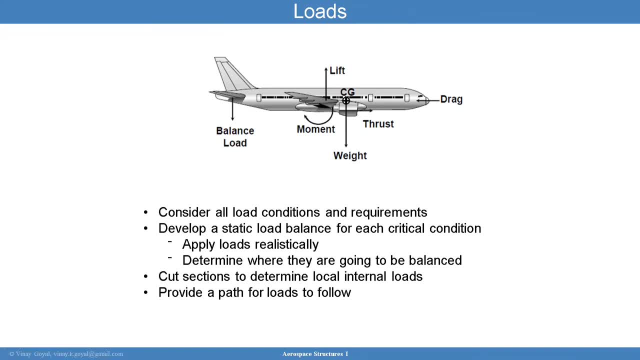 and get the section moment and the section shear. Using those two things as a functional location across the aircraft, you can now determine in size the cross-sections. Okay, That's it. That's a typical procedure for sizing an aircraft by hand. 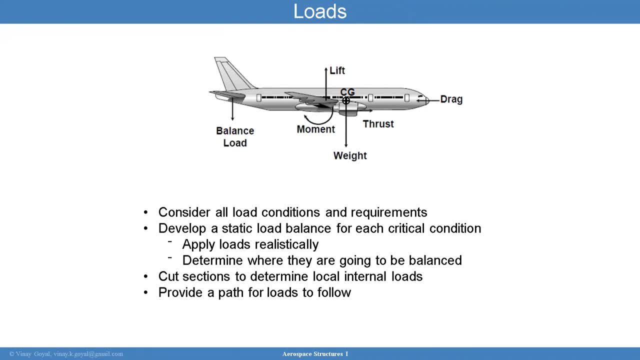 Then you'll go to find elements to confirm that what you're doing is accurate. Okay, So that's the general process here. So, yeah, the static load balance will help you understand what is going on in the aircraft, What is going on with the load paths. 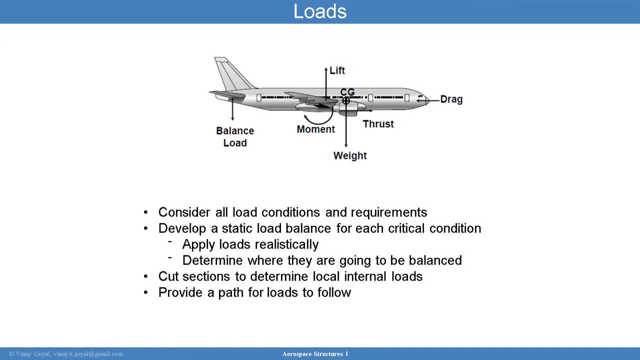 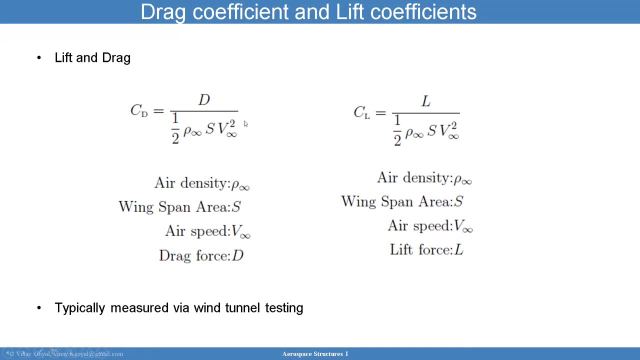 and how the bending moment and shear distributions are distributed- Very important stuff. Then here you have your lift and drag. This is the drag coefficient and this is the lift coefficient. These quantities can be determined from testing. And here you have D as a drag force. 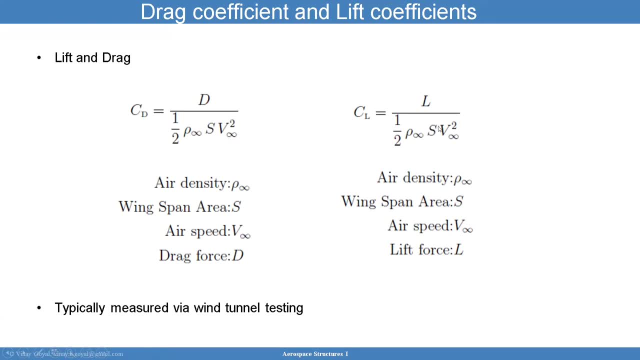 L is a lift force, Here S is a wingspan area, V, infinity. here is the error speed, And I'll go, I'll talk, I'll talk about that later. And then rho. infinity is the error density, And so this quantities correspond to. 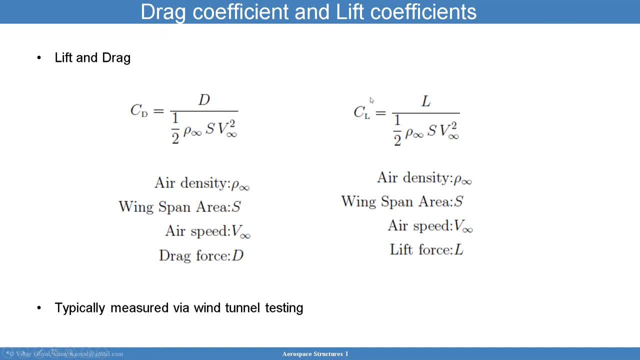 it's going to help you determine. So typically you calculate CD and CL from wind tunnel testing And given the density, given the speed of the aircraft and this wingspan area, then you can get D, the drag. And the same way here on the right-hand side you can get the lift. 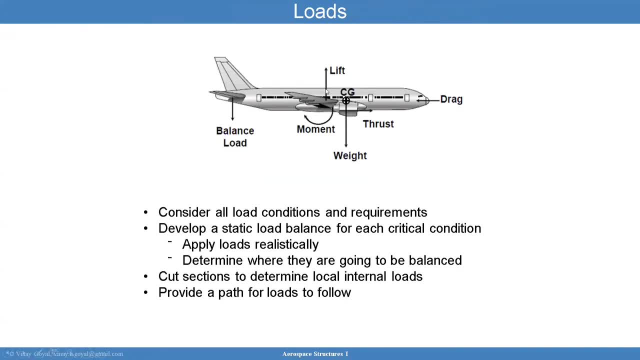 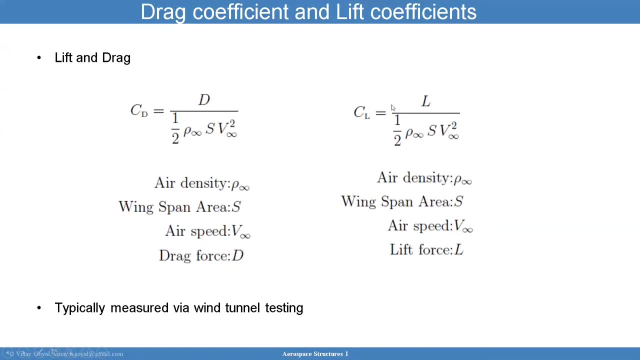 You can see, that is, you will get this lift and then this drag, And then the thrust is balanced in the drag, of course. So very clearly, these quantities can be fully found because you know at a given point what is the error: density. 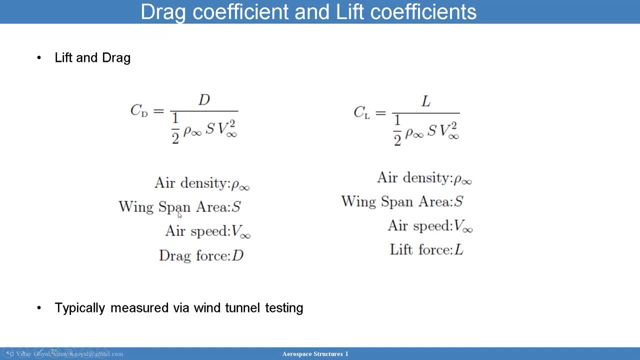 At a given point, you know the wingspan area doesn't change, Although it does change as you're landing. So you have to consider that loading condition as a separate one. And then you have the error speed, which is known as a function of time. 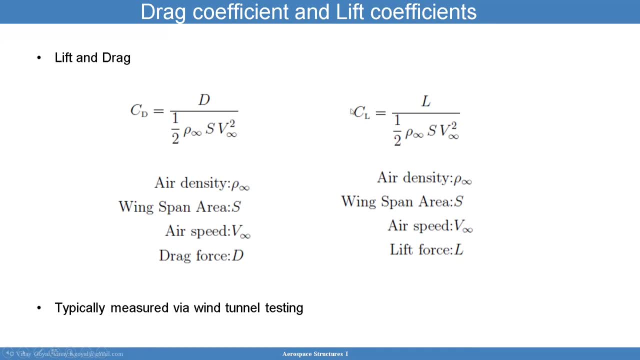 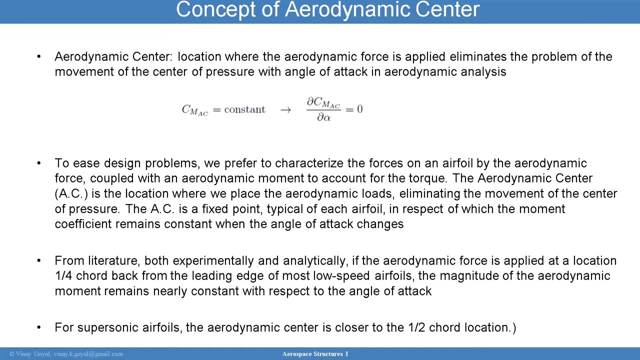 And then the drag coefficient, lift coefficient, which is typically calculated from wind tunnel testing. One of the important aspects that are discussed extensively in my book is the idea of the aerodynamic center. The aerodynamic center is the location where the aerodynamic forces is applied. 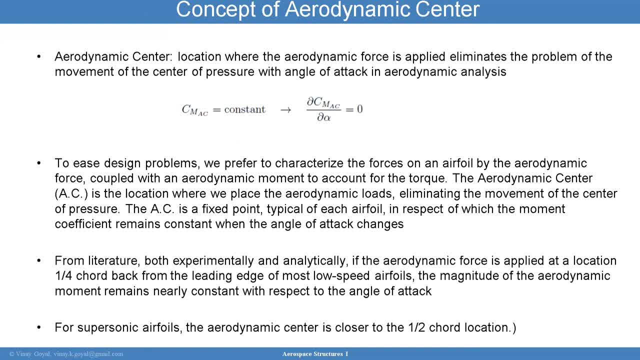 And that helps because it eliminates the problem of a moving center of pressure with angle of attack. in an aerodynamic analysis What happens is when you change the angle of attack, you move, you're going to have movement of that center of pressure on that wing. 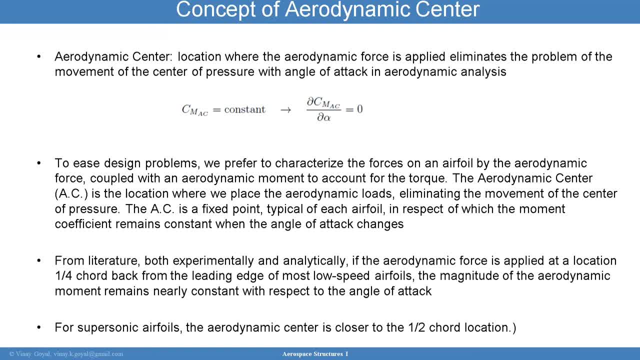 And so what the aerodynamic center is doing is trying to keep that at a particular location. So to ease the design problems, we typically prefer characterizing the forces on an airfoil by the aerodynamic force coupled with the aerodynamic moment to account for that torque. 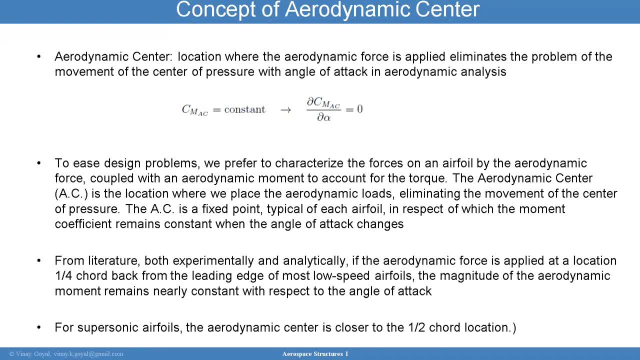 The aerodynamic center, then, is a location where we place those aerodynamic loads. That's where we're going to place them for structure analysis, And that way we eliminate the issue of the movement of the center of pressure. So, in other words, the aerodynamic center is a fixed point. 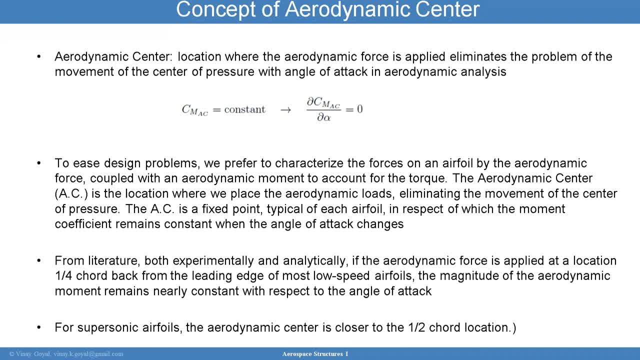 Typically for each airfoil, in respect of which the moment coefficient remains constant when the angle of attack changes. In other words, that aerodynamic center is a fixed point and is irrespective of what is going on with the angle of attack. From the literature. 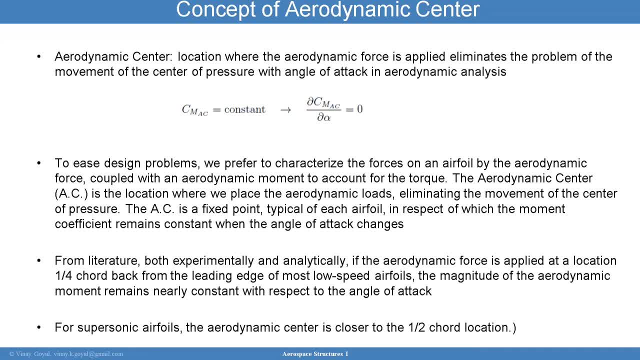 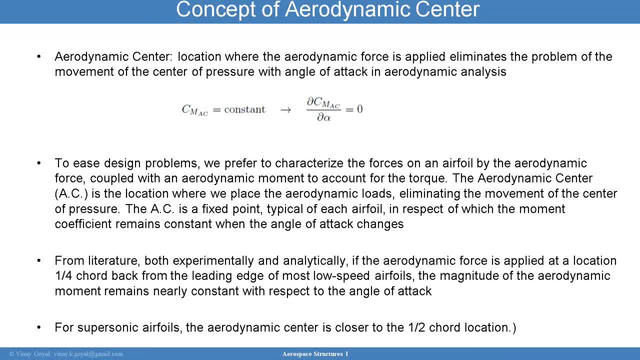 or back from the leading edge of most low-speed airfoils. The magnitude of the aerodynamic moment remains nearly constant with respect to the angle of attack, which is why that's so awesome to have that location defined For supersonic airfoils. you'll find that the aerodynamic center is more closer to a half. 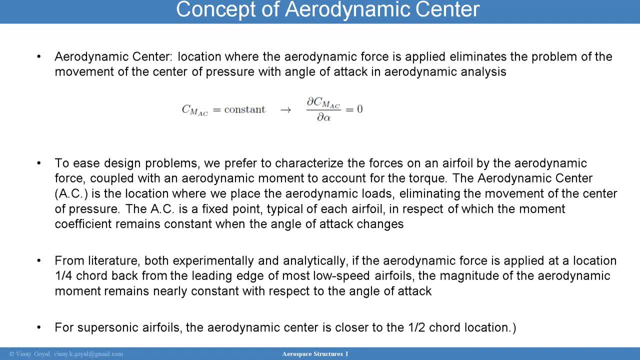 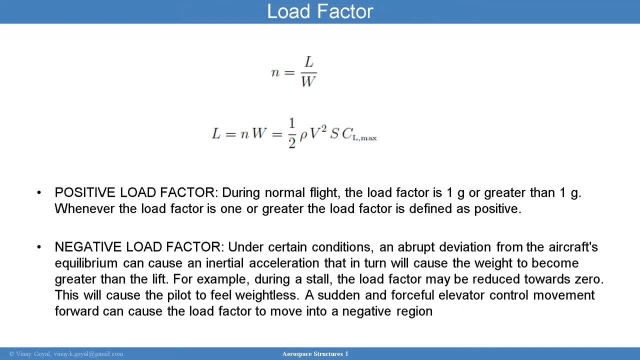 But for low-speed airfoils you're looking more at a quarter quarter back from the leading edge, And that's discussed extensively in the book and even shows you a way of calculating that. In fact that's a formula here trying to find how to calculate it. 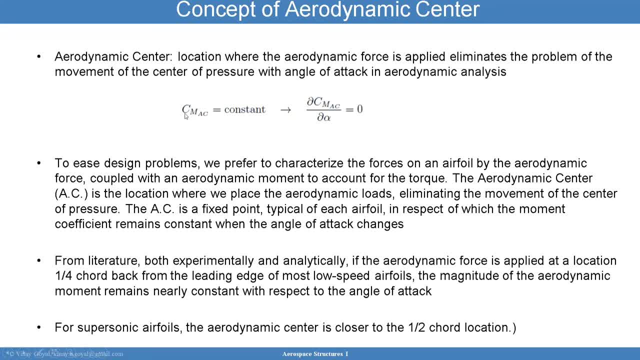 You want to keep that aerodynamic coefficient constant, the moment constant, And so to do that, you take this derivative set equal to zero and that tells you exactly where that needs to be. So you can actually can do it analytically. 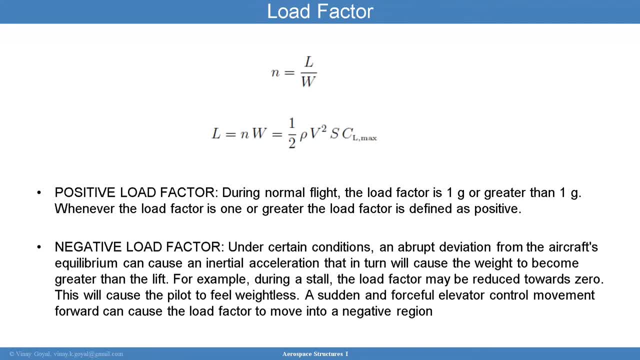 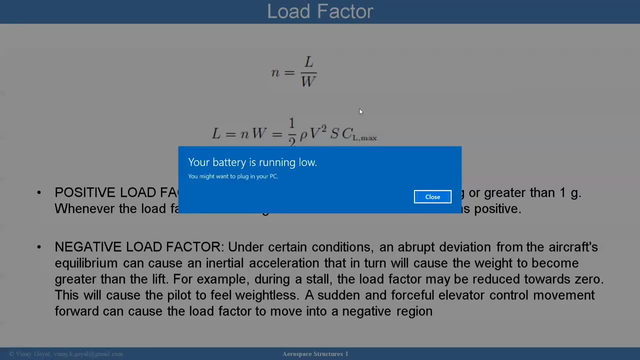 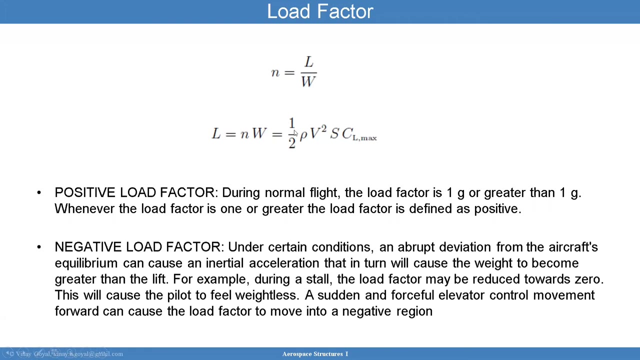 So one of the most important aspects of designing an aircraft is really: we're really here talking about the load factor. The load factor is lift divided by weight- Give me a minute. And so then we have. we have a load factor, And so then we have a load factor. 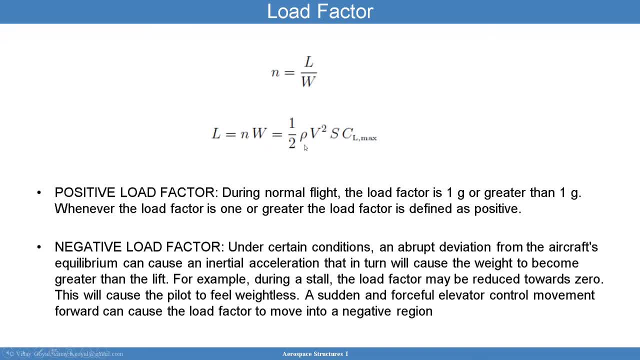 That the lift equals the load factor times the weight, which is one-half rho V squared S, And then you have the lift coefficient, which is the maximum value you could have, And so that will give you the maximum lift you can ever have. 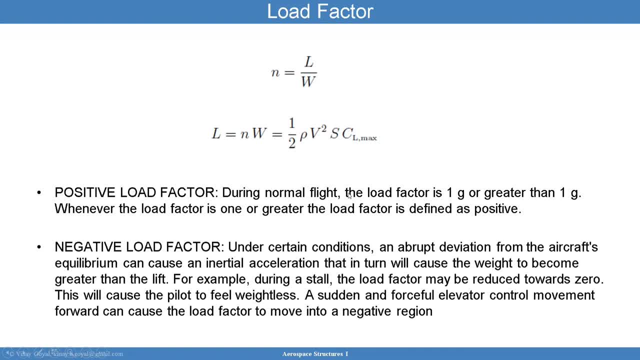 The positive load factor. during normal flight, the load factor is 1G or greater than 1G. Whenever the load factor is one or greater, the load factor is defined as positive. A negative load factor now corresponds that under certain conditions. 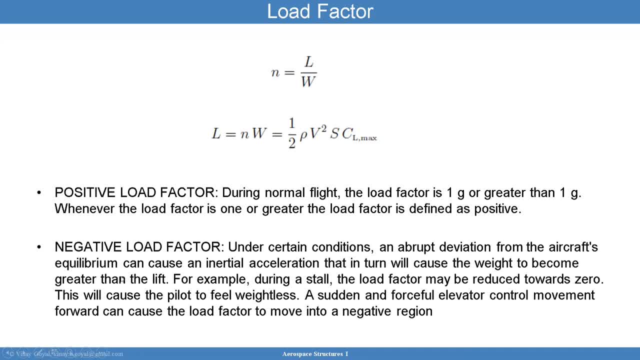 an abrupt deviation from aircraft's equilibrium can cause an inertial acceleration that in turn will cause a weight to become greater than lift. So you can have a situation where weight is greater than lift, And when that happens, then that will happen during a stall. 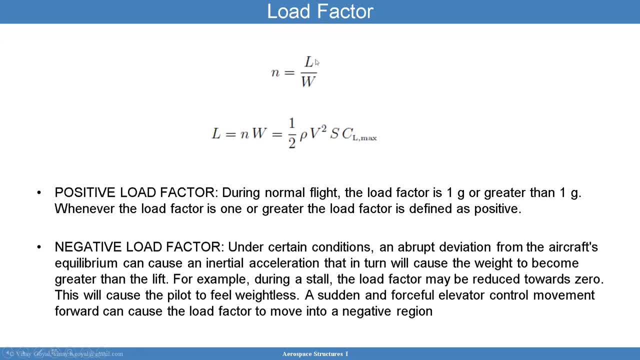 The load factor will reduce to zero, because you get basically zero lift. At that point the pilot, everybody will feel weightless, And so that's why in that case you have a negative load factor. A sudden and forceful elevator control movement can also cause a load factor to move into that negative region. 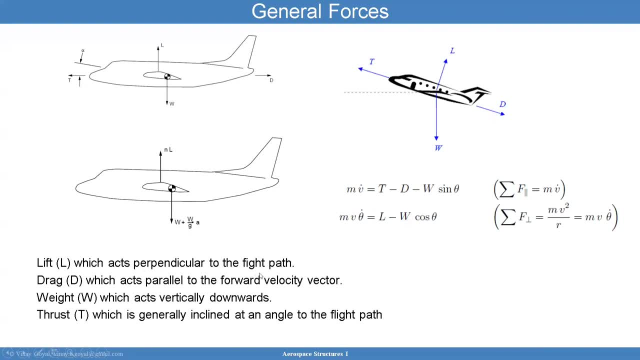 L acts perpendicular to a flight path, And you can see here the vehicle here moving to the left, And so that's that lift is perpendicular to a flight path. D acts parallel to the forward velocity vector and it tends to be parallel to the to the flight path. 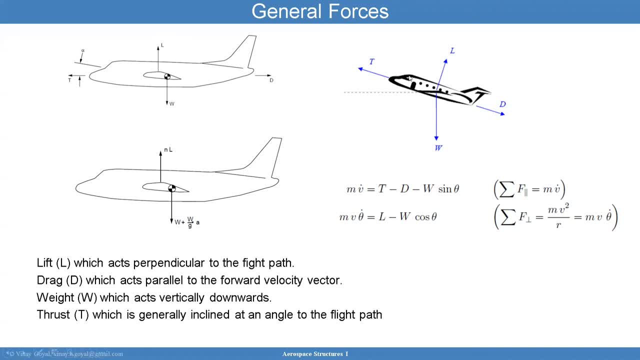 Weight acts vertically down. So you can see here an example: The aircraft is, is inclined, And so W always acts downward And T is generally inclined at an angle to the flight path. So you can then write the equations for this particular situation. 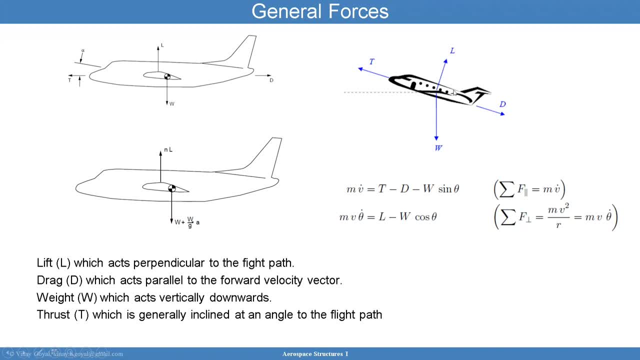 And you can calculate: summation of forces equals ma, which is m times the velocity. dot Equals the thrust minus the drag minus W, sine theta, And so that will give you the velocity. They'll give you the equation of motion along the thrust vector here: 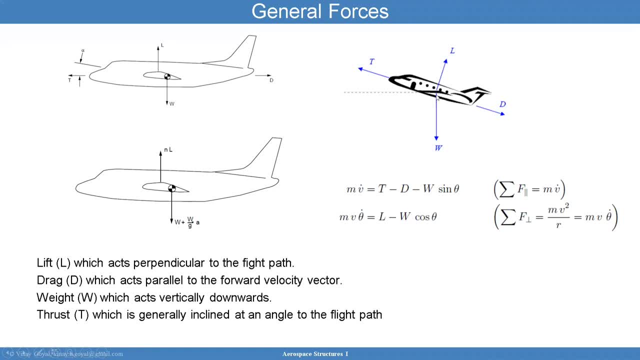 So that's T minus D, And then this W can be decomposed So it goes along the D direction, the drag direction, and that's W sine theta. Then you can write also the, the equation uh, perpendicular to the flight path. 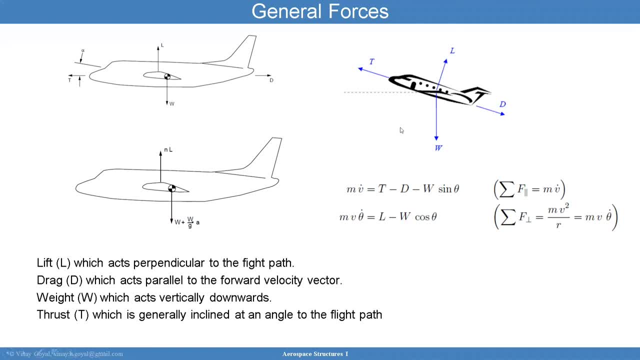 And you can do that very quickly And you get L minus W cosine theta. That's in that direction And they have envy times theta dot or the rotation of that aircraft. So V times theta dot gives you an acceleration as well, And you can see here that I get envy squared divided by R. 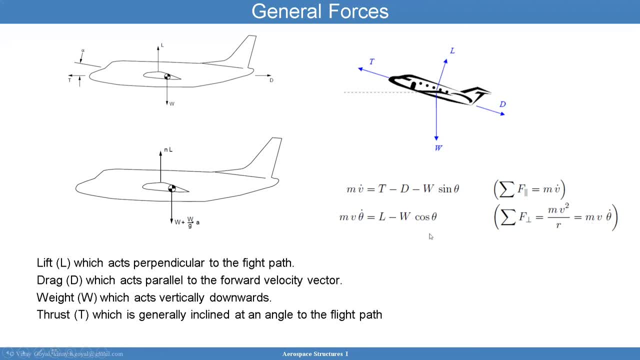 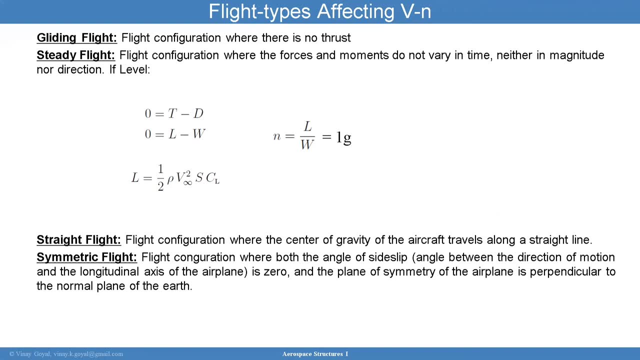 which is the same thing as envy. So that's the equation. So this is the equation I get. uh, for this particular situation. If I have a gliding path, the flight configuration there means that there's no thrust. So in this equation, 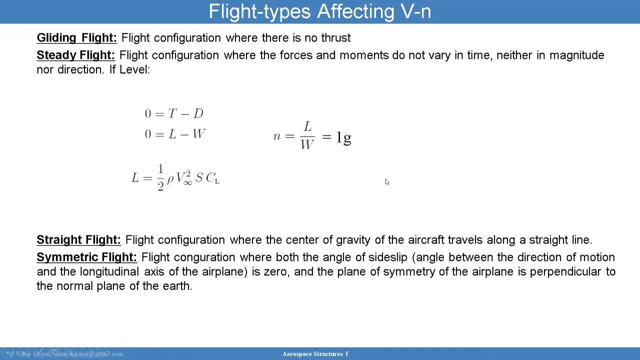 thrust is zero: Steady. steady flight means that the flight configuration where the forces and moments do not vary in time, neither in magnitude nor direction. So if it's level flight and a steady flight, then T minus D is zero and L minus W is zero. 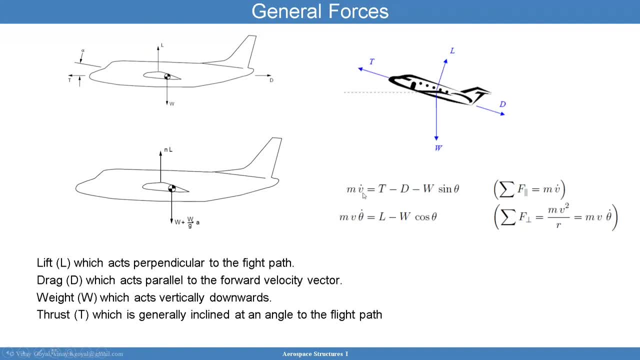 In this case, you can see that that works out because the left hand side is zero, So therefore, and then theta is also zero, So this is one, this is zero, And so therefore, T, the thrust equals the drag, the lift equals the weight. 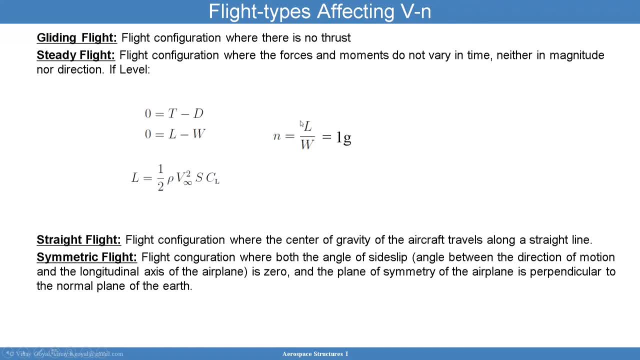 And if the lift equals the weight, then if you're a passenger in an aircraft, you feel a load factor of one because you feel your own weight, one G And again L is one half, rho V, infinity squared, or the airspeed. 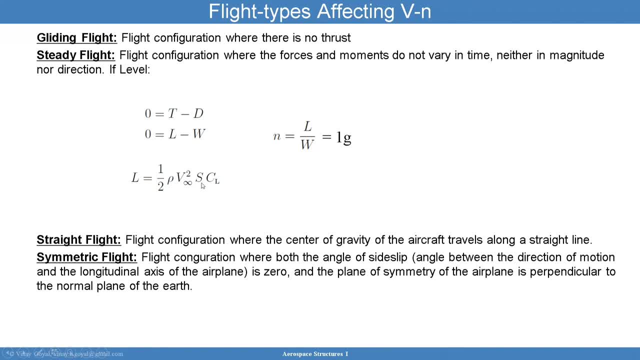 And then S is a span area of the wing And CL is a coefficient of lift that can be found through wind tunnel testing and depends on the angle of attack. Here the angle of attack is zero. I'll show you later how CL varies as a function of alpha. 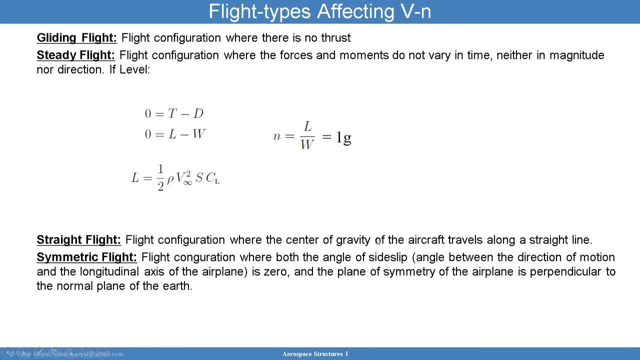 Straight flight, the flight configuration where the center of gravity of the aircraft travels along the straight line. And then you also have the idea of the symmetric flight Flight configuration where both the angle of slight slip, which is the angle between the direction of motion, and longitudinal axis of the airplane. 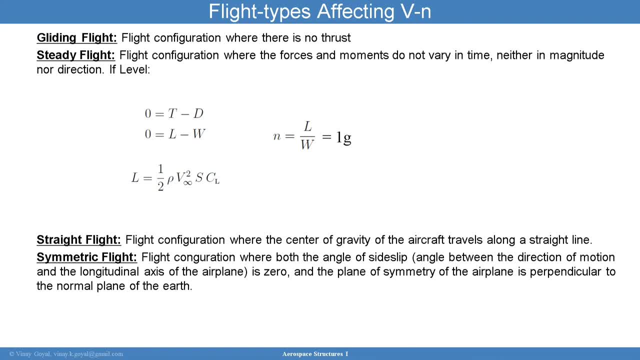 is zero, And the plane of symmetry of the airplane is perpendicular to the plane of the earth. So that's what symmetric flight means. And then you have again straight flight, steady flight and gliding flight- Very important concepts to keep in mind as we move forward here. 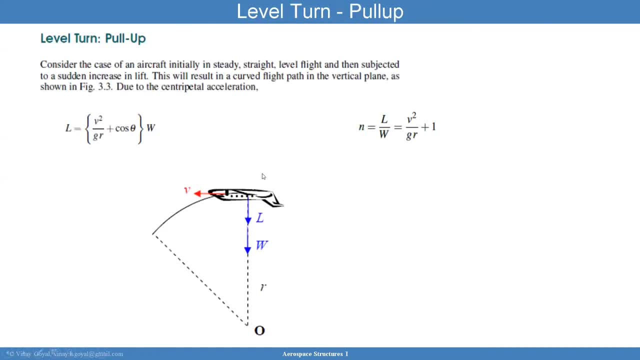 So let's look at the equations for level, turn up, pull up. So here you can see that the lift and the weight are pointed towards O and the velocity here is B. And if you were to calculate the centripetal acceleration, you will find that the lift is related to the weight through this equation. 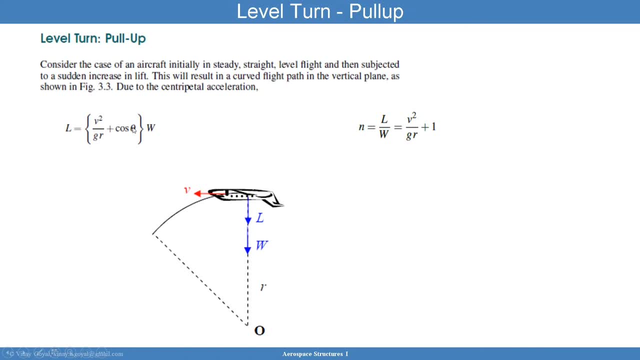 B squared divided by GR plus cosine theta, And you can then also calculate N, which will be L over W. And then you can see here that the greater the velocity, the greater the load factor, or the smaller the radius, they'll also increase the load factor. 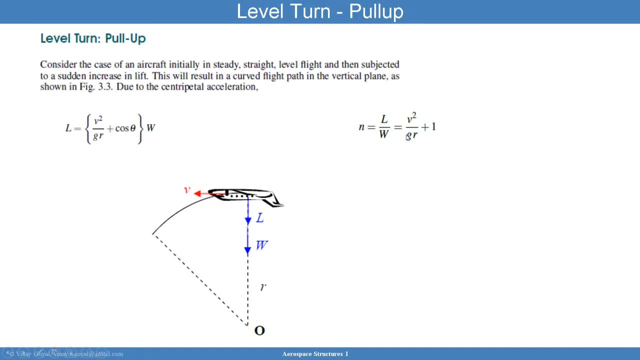 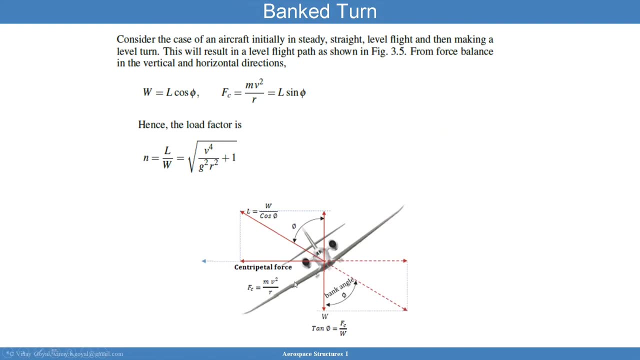 G is a constant, the acceleration constant here. Then you can consider a banked turn. So in this case a banked turn looks like this: You can see that the aircraft is rolling. That's your banked alpha phi. The weight always points downwards. 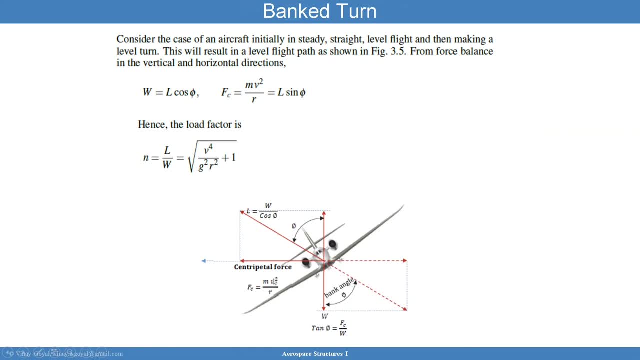 So that's easy. And then you're also going to have a centripetal force: MV squared divided by R, And then you have the lift again. is W divided by cosine P, And so you can calculate from here the load factor for this situation. 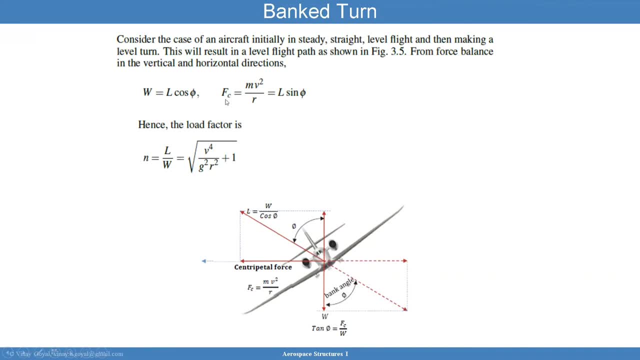 W equals L cosine phi. And then FC is a centripetal acceleration or force. is MV squared divided by R, And that's equal to L sine phi. And you can see here that now I can then calculate L over W. And when I do that calculation? 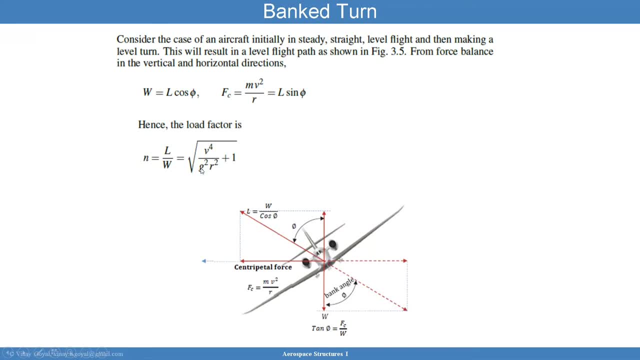 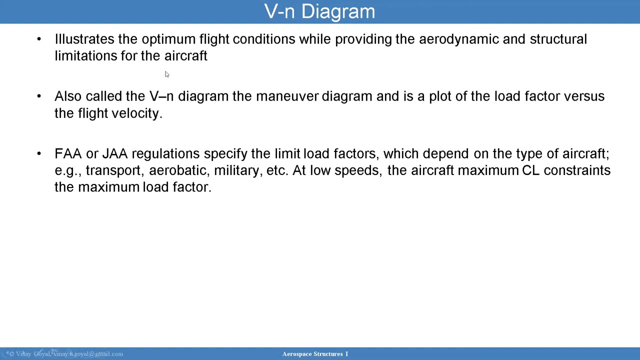 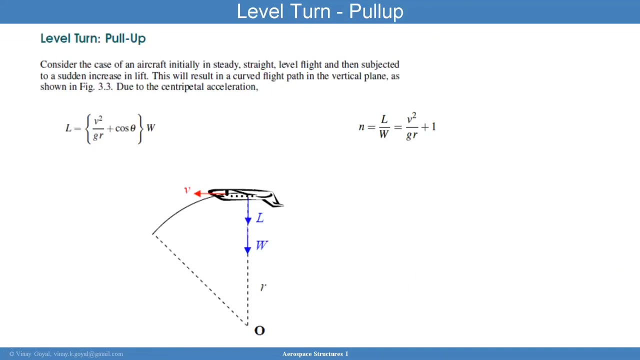 I get the square root of V to the fourth, divided by G squared times R squared. all that plus one Square root of that, that gives you a load factor for this problem. So the V-N diagram And one more thing. So this load factor will become important for the next discussion. 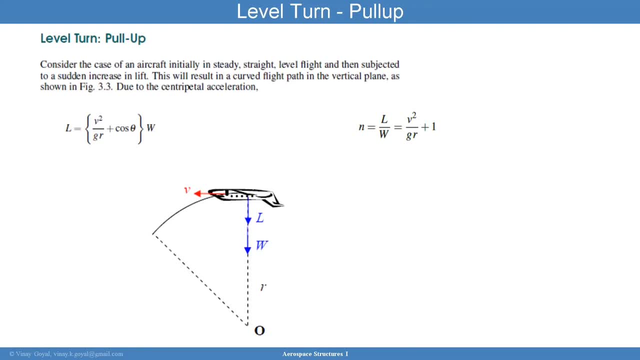 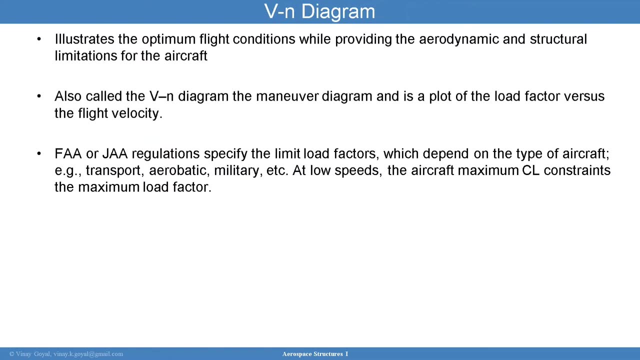 And just for pull-up. you can also calculate for pull-down And that's in the book. You can look it up there. But the load factor will become important coming up. This illustrates the optimal. the V-N diagram illustrates the optimal flight conditions while providing the 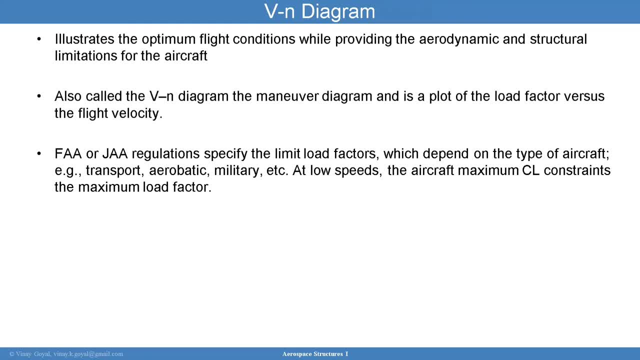 aerodynamic and structural limitations for the aircraft. It's also called the V-N diagram, the maneuver diagram, And it's a plot of the load factor versus the flight velocity. So that's what the V-N diagram is. It allows you to come up with a flat envelope. 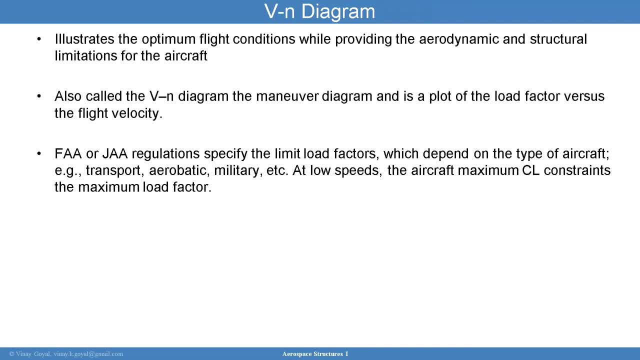 And that flat envelope is important in driving the design. It's actually one of the most important plots in the design process. The FAA or JAA regulations specify the limit load factors which depend on the type of aircraft. It could be transport, aerobatic. 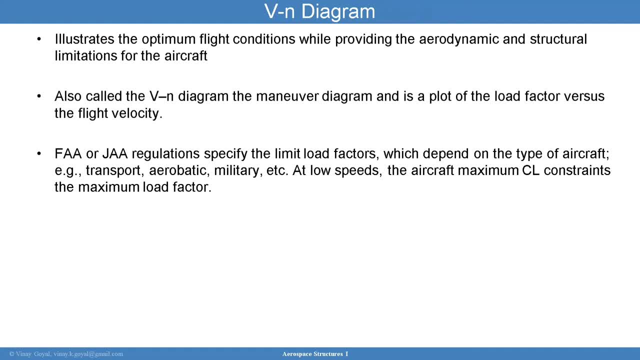 military And at load speeds. the aircraft maximum lift coefficient constrains the maximum load factor. We'll be discussing that coming up. But again the V-N diagram really is the envelope And that drives a lot of the design that goes. that needs to be done. 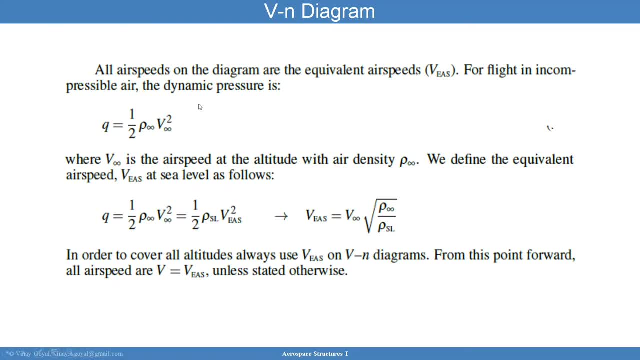 So here I want to point out some important aspects. So here you can see this: the dynamic, the dynamic pressure. The dynamic pressure is one half the air density times the air speed. But all air speeds on the diagram are equivalent air speeds. 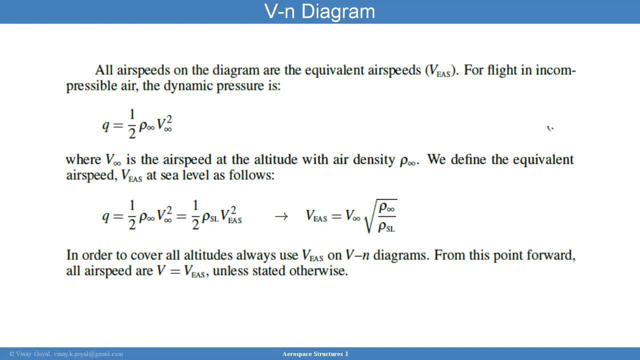 And so when you create a V-N diagram they're all equivalent air speeds. So I had to find a way of transforming that to that For flight in incompressible air. the dynamic pressure is: Q equals one half the air density of air. 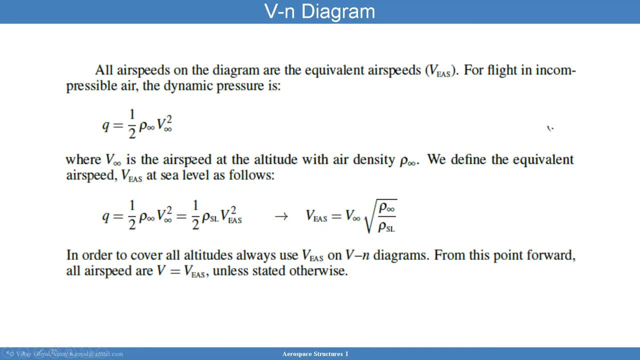 the air speed at the altitude of concern squared. So we have to define an air speed so that everything can be equivalent, And that's typically done at sea level. So the way you're going to do that, you're going to calculate an equivalent air speed. 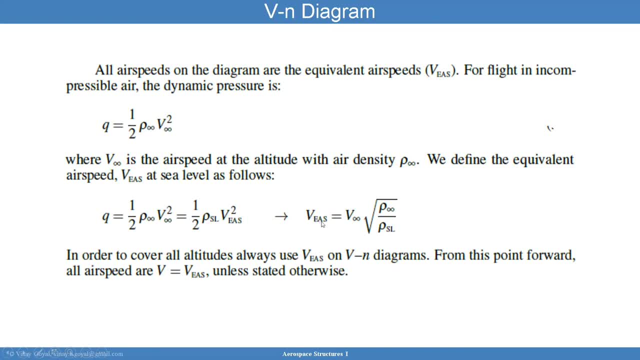 To accomplish that and to do that you have equivalent air speed equals the air speed at that altitude of the density at that altitude divided by the density at sea level. So you're really referencing back to sea level And that's how the velocity is calculated. 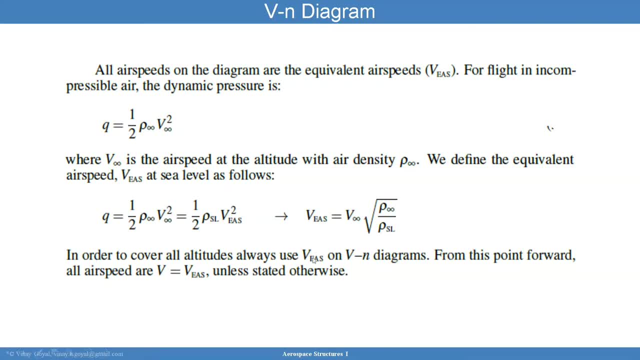 In order to cover all altitudes, we always want to use the velocity at sea level on the V-N diagrams And we call that. the equivalent air speed is what I should say From this point forward: all air speeds. now I won't use the V-E-A-S. 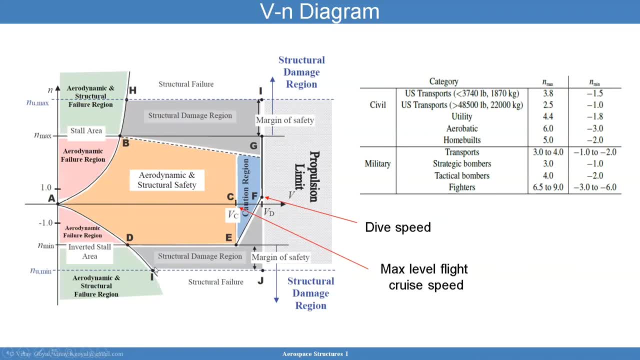 We're going to just call it V, so it's much easier to deal with that. Now, this is the V-N diagram, And the V-N diagram is quite busy here. Let's focus here on the right first, And you can see for civil and commercial aircraft. 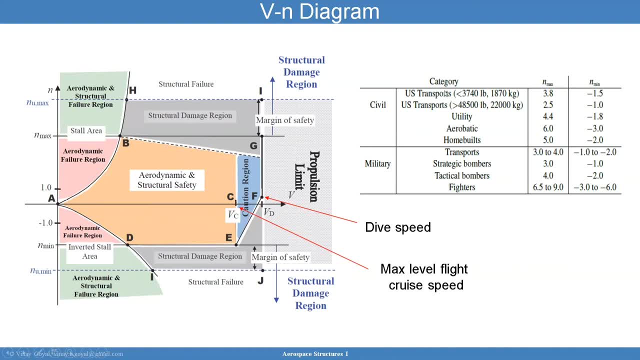 you have category aircraft. You have US transports less than 3740 pounds. You have US transports greater than 48,500 pounds. You have utility aerobatic, home built transports. strategic bombers, tactile bombers. 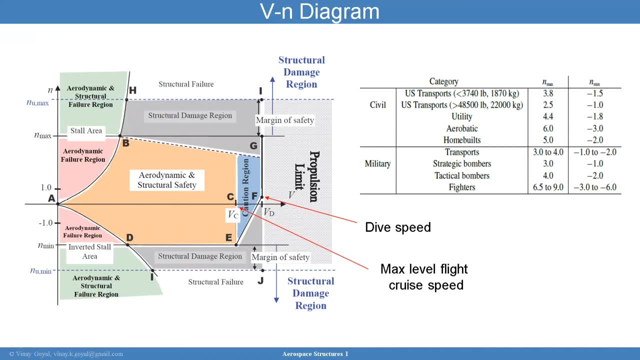 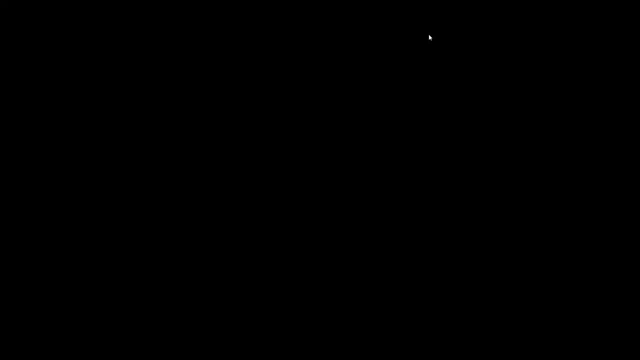 and fighters. And then in the next column, what you have there is the maximum load factor, And that's the maximum load factor. It's really the maximum load factor that's been specified. And then you have the minimum load factor. So the load factor here. 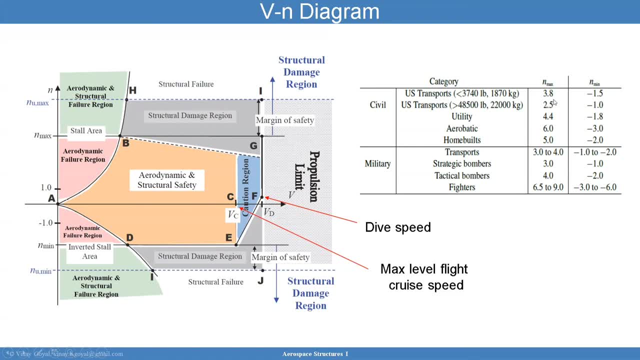 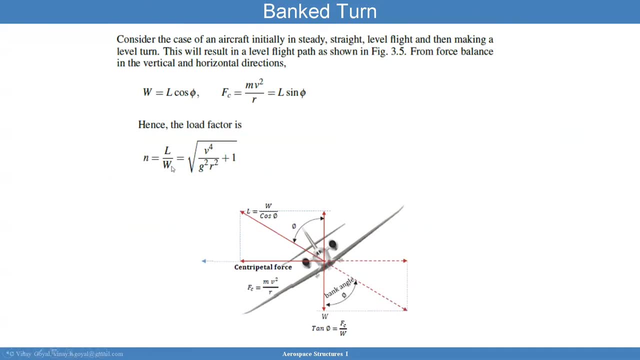 you can see that for US transport is 3.8.. What does that mean? Let's go back to the definition of load factor. So here lift divided by weight, the maximum value it can have is 3.8.. 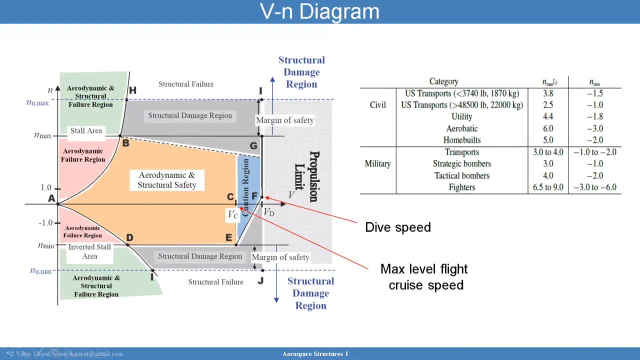 That's what this is telling us that N max is. And then we also have the US transport above 48,500 pounds is 2.5 N max, But the negative load factor is 1.0.. So these you can see here. 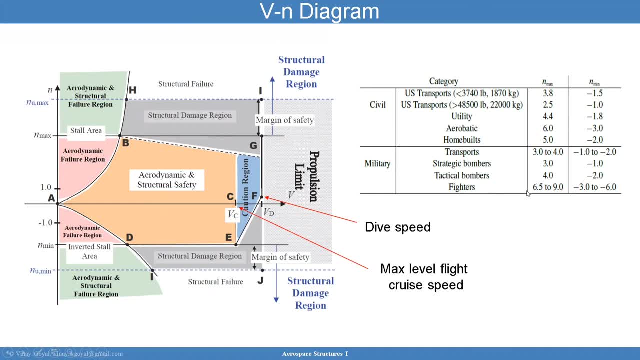 the fighter jets can achieve a higher load factor, And so they're designed more aggressively to meet that. So when I look, this is very important information. This drives your design. So I go here towards the left and I study what is going on. 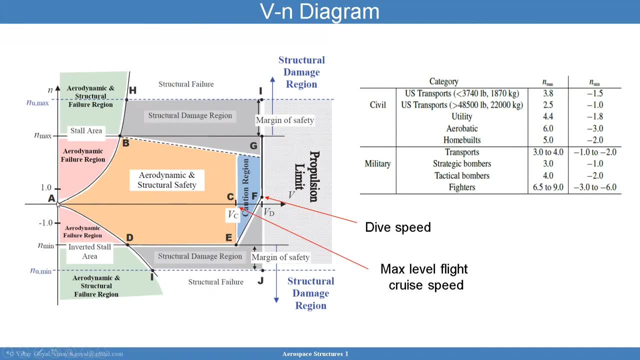 Let's take it step by step. From you can see here there's a curve here right And where you see this color, here this peach color AB, the region AB and then a line drawn downward, C ED. 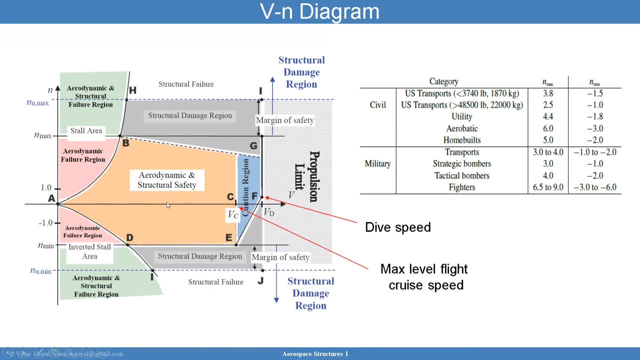 all this area here, I call it the aerodynamic structural safety. I'm safe in this space, Okay, And then the next thing I want to point out: let's go all the way to the right. So when I go beyond this straight line downwards, 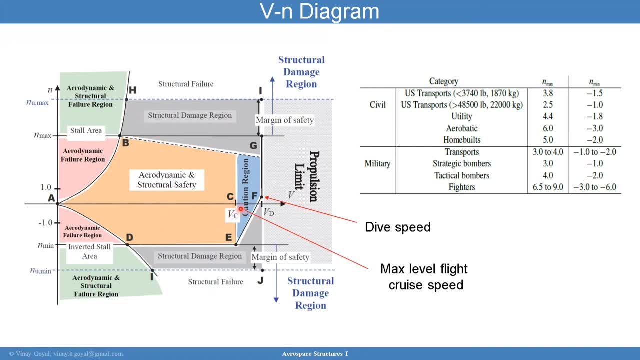 and let me use a laser pointer here. When I go past this straight line to the right, I start to enter the calcium region, And what I mean there is I'm going to come into something called the dive speed. And this dive speed. 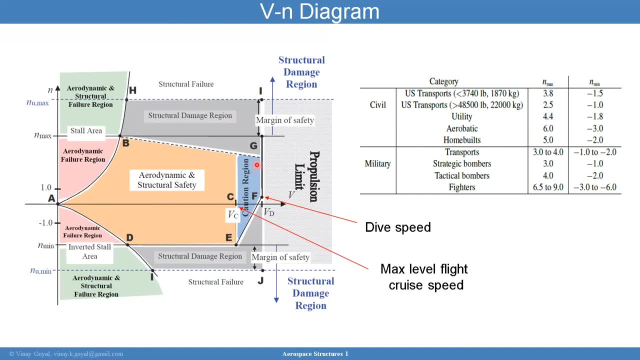 you could have a flutter, a condition called flutter That velocity. we want to stay away from that. There's a particular test that's done to really show that we're okay. there. Past this point, we are at the proportion limit, So clearly we're going to be not here. 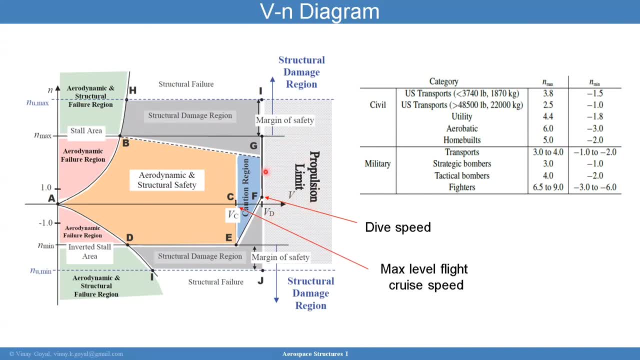 It will be very hard to get here because of the proportion limit itself. So you're really constrained from VB and less And we want to really keep it at the maximum level flight cruise speed, And if you went above that, that's a calcium region. 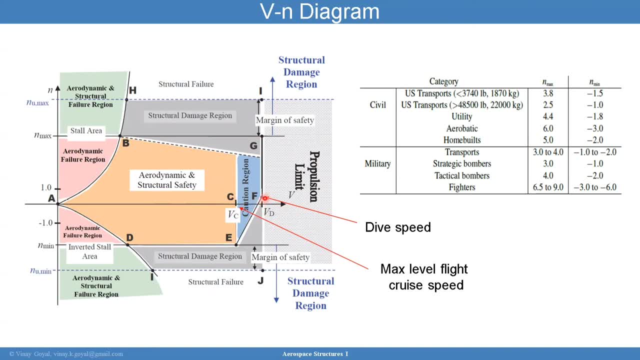 And you could start entering flutter when you hit the dive speed. So that's where we are. So now let's look at what is going on here. This curve here, curve here, ABH. This curve here. if I'm less than this curve. 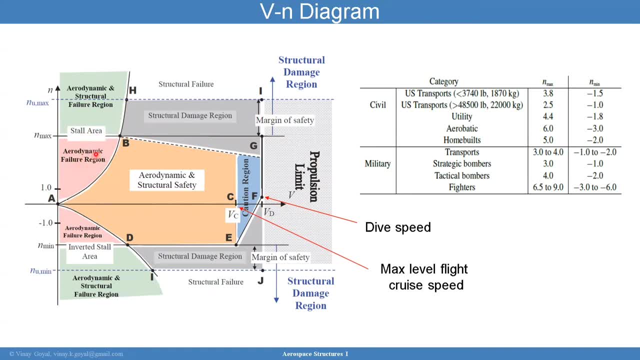 and I'm in this pink region. I call that the aerodynamic aerodynamic failure region, So I could be stalling right. So that's what that means. This pink area here is called aerodynamic failure region And I will have inverted stall in this region. 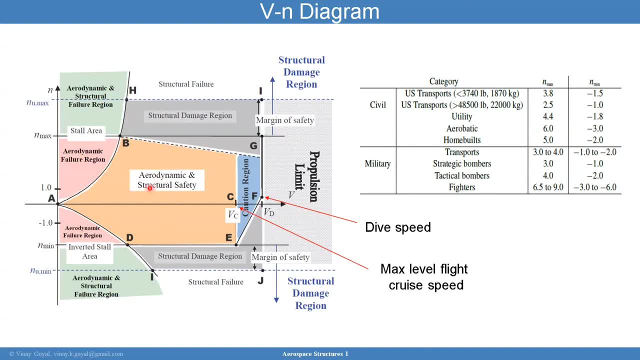 So I want to stay away from here and here. I want to be in this bucket here, And then I have the Nmax, Nmax, points B to this point here, protecting us against structural damage. That's what that is. And then here: 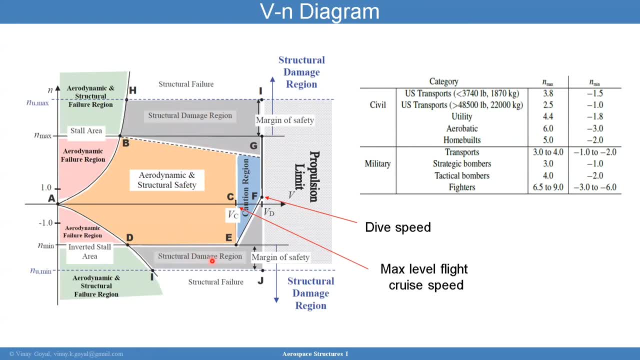 I also want to protect against structural damage in the inverted configuration with negative load factors. So, again, this is where I want to be And this is where I want to be Okay, And I want to keep within this zone here. That's what we want to do. 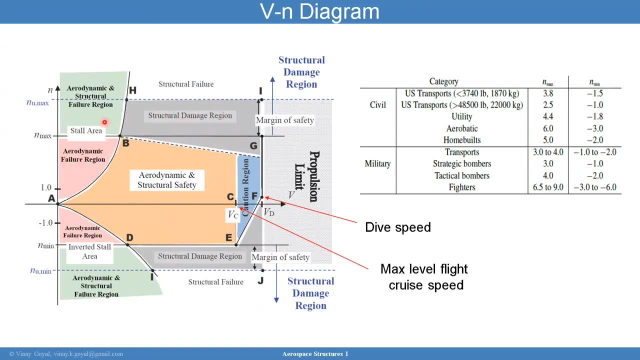 We want to keep away from structural failure in the gray, Aerodynamic failure in this region, And then we don't want to enter into the calcium region. We want to stay in this area And notice how- and I apologize if it was not clear- 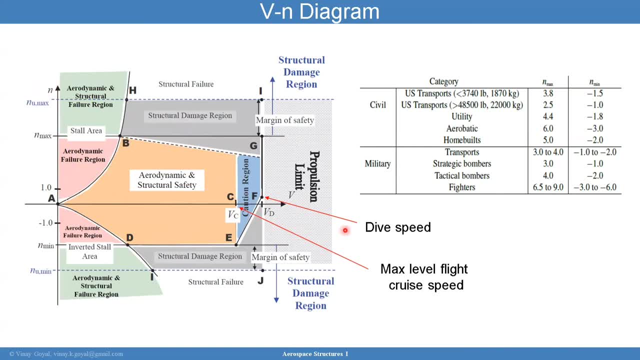 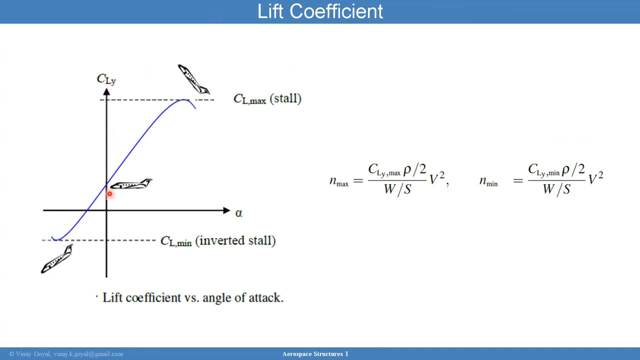 The y-axis is a load factor And the x-axis here is the velocity of the aircraft. Again, the V-N diagram drives a lot of the analysis that needs to be done. Here you can see what the lift coefficient is. The lift coefficient is a y-axis. 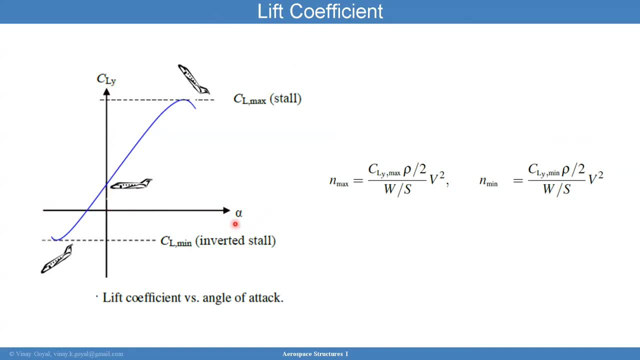 In the x-axis, we have the angle of attack And you can see here: zero angle of attack. you have a particular lift coefficient And, again, what you want to do is you want to use this information. You can see here: 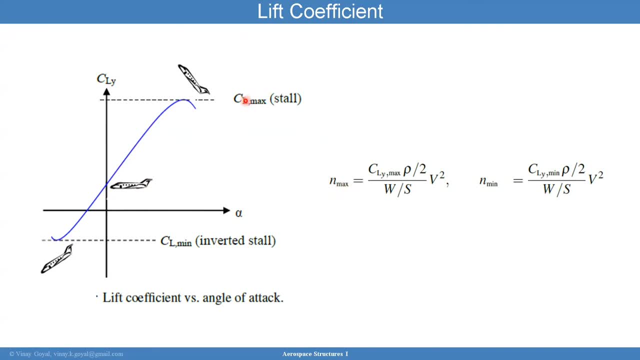 how Nmax is equal to the maximum lift coefficient I can have. Right, What is the highest load factor I can have? The highest load factor I can have is one that gives me the maximum lift coefficient, The maximum lift coefficient. So that's that point here. 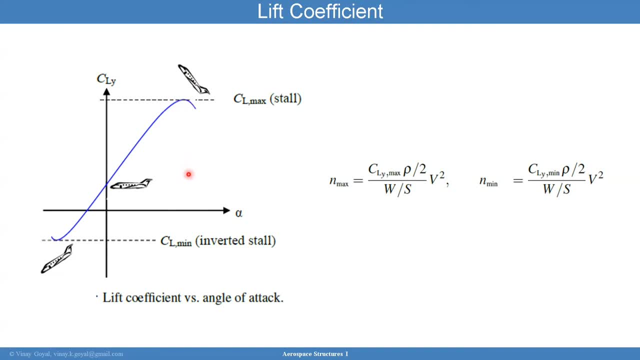 Okay, And that means I'll be at a higher angle of attack, So I'll be pushing the load factor quite strongly there. And then times the roll divided by two, Doubly divided by S, And this is the velocity airspeed. 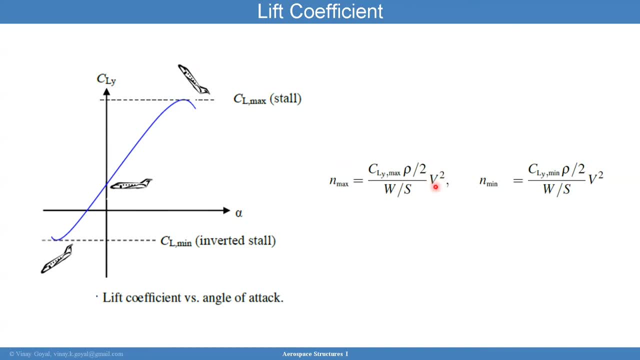 equivalent airspeed, as we discussed before, which has been done by referencing to the sea level density, And then, very similarly, I can calculate the minimum load factor, And that minimum load factor is driven by here. You can see, here I have an inverted stall. 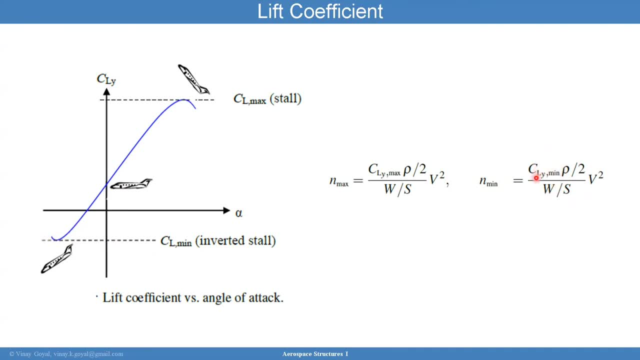 And so that coefficient of lift can also be calculated. And so with that information you can determine Nmax and Nmin. And you can plot that very simply because you know the weight of the aircraft, you know the wingspan area, you know the density. 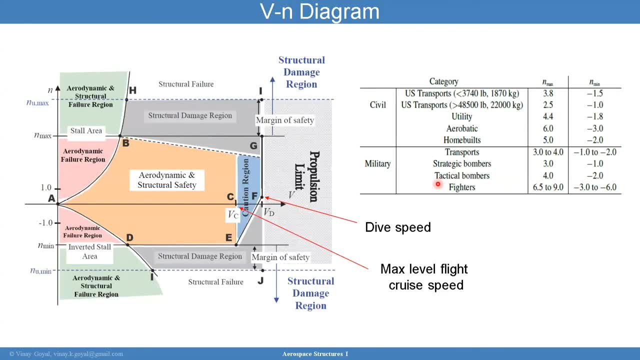 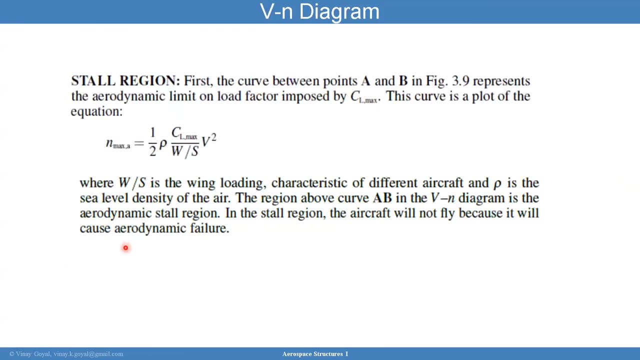 and then you know V, the airspeed And you can see here I can now calculate Nmax and I can calculate Nmin for point B and for point D. So let's look at the stall region first, very carefully First. 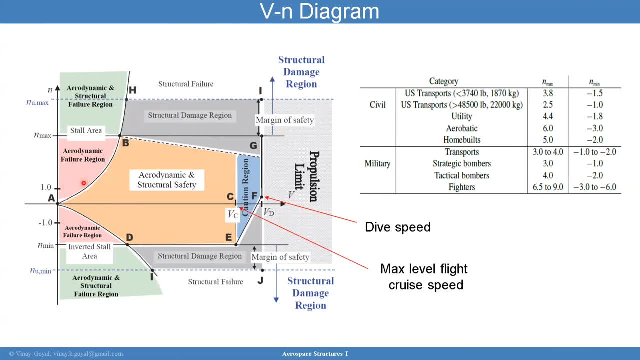 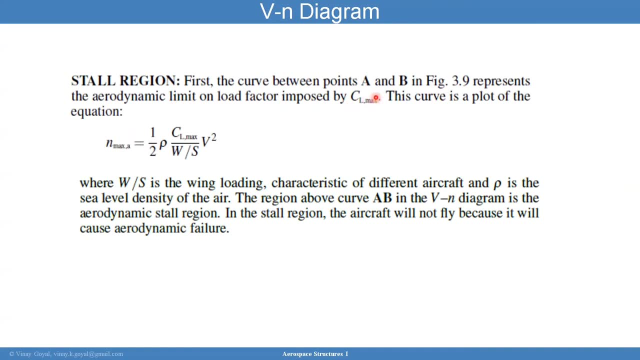 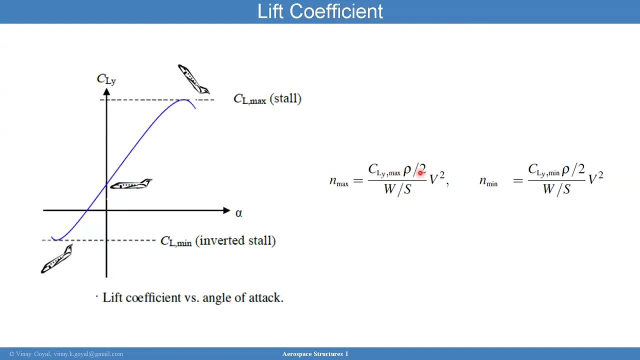 the curve between points A and B. so the points between points A and B here represents the aerodynamic limit on load factor imposed by Clmax. So Clmax here was calculated to be this. I showed it in this slide And I put a comma A to indicate aerodynamic failure. 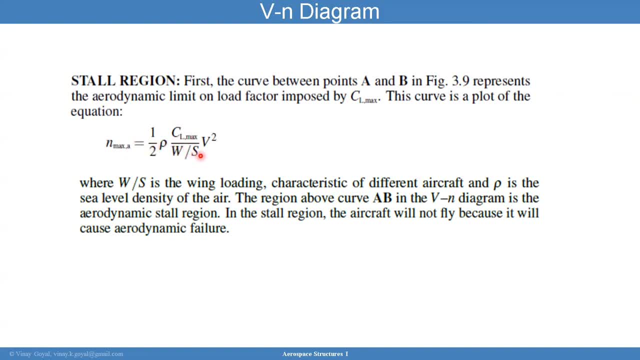 So one half rho Clmax W over S V squared Where Ws is the wing loading. it's a characteristic of different aircraft So this will be always different for different aircraft. Rho, here is the sea level density of air, Remember. 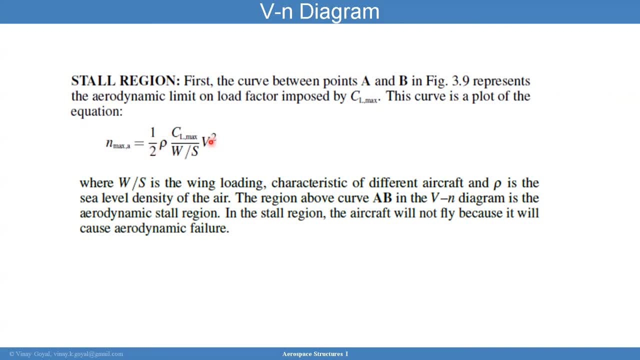 we tried to reference everything back to sea level And V is the equivalent airspeed. The region above curve AB in the V-end diagram is the aerodynamic stall region. In this stall region the aircraft will not fly because it will cause aerodynamic failure. 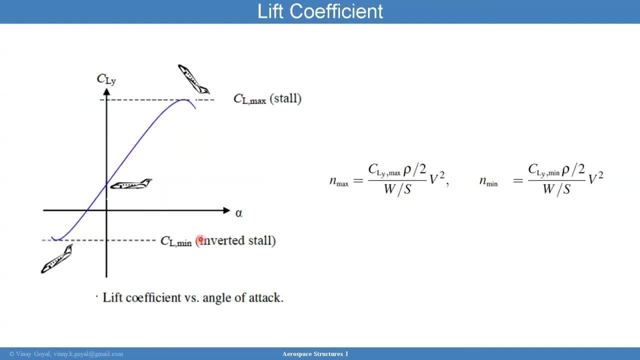 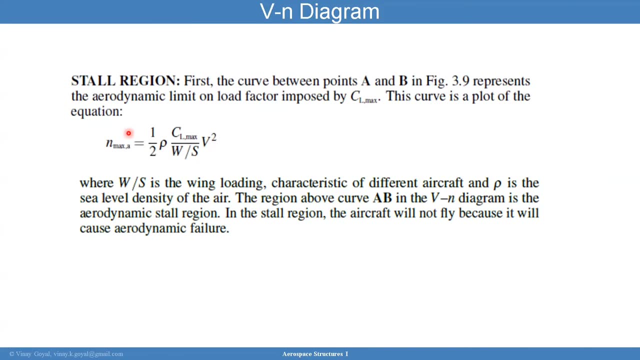 I mean, if you try, then you're going to fail aerodynamically. So that's what that curve, that's how you construct that curve. right here In the book we go through several examples on how to construct this very carefully. 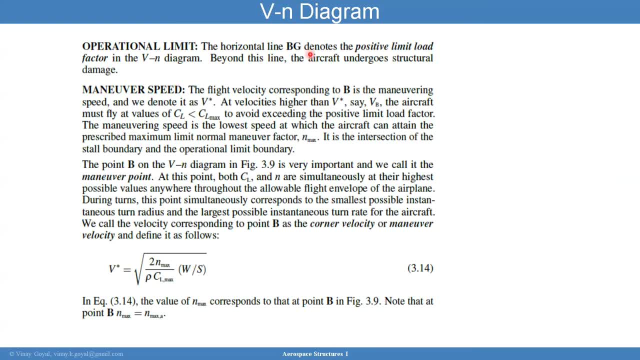 The operational limit, which is a horizontal line B. BG denotes the positive limit load factor in the V-end diagram. Beyond this line, the aircraft undergoes structural damage. Let me look at that with you carefully. So that's line BG here. 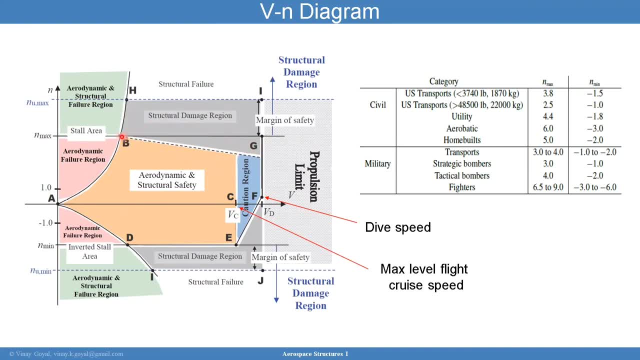 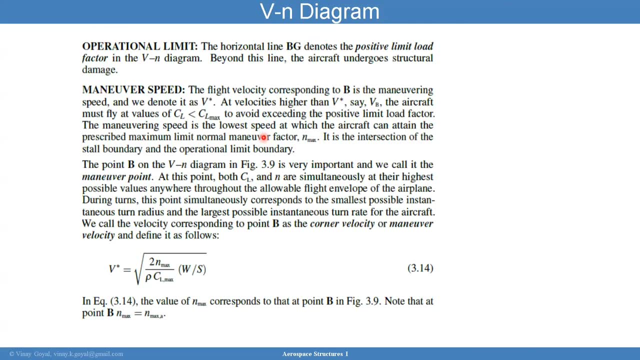 Okay, that line BG and I should draw from here to here- I apologize, from here to here. If I'm above that line, then that above that load factor the aircraft will undergo structural damage. Maneuver speed: the flight velocity corresponding to point B is the maneuver speed. 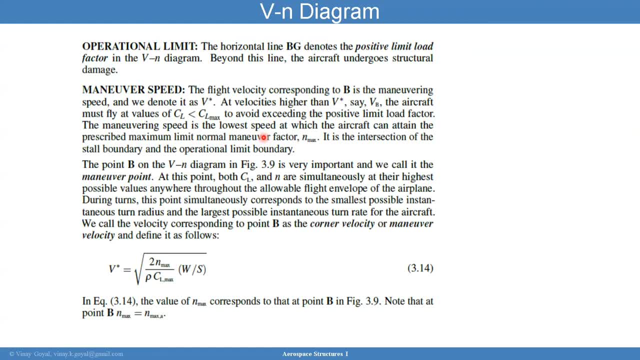 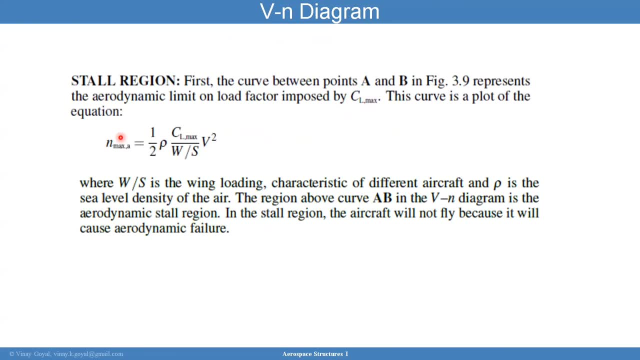 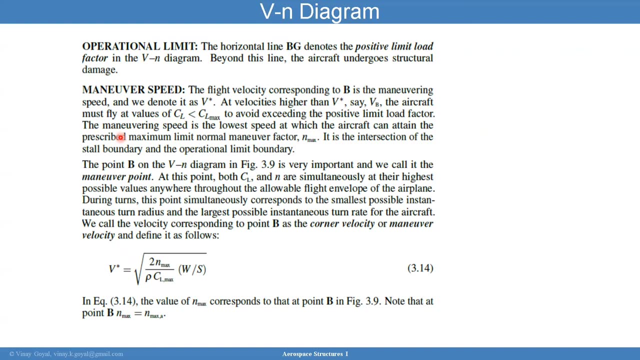 And I'm going to denote that as V-star. So let me look at the flight velocity here. That's the velocity V-star we're talking about at that point in time, And as velocity is higher than V-star, say VB, the aircraft must fly at values that are lower than the maximum lift coefficient. 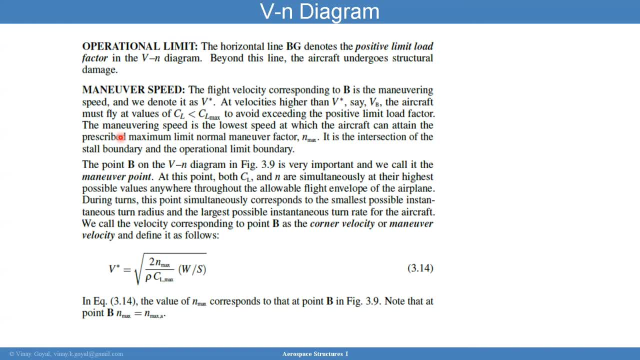 to avoid exceeding the positive limit load factor. The maneuvering speed is the lowest speed at which the aircraft can attain the prescribed maximum limit, normal maneuver factor and max. And it is the intersection of the stall boundary and the operational limit boundary. So I showed you that. 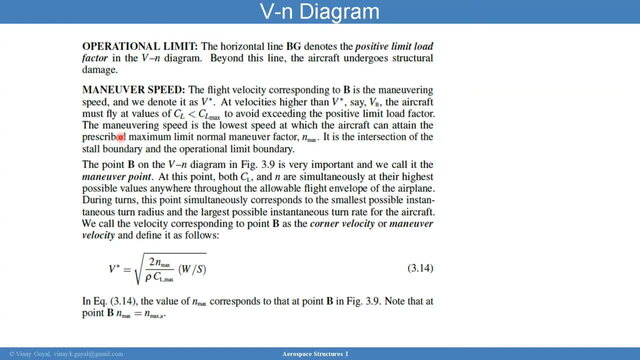 The point B on the V-end diagram is very important and we call it the maneuver point, And I said that several times At this point. both the coefficient lift and the load factor, both of these are simultaneously at the highest possible values anywhere throughout the flight envelope of the aircraft. 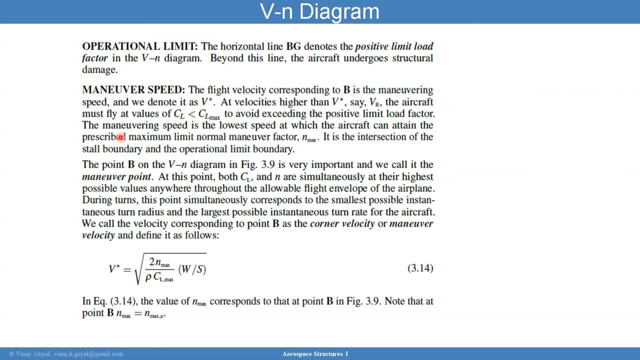 During turns, these points simultaneously correspond to the smallest possible instantaneous turn radius. So if I'm turning and that's going to correspond to the smallest possible turn radius and the largest possible turn rate for the aircraft, So we call the velocity corresponding to point B. 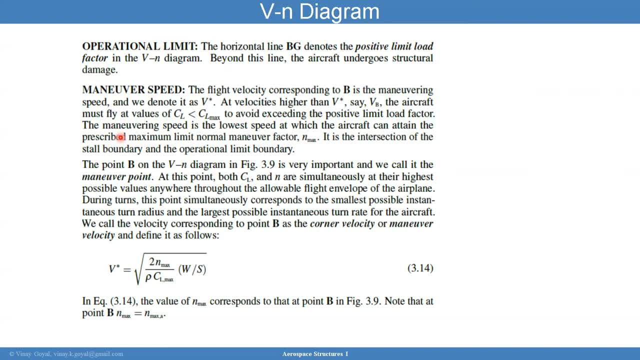 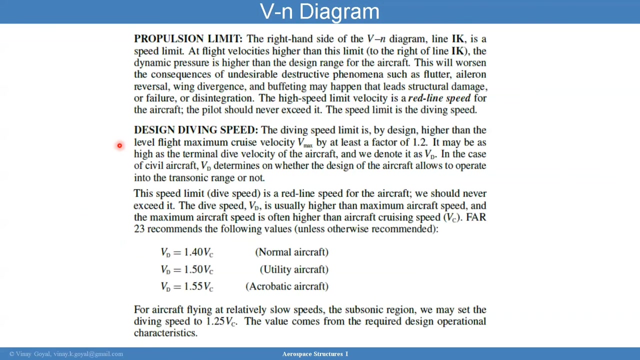 as the corner velocity, corner velocity or maneuver velocity, And we can define it as such. So I can define it as such, Okay, So there you go, That's how you calculate that. And here again the maneuver speed. we're talking about that point here. 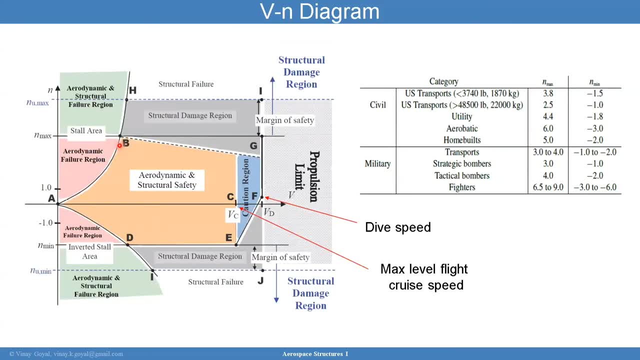 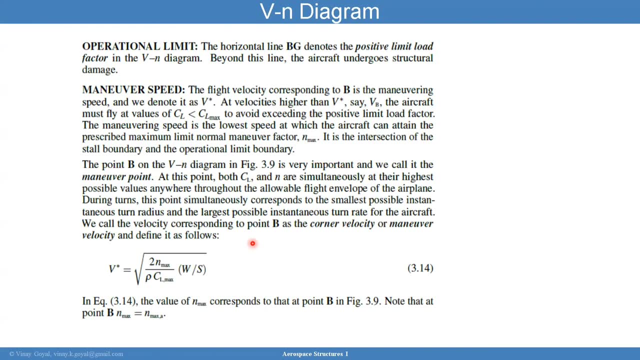 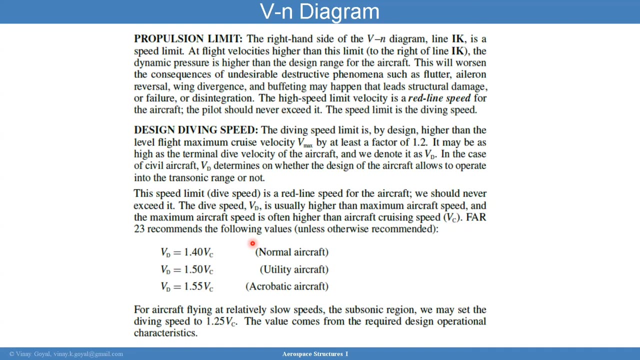 And proportion limit. we already covered the proportion limit. That's this line. I from I to like this line right here, right. And that line is a speed limit. As velocity is higher than this limit, the dynamic pressure is higher than the design for the aircraft. 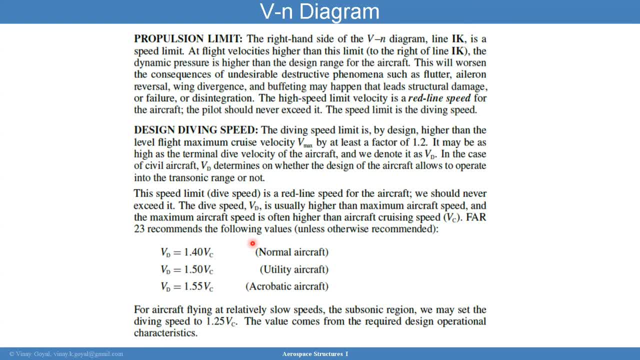 So that will not really. that's going to cause flutter, aileron reversal, wing divergence and buffeting, which will lead to a failure and disintegration. So the high speed limit, velocity- we call that the red line speed for the aircraft. 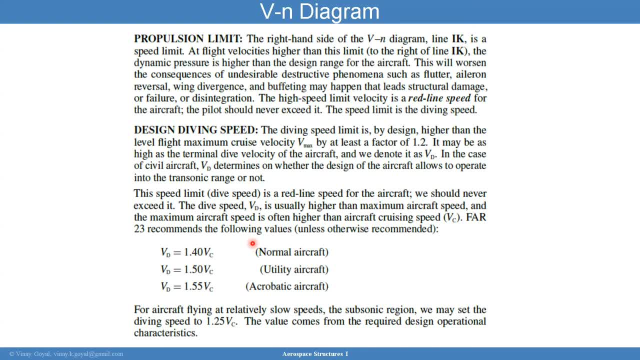 and the pilot should never exceed that The speed limit. there is the diving speed, So designing for diving speed. typically the diving speed for a normal aircraft is about 1.4 times the cruising speed. I'm sorry, I apologize, And the diving speed limit is by design. 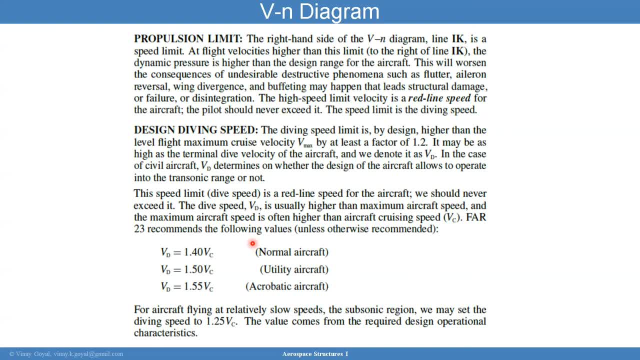 higher than the level flight cruise velocity V max: usually by at least a factor of 1.4.. At least a factor of 1.2.. But typically for a normal aircraft 1.4. It may be as high. 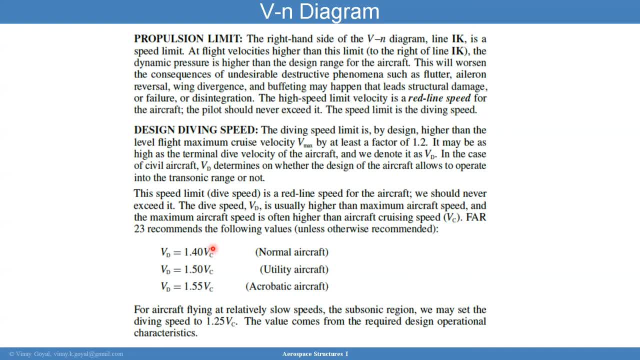 as the terminal dive velocity of the aircraft. In the case of civil aircraft VD, the dive velocity determines whether the design of the aircraft allows to operate into a transonic range or not. This speed, this dive speed, is a red line speed for the aircraft. 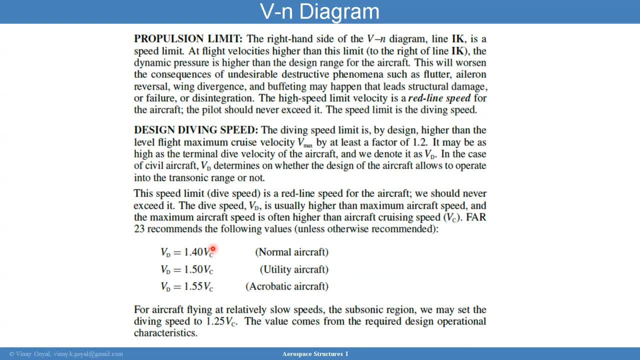 We should never exceed that. Never For FAR 23,. we recommend these values, as I said, And for aircraft flying at relatively low speeds. subsonic region, you can set the dive speed to be one and a half- 1.25,. 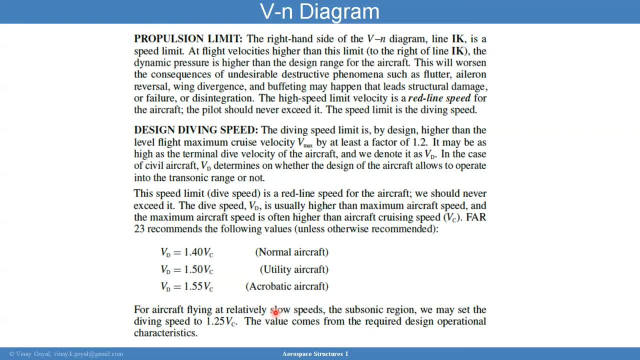 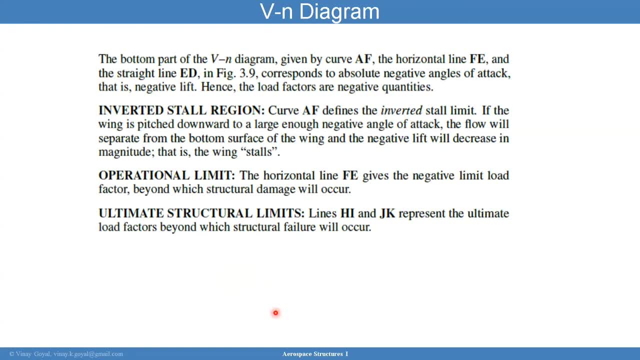 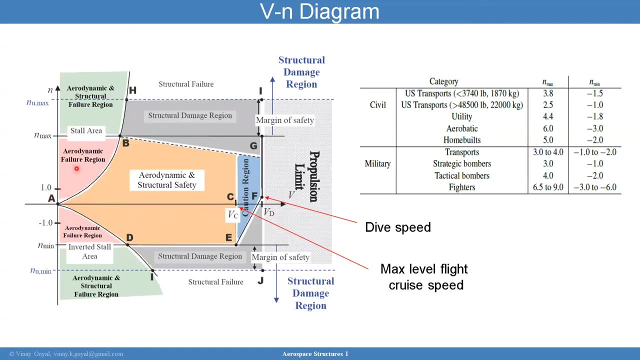 the cruising velocity, And this value comes from the required design operational characteristics. And then now the bottom part of the VN diagram is given by the curve AF. Let me show you the curve here. So the curve is. we want to talk about this curve here. 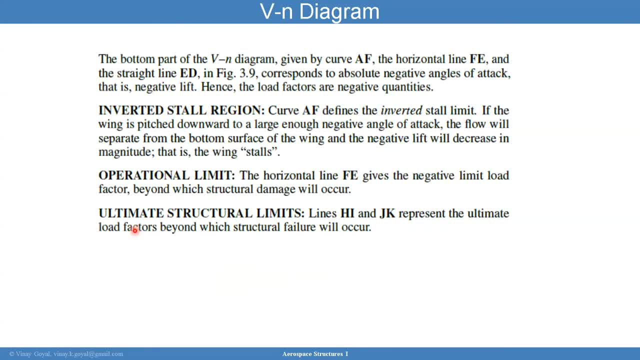 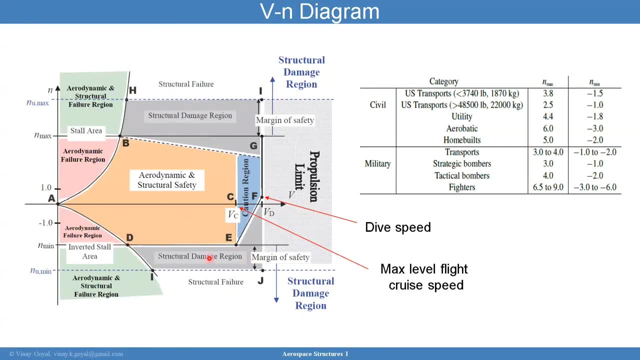 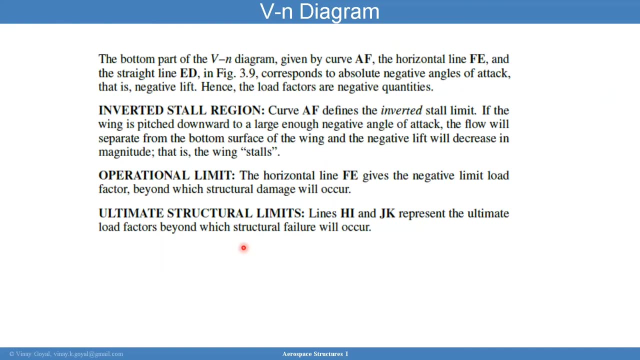 And the horizontal line. this horizontal line, so this should be this line, This should be F here. So that curve right here, AF and FE, that's your safe zone there And it corresponds to absolute negative angles of attack. That means you have negative lift. 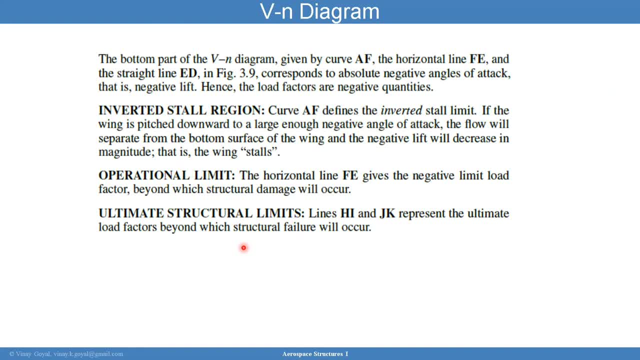 hence the load factors are negative quantities. An inverted stall region where the curve AF defines the inverted stall limit. If the wing is pitched downward to a large enough negative angle of attack, the flow will separate from the bottom surface of the wing and then you will get a negative lift. 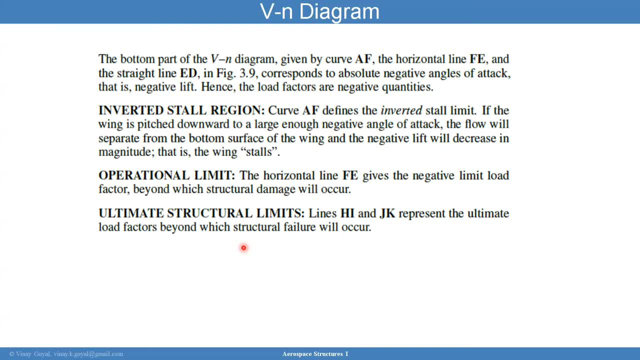 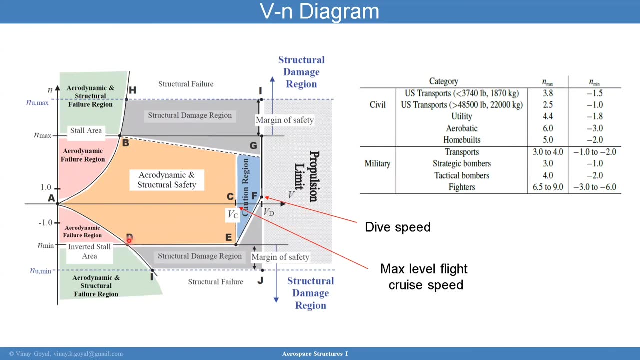 And the wing could stall The operational limit. the horizontal line is DE in the plot gives the negative limit load factor. beyond you can have structural damage. So this should be FE. this should be F. this should be F, not D. 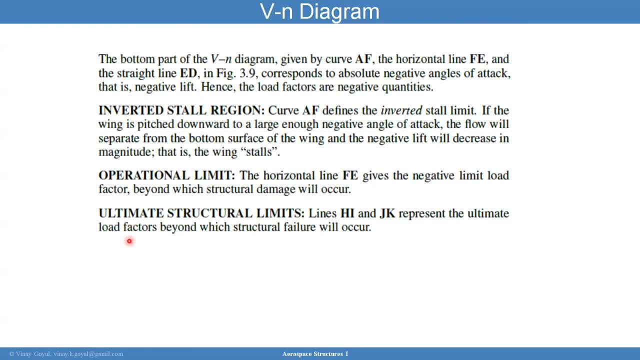 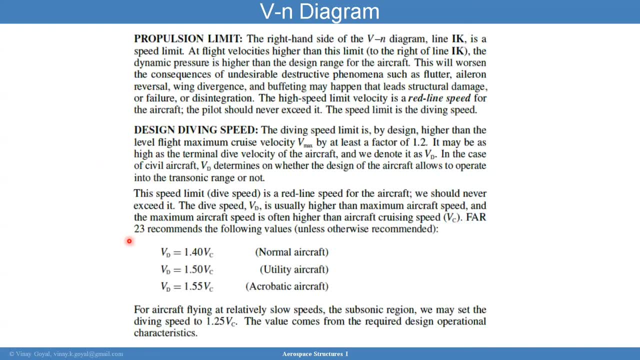 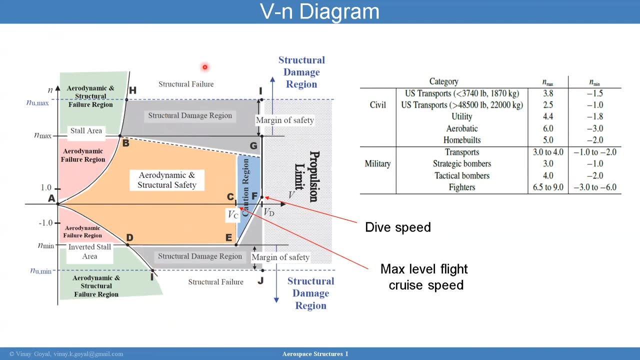 and that's why that's getting confusing- And the ultimate structural limits. the lines HI and JK represent the ultimate load factors beyond which structural failure will occur. So that's these lines here, HI and IJ. Beyond these you're going to have structural failure. 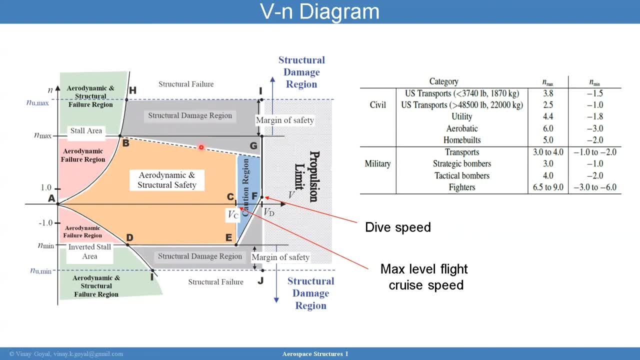 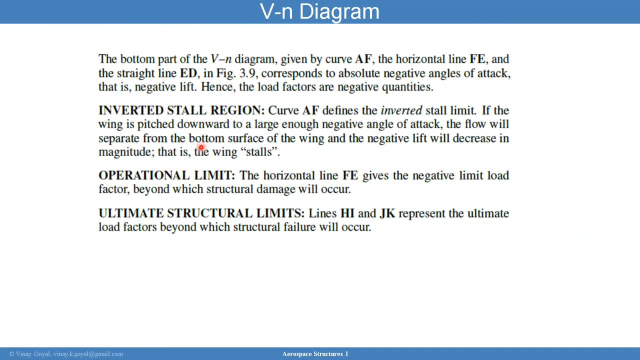 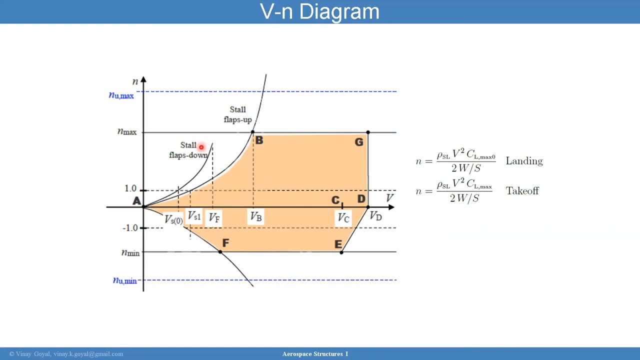 Here in between you could have some amount of structural damage. So very important consideration as you're moving forward. that's going to drive your design. That's going to drive what the design looks like When you put the flaps down and when you put the flaps up. 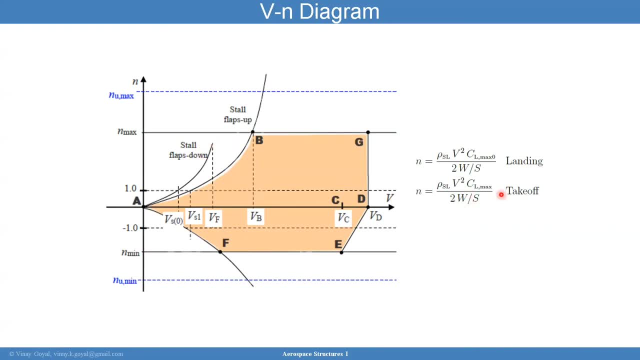 it's going to change the behavior during landing and takeoff. It's a very important consideration. During landing and takeoff, you're going to have different values, And so you could have a different VN diagram because of the influence of the landing and takeoff. 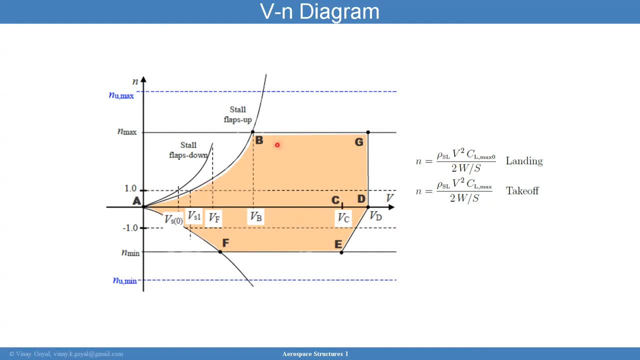 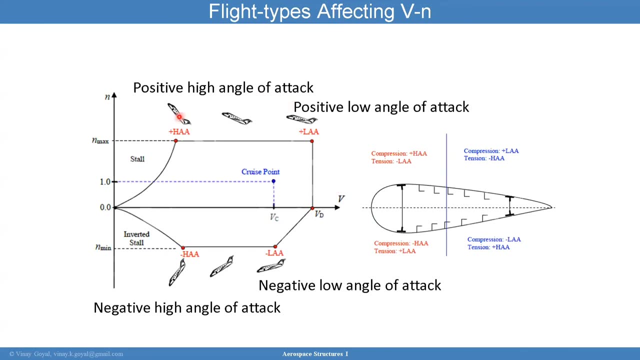 on the load factor. So that's going to change this VN diagram behavior. A positive angle of attack means you're over here in the top at positive load factors And then you have a negative high angle of attack if you're down here. 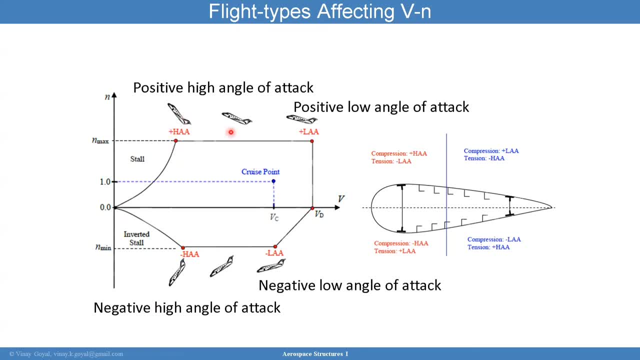 And you can see here: high angle of attack, low angle of attack. So high angle of attack, low angle of attack. The higher the velocity, the lower angle of attack. It forces you to have a lower angle of attack if you're going to a higher velocity. 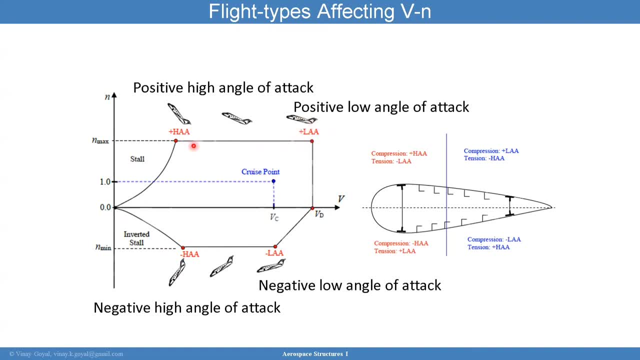 Because I need a lower lift coefficient. that's why- And then here I can be a higher angle of attack if I want to maintain that particular load factor, And then very similarly negative high angle of attack if I'm at very low velocities. 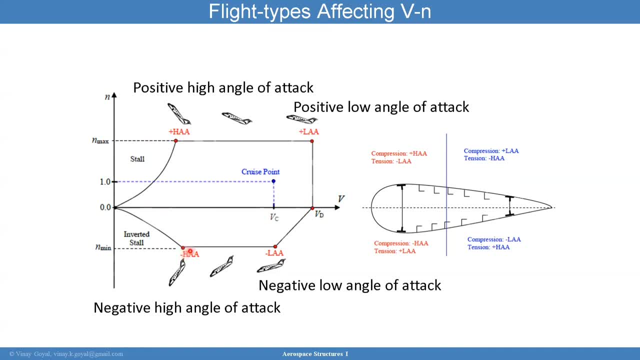 and I want to keep the same load factor Again. angle of attack really increases the load factor, And so that's why that's important to understand what's going on here And so you can see here on the wing croc section, what is going on. 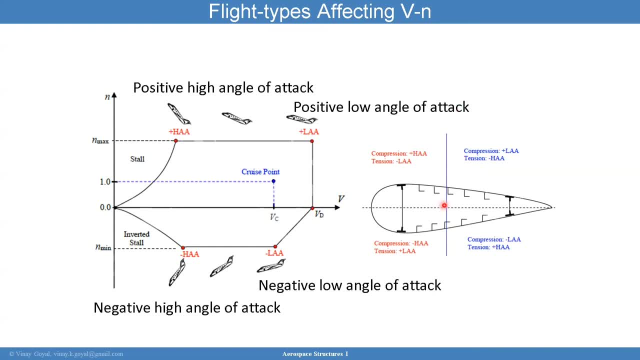 If I drew a quadrant just about like that, the top left quadrant, you're going to have a compression behavior at a high angle of attack, tension behavior in a low angle of attack And then here at the bottom you can see bottom left quadrant. 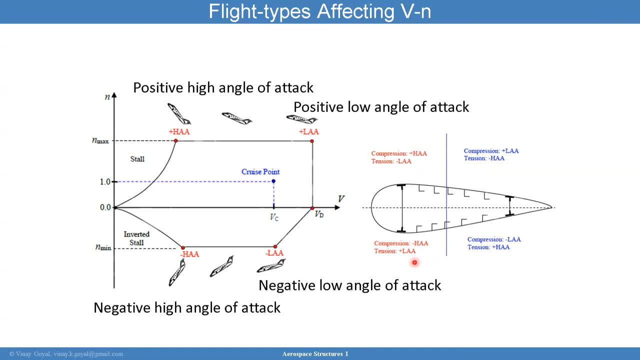 is a compression- high angle of attack, tension- low angle of attack. On the top right you can see compression- low angle of attack, tension- high angle of attack. On the bottom right you have compression- low angle of attack and tension- high angle of attack. 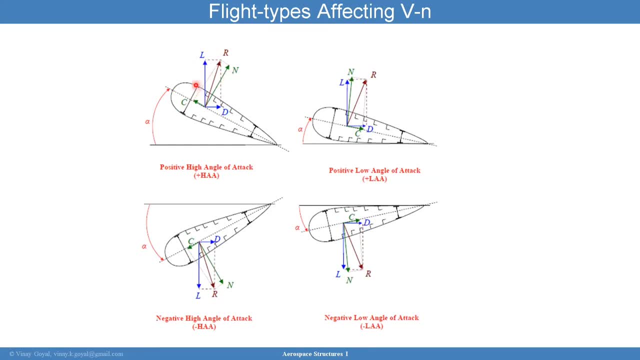 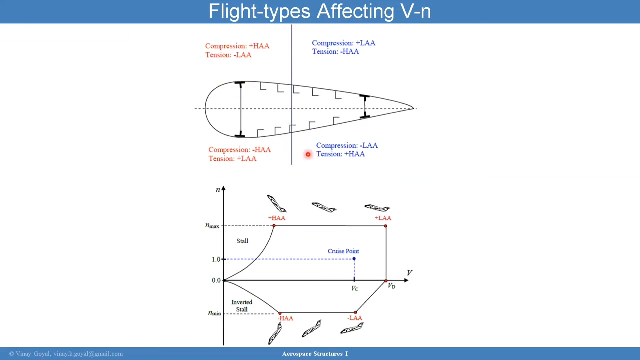 And here again more pictures showing what's going on: Positive high angle of attack, positive low angle of attack. and then here you have negative high angles of attack And again showing you how this maps into the curve below the VN diagram. 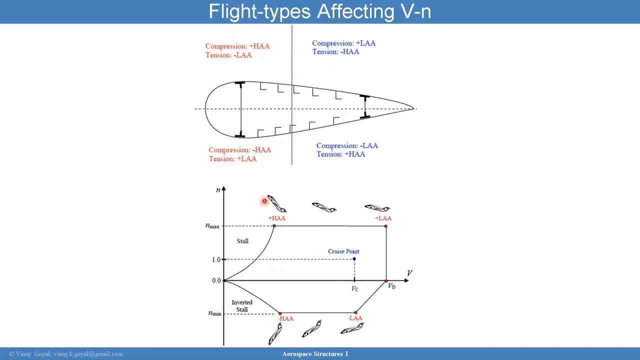 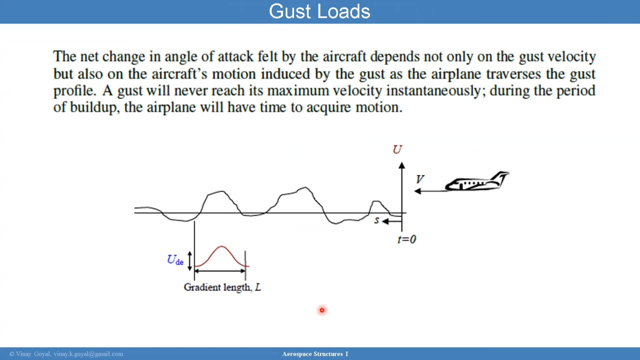 So high angle of attack compression on the top and you can see here that matches this point, And so you can just keep looking at the different quadrants to see where are you matching this. Another important consideration is gust loads. Gust loads need to be considered. 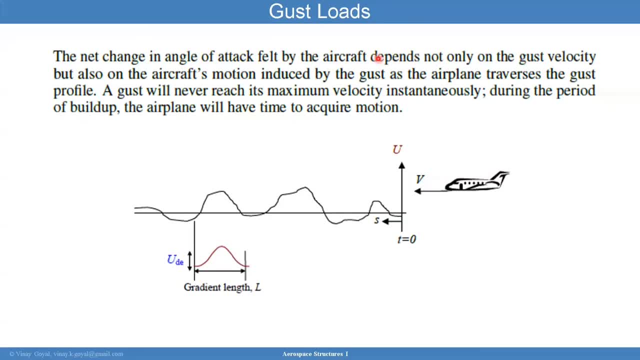 And so gust loads. the net change in angle of attack is felt by the aircraft, And it depends not only on the gust velocity but also on the aircraft motion induced by the gust as the airplane goes by this gust profile. So say you have this gust profile here. 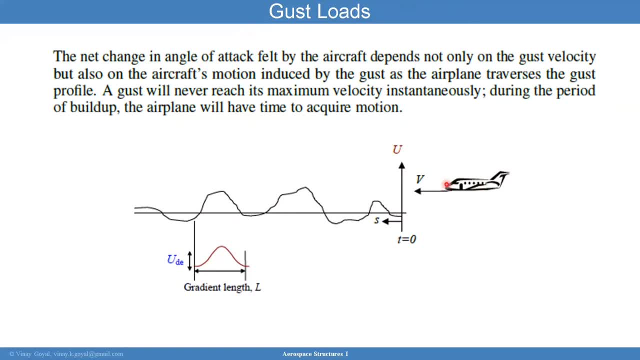 and you have a velocity in this manner and the aircraft is transversing, that that gust will never reach its maximum velocity Instantaneously. During the period of buildup, the airplane will have no time to acquire that motion. So therefore, and you can see here that- 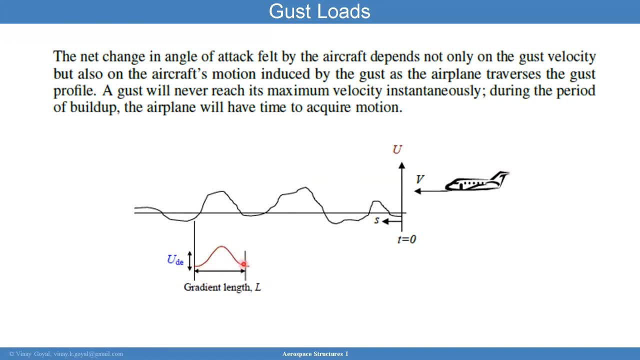 if I look at this curve right here, that's the gradient in length And then that's a change in velocity for that gradient in length. I'm looking at a particular area here of that gust And so very typically you approximate this gust. 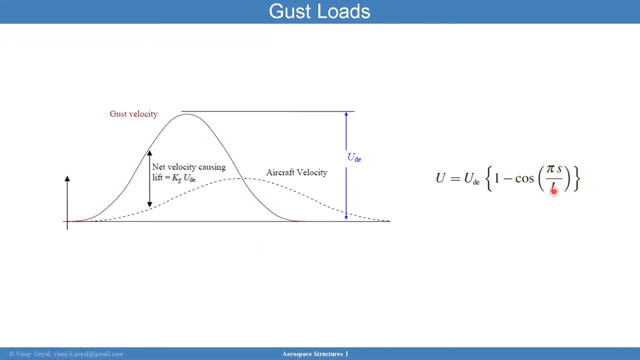 as a cosine function. here pi S divided by L, So that's your gust. velocity, That's how that's approximated using this cosine of this formula here, And so then you take that and the aircraft velocity is this right? So that's your aircraft velocity. 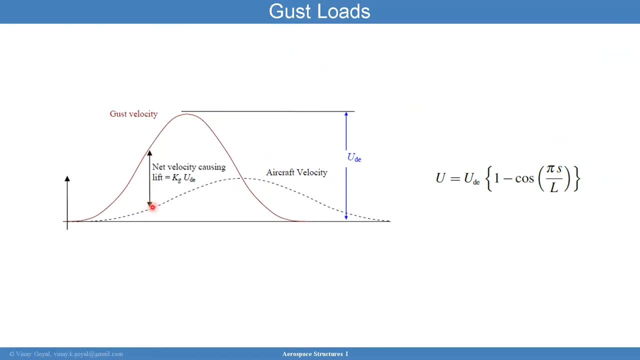 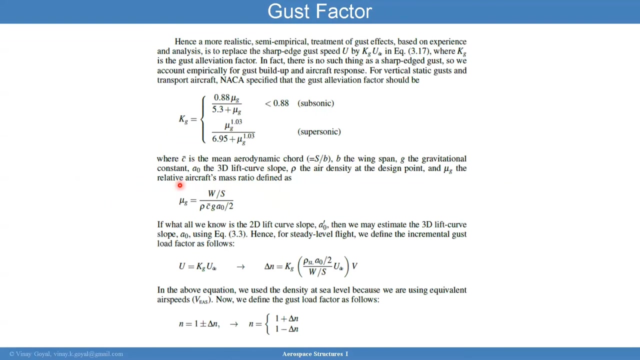 And then this becomes your net velocity causing lift. And so you have to take this kg factor multiplied by UDE to get the net velocity causing the lift. That's typically how that's done And how you calculate that kg. that kg is calculated through these formulas here. 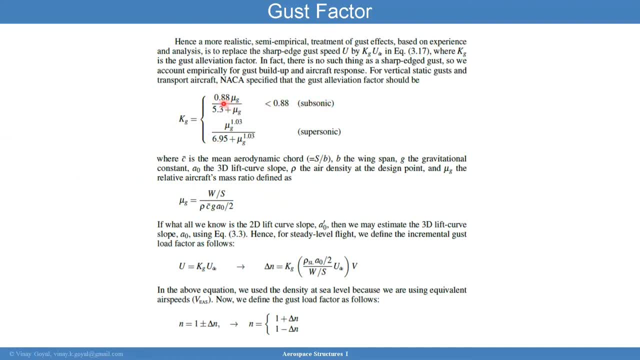 For subsonic less than 0.88, you're going to have a formula that looks like this: Okay, And then for supersonic, you're going to have a formula that looks like this: Now, mu g is the relative aircraft mass ratio. 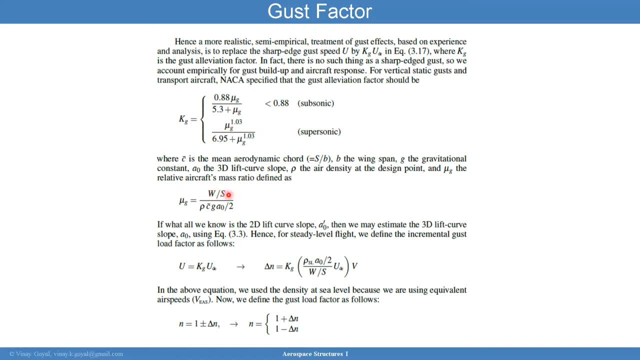 which is defined by another formula: W divided by S, rho, C bar g, A naught divided by two. Now that all this is in my book is described very carefully And if all we know is a slope A naught prime, then we can estimate a 3D lift curve slope A naught. 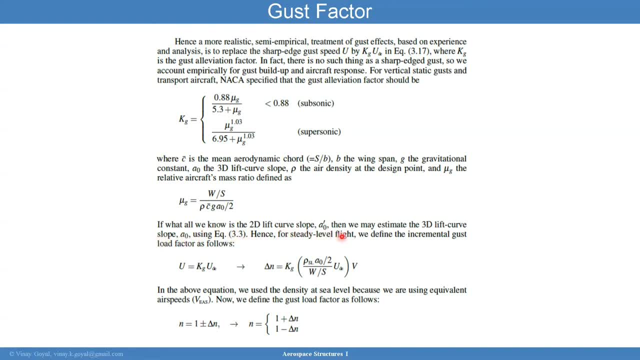 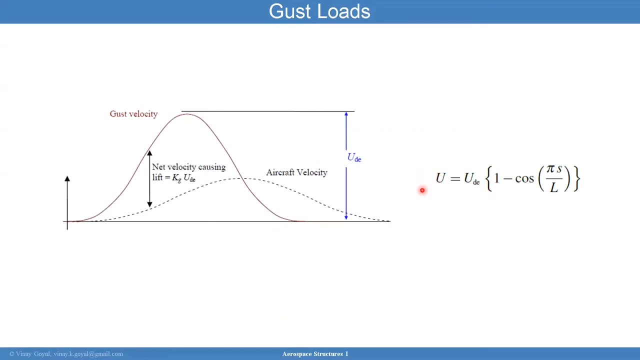 And I provide this in my book. Hence, for steady state flight, we can define an incremental gust load factor as follows: The velocity U okay, equals kg UDE. That's what we talked about here, right, That's the gust. velocity equals UDE. 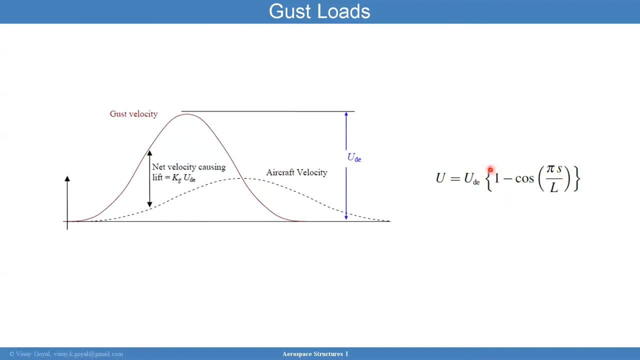 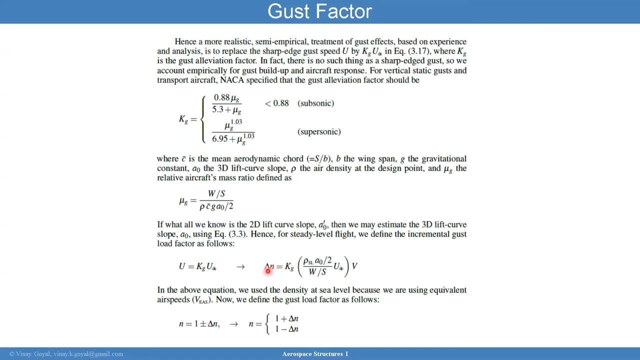 times this cosine behavior here, And so we're taking kg and multiplying by that. That's what this is, And now I can calculate the incremental load factor due to this gust, And so that's going to be kg times this formula here, times V. 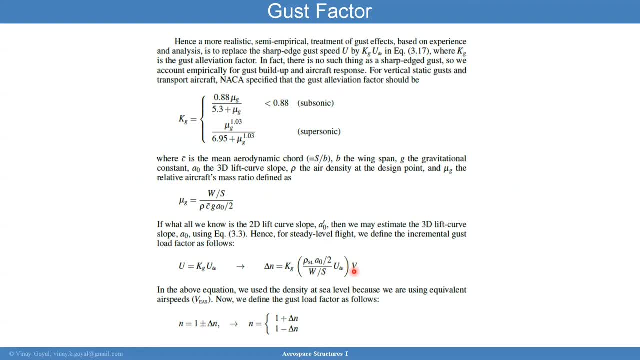 And we're using the equivalent error speed here. So, yeah, that's how you will do it, And now we can define a gust load factor as one plus minus delta N, And N is going to be either one plus delta N or one minus delta N. 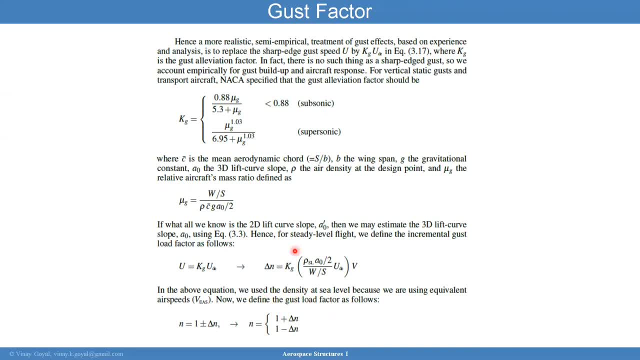 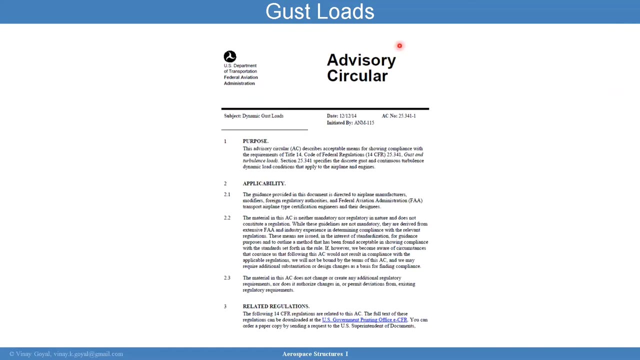 depending upon what's going on with the gust. So that's how you do this calculation And so that shows you the treatment of gust effects and how to deal with that. Now I want to point out that this advisory circular goes into the dynamic gust load factors. 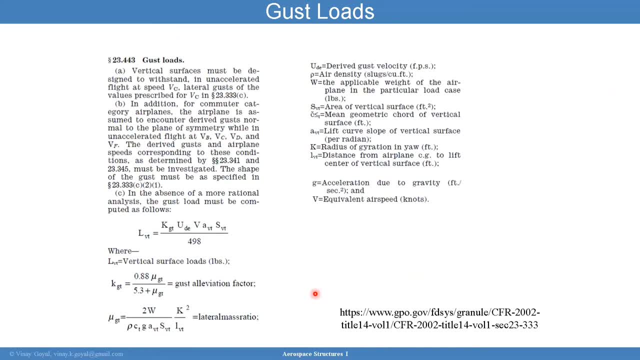 in a lot more detail And here is from the government website. It shows you the formulas I'm showing you here are consistent to the requirements as written in 23.443 in the Federal Aviation Regulation Standards And it tells you basically the vertical surfaces. 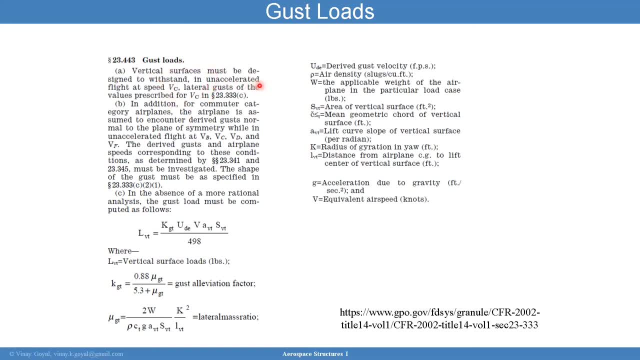 must be designed to withstand, in an accelerated flight at speed cruising velocity, lateral gusts of values prescribed by the cruising velocity. In addition, for commuter category airplanes, the airplanes assumed to encounter derived gusts normal to the plane of symmetry, while an unaccelerated flight. 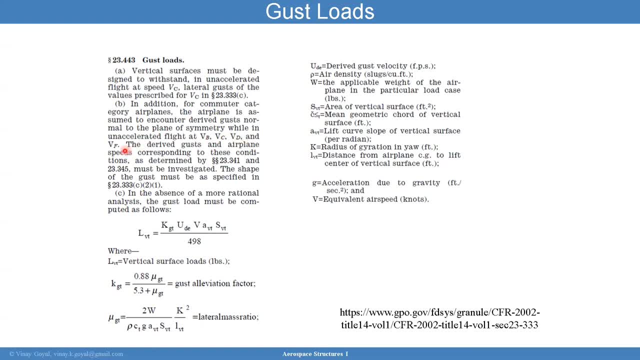 and then it tells you VB, VC, VD and VF. Those are the points in that VN diagram that we talked about, that the derived gust and airplane speeds corresponding to these conditions are to be determined based on these articles here and must be investigated. 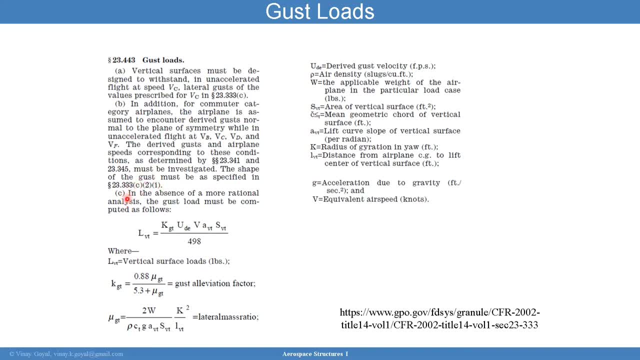 The shape of the gust must be specified, and is going to use the cosine function I talked about. In the absence of a more rational analysis, the gust must be computed as this, And so that's the gust load that you have to consider, And that's the load on the vertical surface. 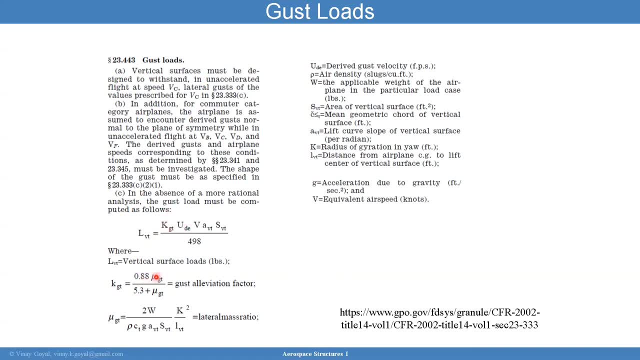 And then now you have this calculation that matches exactly what I showed you earlier, And the mu is the lateral mass ratio I showed you earlier as well, And all these parameters will match exactly what I just showed you And you can see the impacts of gusts. 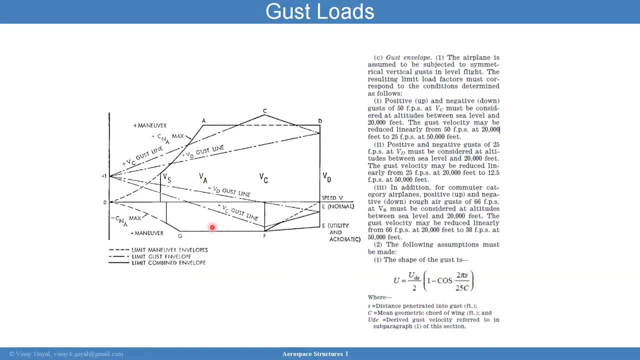 is going to change the VN diagram, the shape of it, And so when you're designing an aircraft, you want to design for an envelope that envelopes both the gust line load and envelopes the no gust load. So, however, the VN diagram looks more expanded. 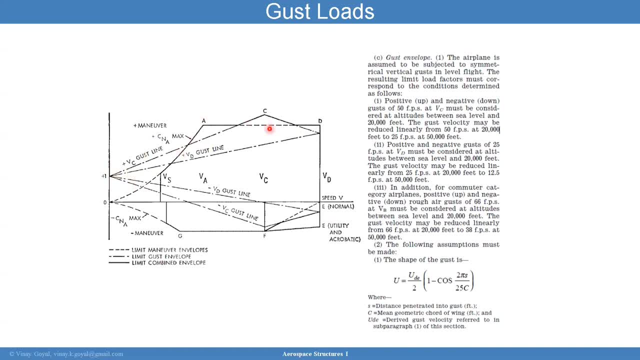 whether by the gust line or the maneuver. you want to have that envelope fully taken care of, And that's what this is talking about here. That's a formula I just told you about, that's in my book and is in the Federal Aviation Regulations. 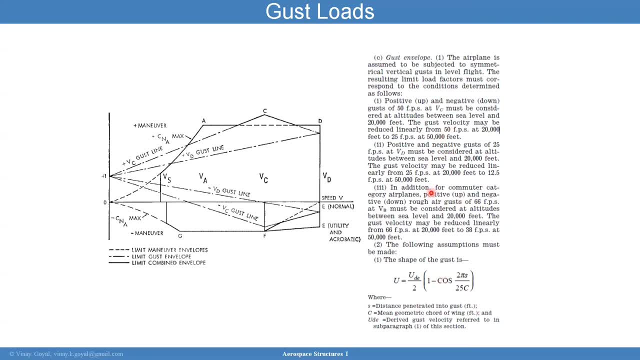 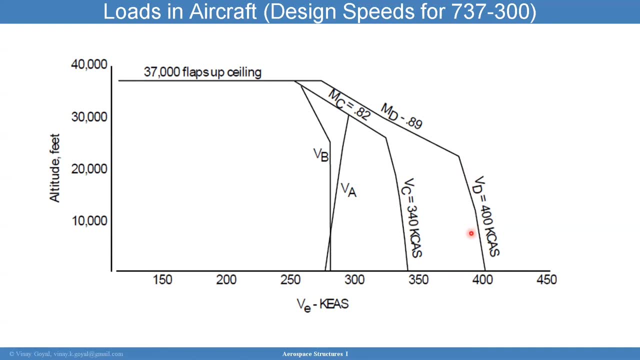 It gives you additional information here about this. The 737 you can see here has a dive speed and then you have your cruising speed And then you can see that's corresponding to Mach 0.82.. This is Mach 0.89.. 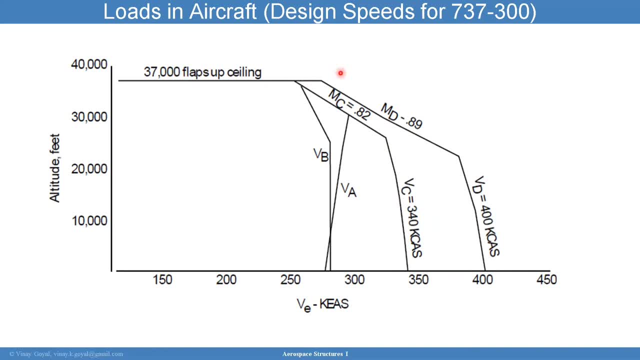 And again very similar. And then you have your 37,000 feet flaps up ceiling. So this is not your VN diagram, but shows you the altitude as a function of airspeed, equivalent airspeed for a 737.. And my point here is to show you. 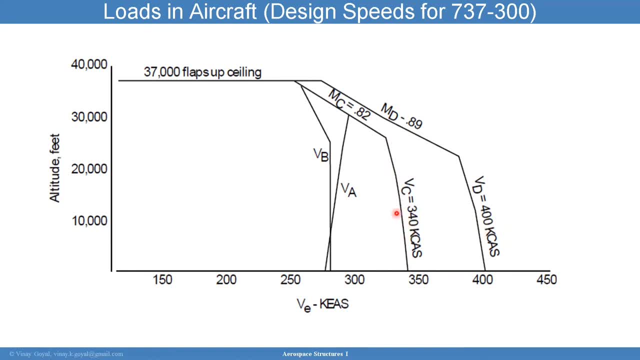 that difference between dive speed and cruising speed. And you can see here that as I go higher in altitude then these values change, because I'm calculating according to this equivalent airspeed. That's why that's happening. The air is lighter as you go higher up. 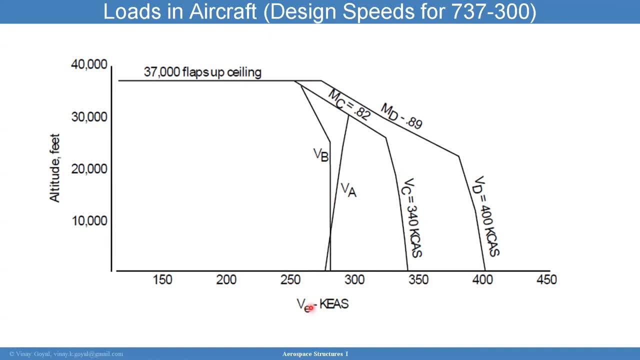 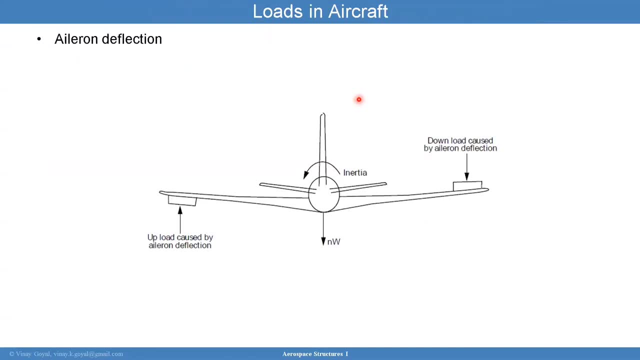 So it's less dense, And so then your equivalent velocity decreases because of that. Again, I'm doing everything in reference to the sea level. So what are the loads in an aircraft? You have the airline deflection. That's one type. 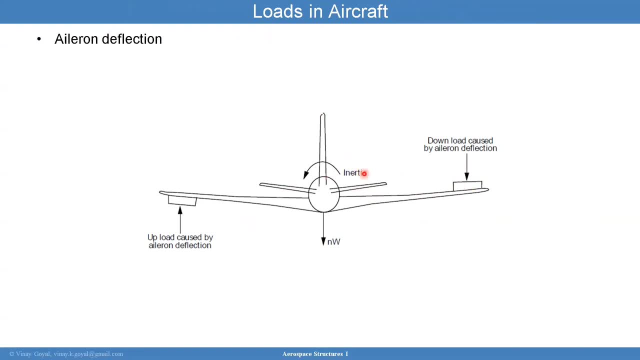 You apply airline deflection, you get a roll and then you have the inertia and the load factor here. So you can construct with the lift applied, you can construct a free body diagram that basically tells you what is the distribution of the lift and the load shear and bending across its wing. 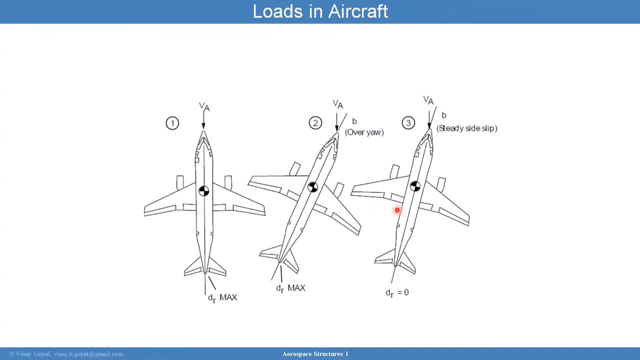 Then you have loads in an aircraft that are caused by this yawing of the rudder. So if I put a rudder deflection you're going to have an amount of deflection. The aircraft is going to have a side slip. 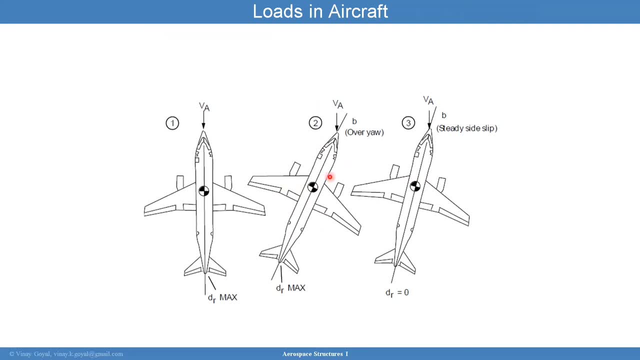 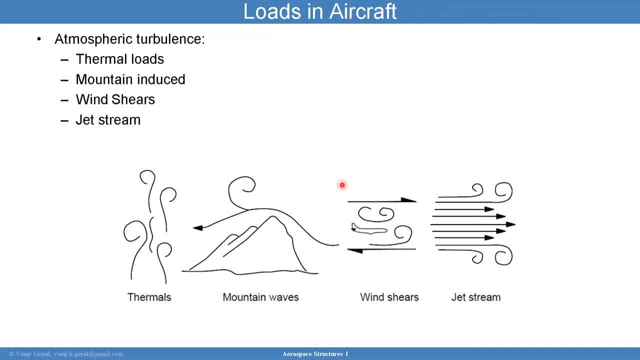 And so you can then construct a free body diagram to account for a side slip condition. Loads in an aircraft are going to entail thermal loads, mountain induced wind, shear, jet stream. These are very. these are loads that are going to impart additional loading into your aircraft. 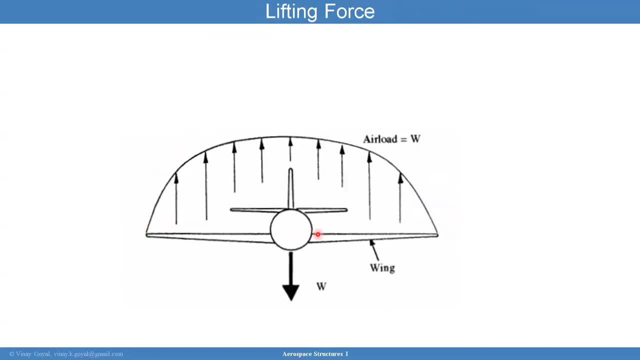 Lifting force typically is going to have a distribution like that. That's your wing And now that you have this lifting distribution, you can do cuts to figure out if you treat this wing as a beam. you can then do cuts to figure out the bending moment. 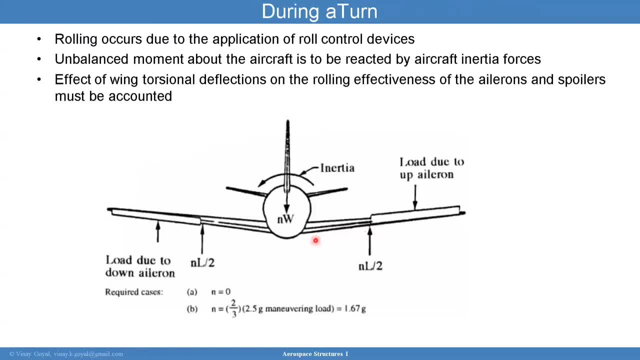 and the shear diagram and then use that to size your design. I'll come into that a little bit later During a turn. so you're taking a turn. rolling will occur due to the application of the roll control devices. An unbalanced moment about the aircraft. 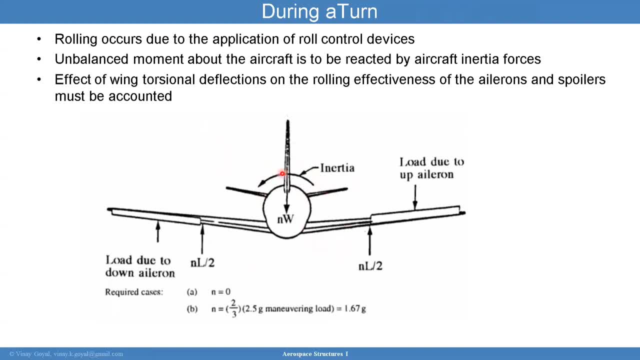 has to be reacted by the inertial forces. You can see that here, And so here's a load due to the aileron deflection. You expect it to roll to the right, and then this inertia is counterbalancing that: The effect of wing torsional deflections. 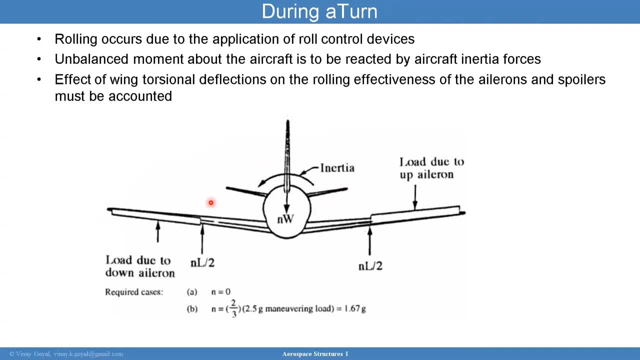 on the rolling effectiveness of the ailerons and spoilers have to be accounted. You have to account for that, But again you can. now the required cases here is: N equals zero and N equals two over three, two times 2.5 G maneuvering loads. 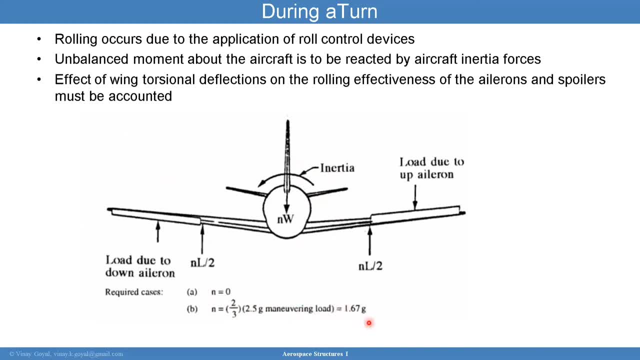 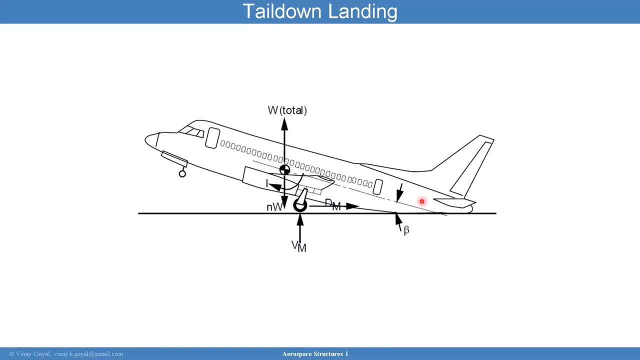 That gives you a 1.3 G maneuvering load 1.67 G. So these are required cases to be analyzed. You also have the tail down landing, where you get a tail strike here, And so you get a lot of loading here. 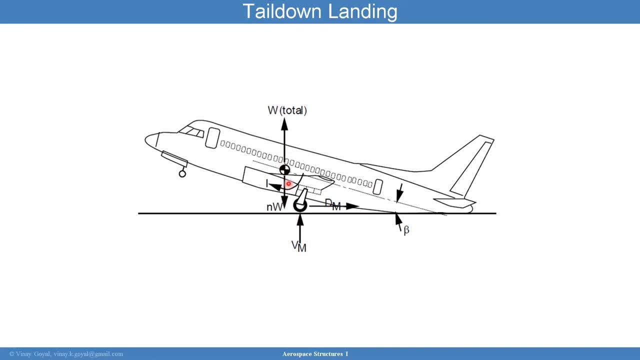 And that needs to be looked at and analyzed. You can see here I have the weight, I have N times W, You have the inertia loads And then you have the loading at the wheel, because you're going to hit the wheel as well, and then the drag in this direction. 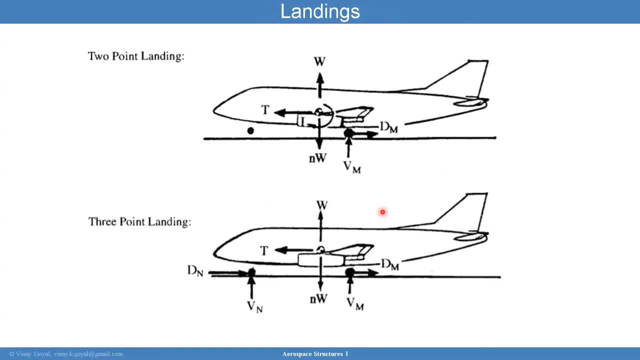 And you can again draw a free body diagram of this. You have the two-point landing. I promise I'll touch on that, The two-point landings. at the back end of the aircraft, the wheels are touching the ground, So you have the normal load here. 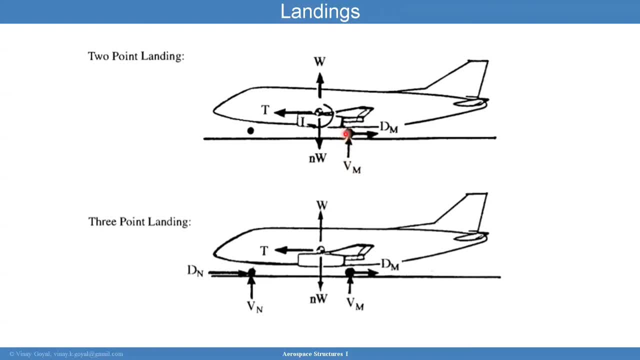 It's a reaction. This V is not a velocity, It's a reaction force. And then you have here the directional forces. These are thrusts because you're moving forward. That's a weight. And then you have N times W Again. 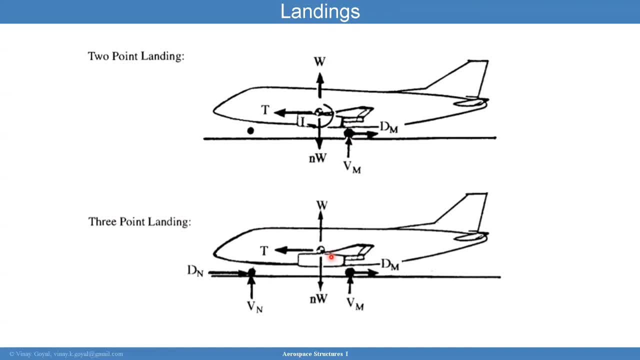 three-point landing again, And here the lift got inverted because you're pushing the aircraft downwards against the ground And you can see here that for three-point landing now I have some sort of forces in the front wheel. You could also have a single wheel landing. 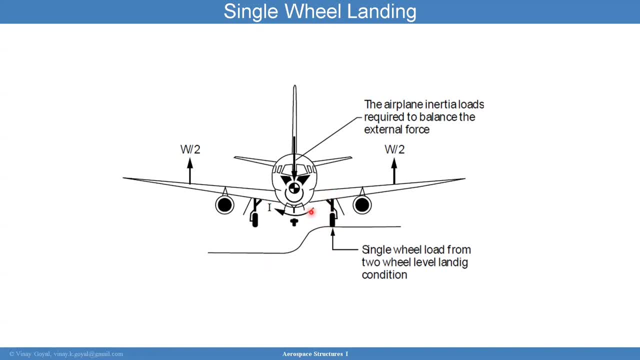 That's going to cause you to do a lot more work in terms of you know, the loading is going to be such that you're going to have to draw a free body diagram again. So see, here you have a single wheel condition, Here in the single wheel condition. 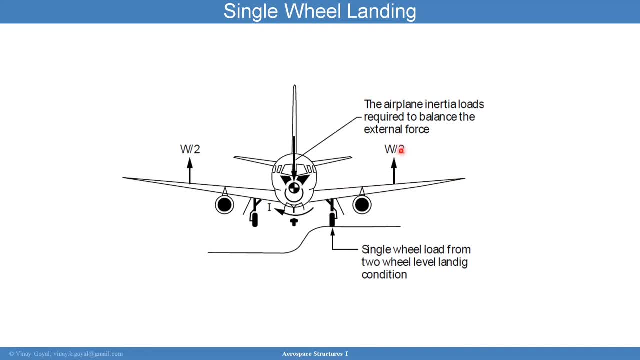 you have a huge amount of shear across these two loads And the airplane. the inertial loads is going to cause it to be in equilibrium. Without that, the whole aircraft will crash. So inertial loads, Newton's law- is really helping us keep this aircraft in check. 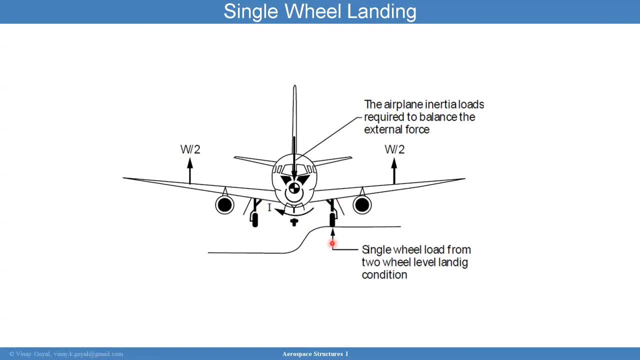 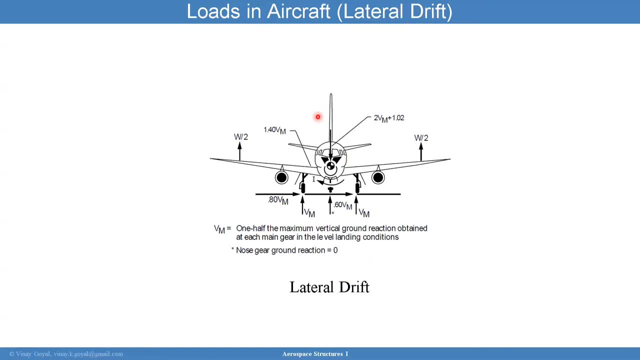 And you can see here those inertial forces are going to balance a single wheel load. You also have loads in aircraft due to lateral drift. So say we have some amount of lateral drift, then you have to then calculate the behavior for that condition. 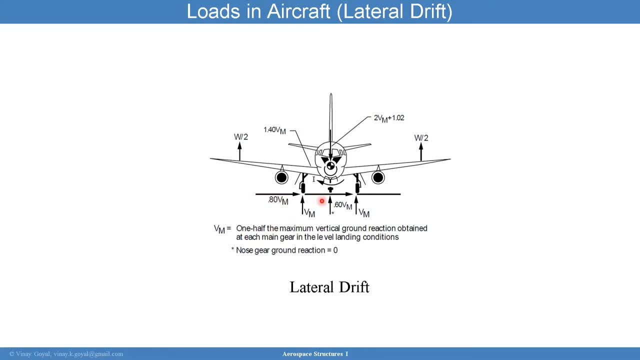 And so you can see if I have a lateral drift, then I have 0.8 here, 0.6 here, So you get a total reaction of 1.4.. And you still have some inertia that has to balance that somehow. 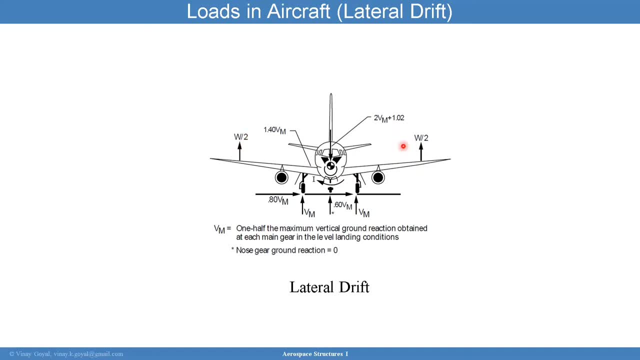 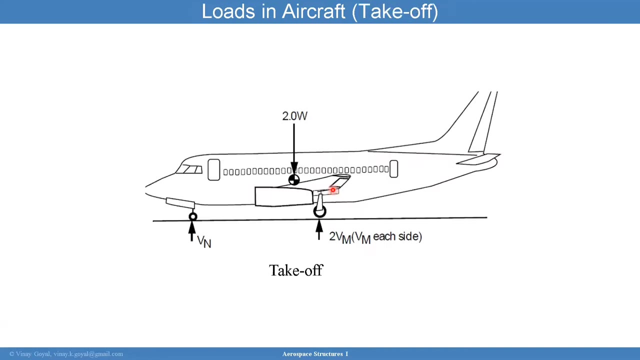 And then you have: this weight is getting balanced as well And the wheels will then also have some amount of it's going to have a reaction force in the front wheels here and the back wheels as well. And these are the general analysis that you will perform. 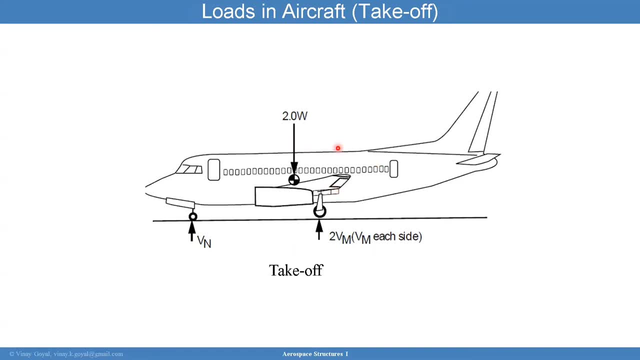 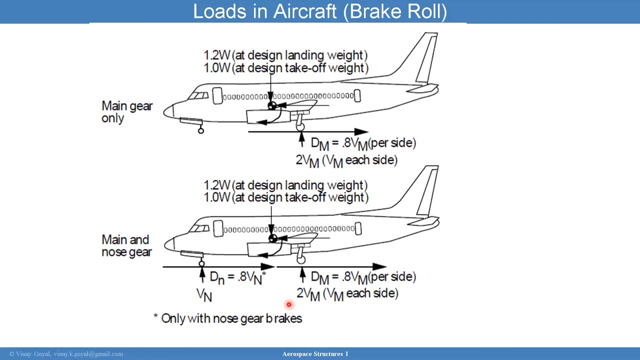 All of this can be done with free body diagram And here you have a takeoff situation: some amount of loading here, some amount of loading here, and then 2.0 times the weight here Brake roll is going to have. you have to look at. 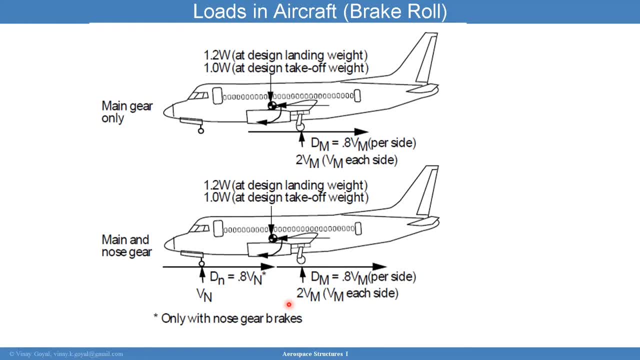 brake roll as well, And from brake roll you also get an amount of loading on the wheels that need to be considered for the main gear only and the main and nose gear as well. So this the design loading that needs to be accounted for in the analysis. 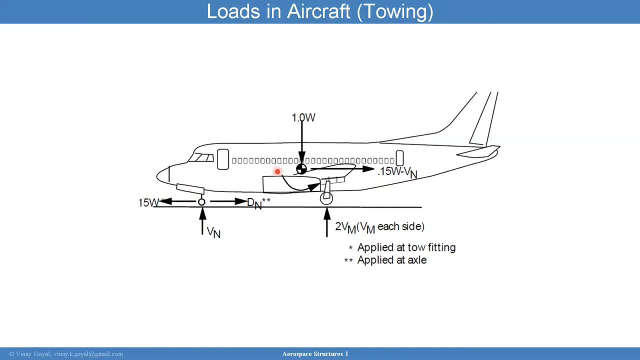 And then here you have towing, So I'm pulling now the aircraft, The weight is 1.0. So that stays the same, And then you just basically have an applied tow lift, applied tow lift at the axle of the nose gear. 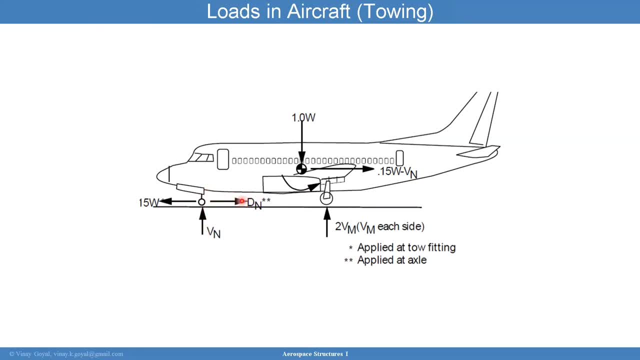 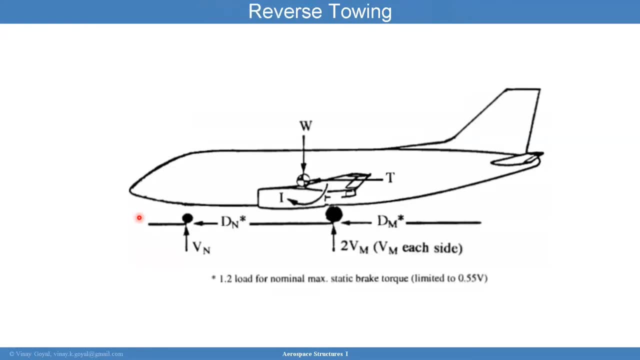 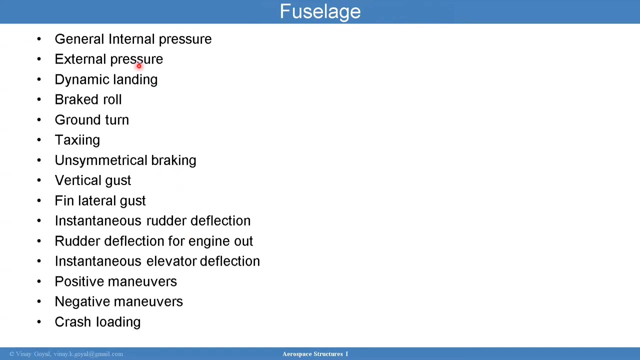 And you also have a force here and a frictional force there- Reverse towing- again, that's different from this one. This is pulling and this is reverse towing, which can also occur. The fuselage has to be analyzed for a number of conditions that I already covered. but I'll repeat them: General internal pressure, external pressure, dynamic landing brake, roll, ground turn, taxing, asymmetrical braking, vertical gust pin, lateral gust and so forth. The engine mount also has to be analyzed. You need to analyze for yawing. 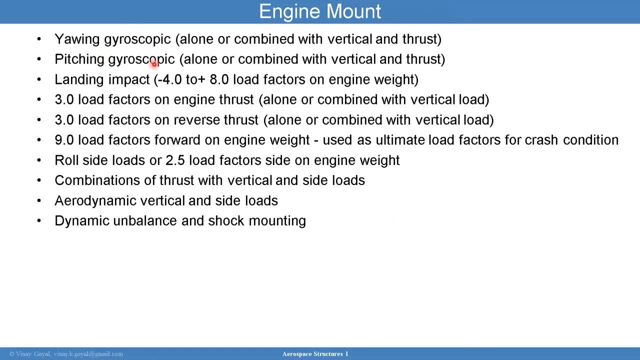 gyroscopic behavior- pitching gyroscopic behavior- landing impact: 3.0 load factors on the engine thrust, 3.0 load factors on reverse thrust, 9.0 times load factors forward on engine weight, And then roll side loads of 2.5 load factors on the engine weight. 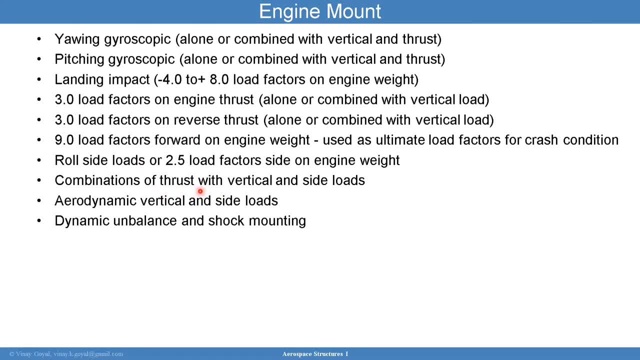 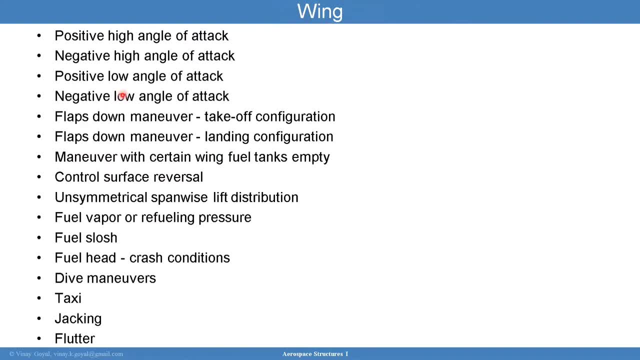 And then you have to combine the thrust with vertical and side loads. So there's a lot of load cases that have to be looked at, for the engine mount is my bottom line And the wing has a number of load cases that have to be looked at. 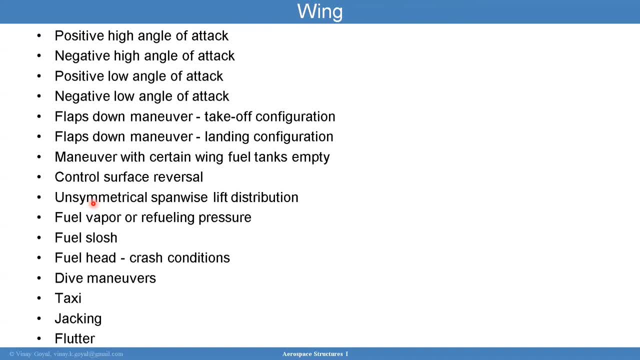 Fuel sludge, fuel vapor: unsymmetric spanwise lift distribution control surface reversal maneuver with certain wing fuel tanks empty flaps down for takeoff and flaps down for landing. negative low angle of attack. positive low angle of attack. 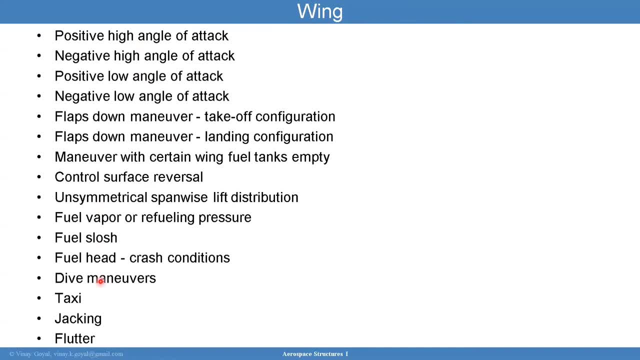 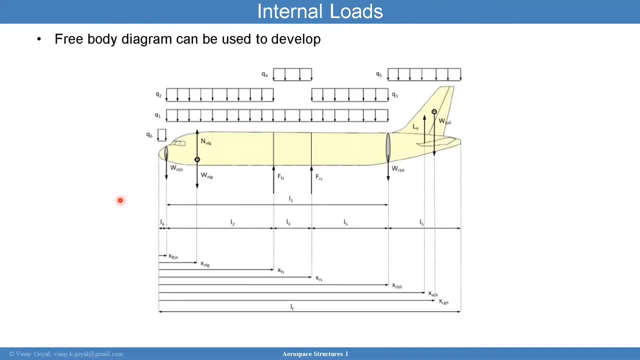 negative high angle of attack. positive high angle of attack. taxi jacking and floater- All these needs to be accounted for the wing, And so how do you go about this? It's a very simple analysis. It goes back to beam theory. 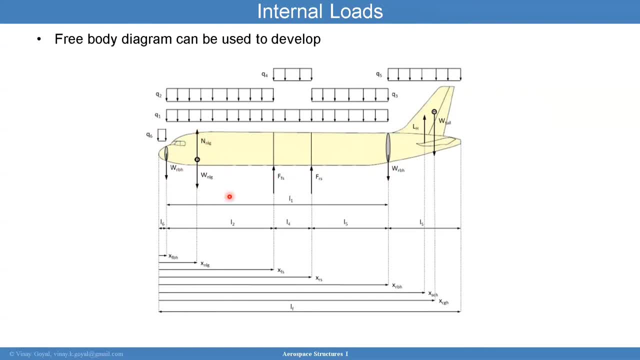 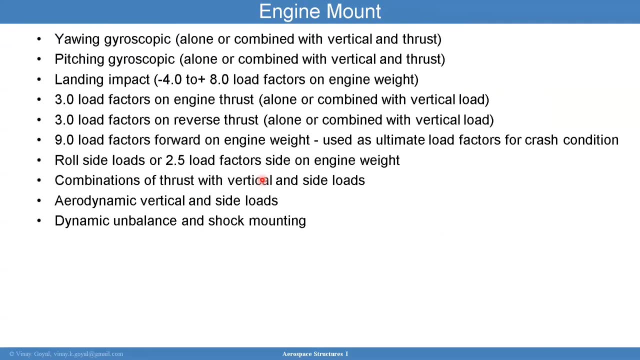 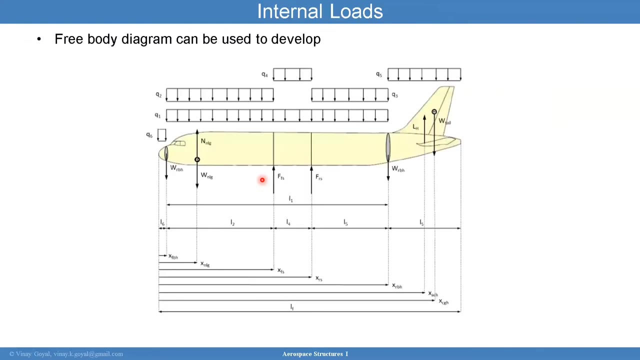 You plot the weights for everything And then you do section cuts to figure out what the distribution is going to be of shear and bending. moment, That's all you have to do. Given these loads, you should be able to tell me what the distribution of shear and bending is across this vehicle. 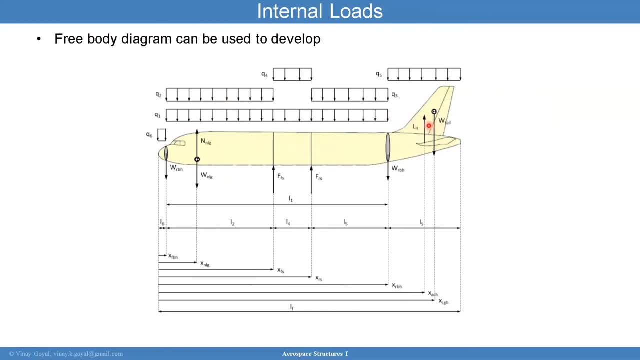 by doing section cuts And you're going to have a lift here on this surface. You're going to have a lift on this surface, So on the wing of course. So you have to do section cuts until you figure out what the shear. 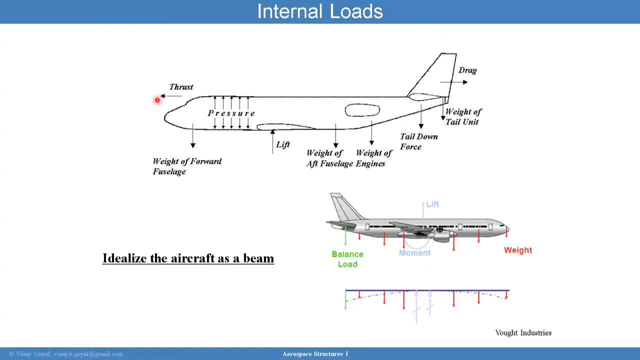 and bending moment diagram are. Here is an example of idealizing the aircraft as a beam, courtesy of Vaught Industries. And you can see I have pressure inside, I have the drag, I have weight, I have tail downforce, I have the weight of the engines. 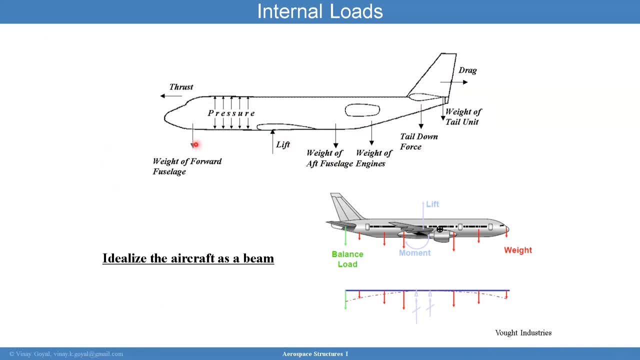 the weight of the fuselage, the lift. So this in the flight configuration, I can still do a cut and figure out the axial shear and bending is at every single cut. based on that information, And if I idealize the aircraft as a beam, 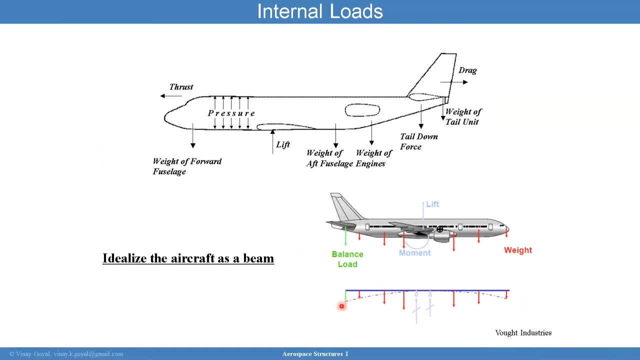 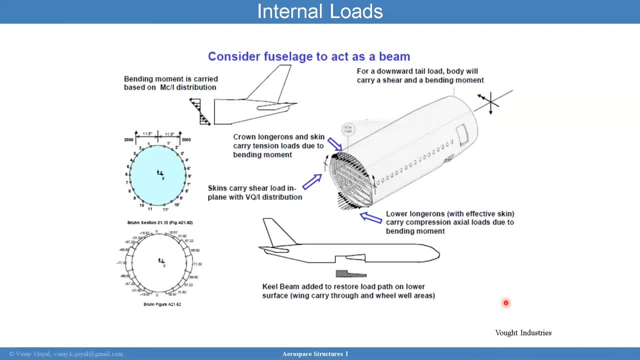 and I were to plot it. it's going to look something like this: right, You can do the calculation at home with a real problem. So for internal loads, what you're going to do is, once you have the internal loads, you have the shear and the bending. 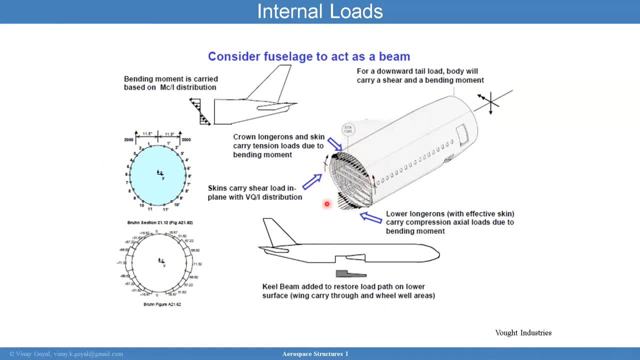 you're going to start studying how that's going to translate into the fuselage skin and the longer run. So the bending moment is carried based on the MCE over I. You've seen that formula before. Stress equals MCE over I. That's exactly how that cross-section is going to behave. 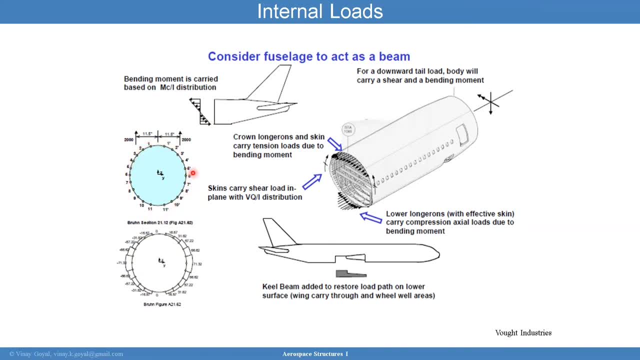 And here you can see the different stiffeners And you can see how the bending is going to get distributed here. at the bottom left Crown, longer runs and skins carry tension loads due to the bending moment, So these are going to carry the tension loads. 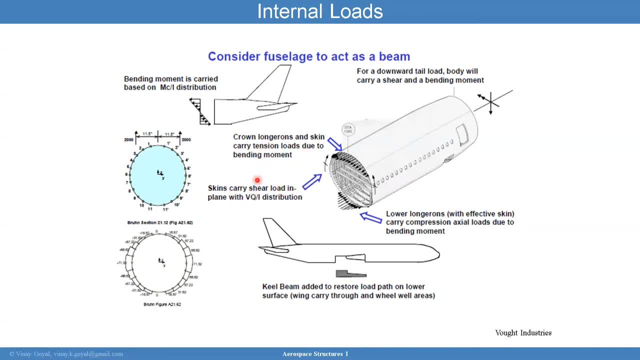 The skins also carry the shear load VQ over I. You've seen this in mechanics and materials. In the lower longer runs we'll see compression due to the bending moment. in the way we plotted it, You can see there's compression here. 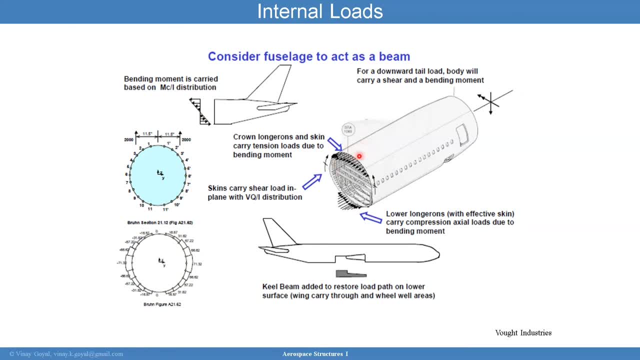 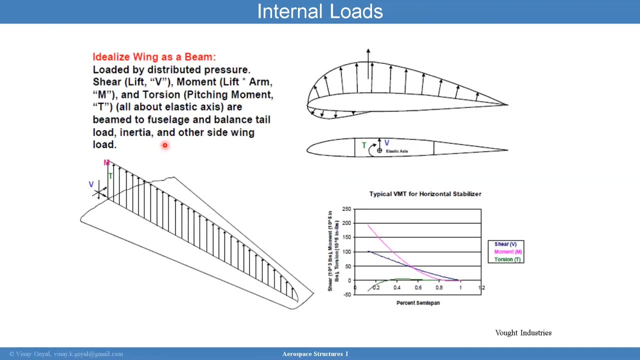 tension there. So that makes sense, And you will then basically plot that as a functional location and simultaneously calculate the shear on the panels on the skin and then the axial or compression loading on each of the longer runs For the long runs. 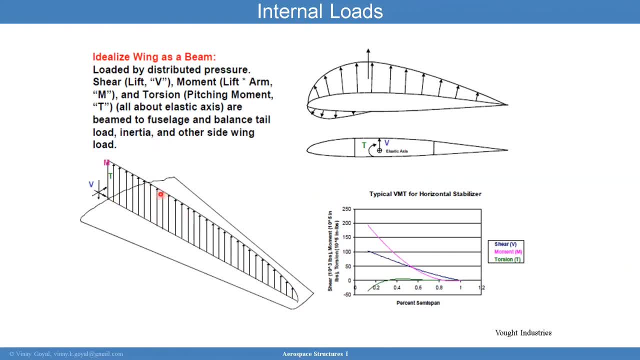 you can also idealize that as a wing. And if you idealize that as a wing, you can calculate the distributed pressure, You can calculate the moment and the shear- if I do cuts- And you can even calculate the torsion, And that's going to help you figure out. 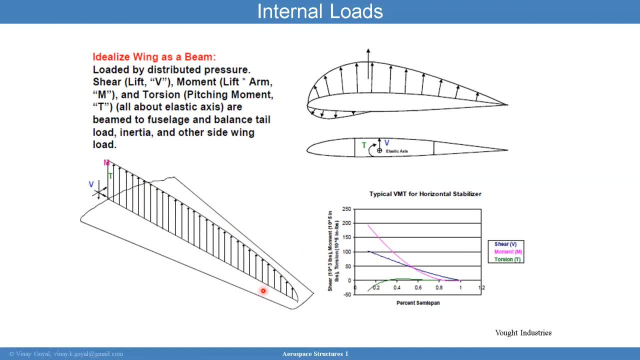 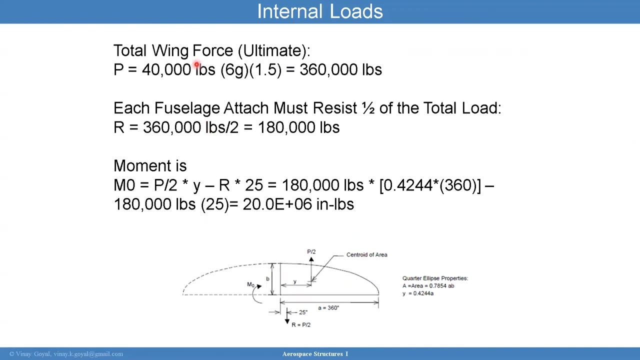 you can size now the wing cross-section, knowing that any stiffening elements going along the wing takes the tension and compression load and the skin will take the shear. Here's a very quick example: I have a total wing force of 40,000 pounds. 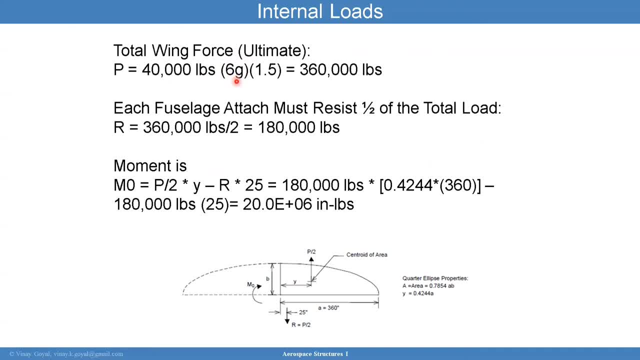 And I have a 6G of loading condition. times one and a half for factors That's 360,000 pounds. So that 360,000 pounds has to be divided because I have two wings, one here and one here, And then each fuselage must receive half of that load. 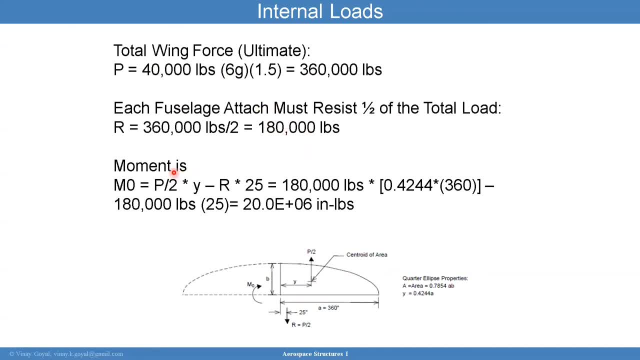 So that's 180,, like I said, 180. And the moment then becomes P half. So apply that at the center of the area of this distributed load And it's going to be about here. So P half times Y minus R times 25.. 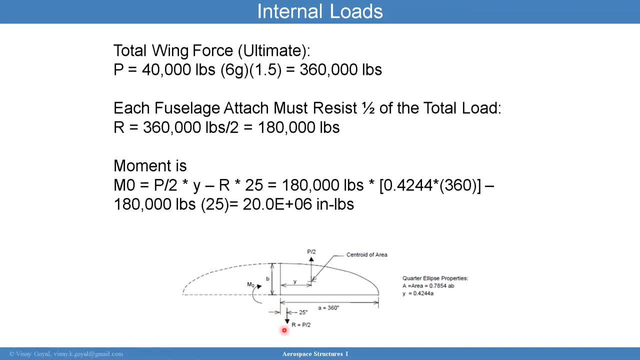 So that's how you will do the calculation R here is this reaction force, here. So you can calculate it as 180 times that minus 180 times 25.. And you get the moment at this base, And this is the moment at the center of the fuselage. 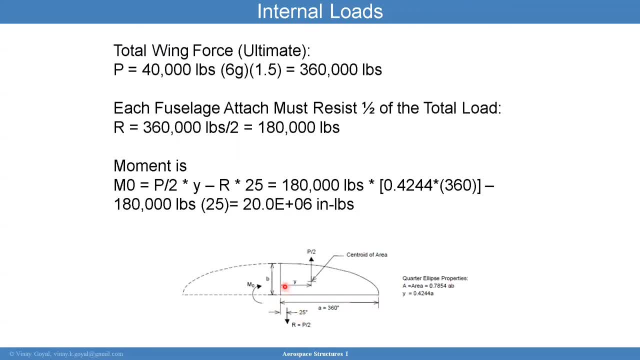 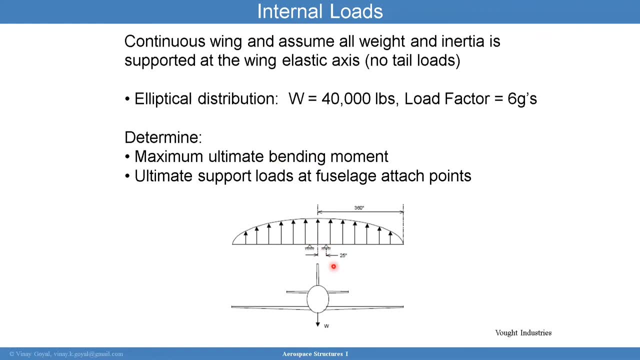 And so so, yeah, so that's, that's what I was talking about. This is basically your fuselage here, Okay, And I should have covered the problem statement first and gone to the solution next. So let me cover the problem statement again. 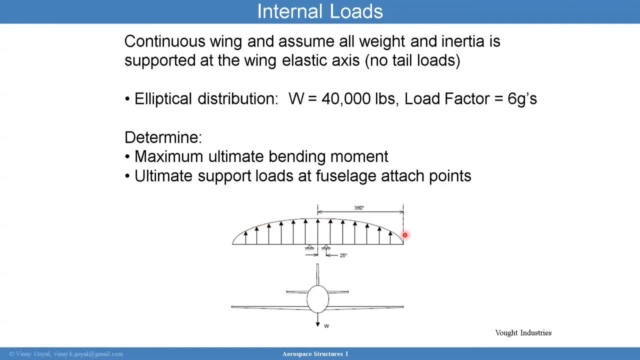 You have a continuous wing And you assume that all the weight and inertia is supported at the wing. elastic axis, The elliptical distribution is 40,000 pounds. a load factor of 6Gs Determine the ultimate bending moment And you support everything at the fuselage points. 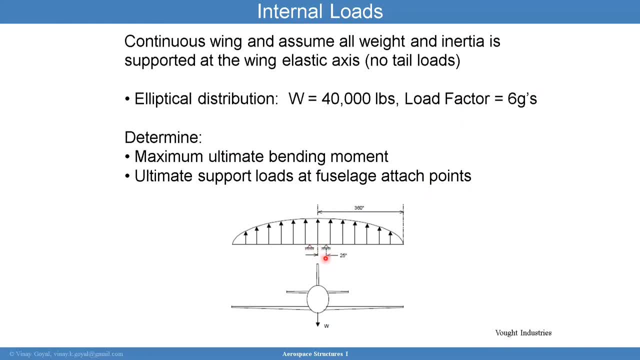 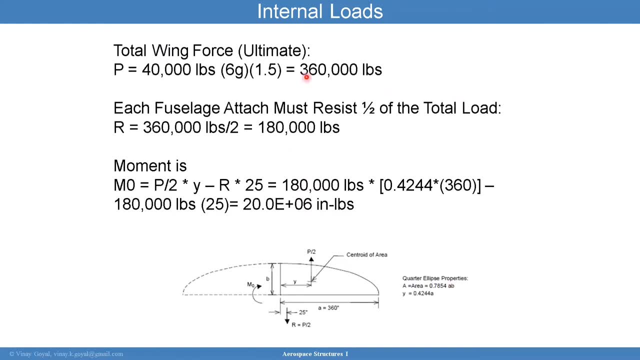 We support it here and here And that's 25 inches. I apologize for kind of skipping on that, But now that you know that it's 40 times 6, that makes more sense 40 times 6 times 1.5 for factor of safety. 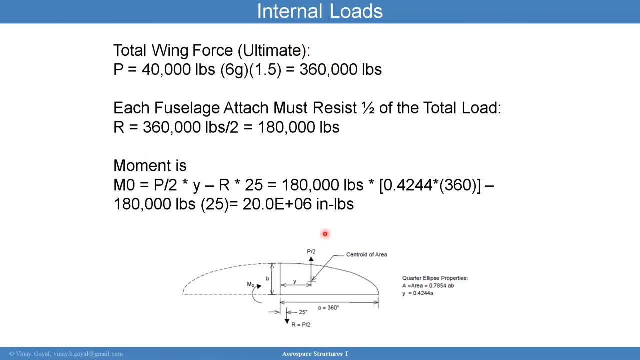 since it's ultimate 360,000 pounds And that's 360.. So half of that here: 180.. So it has to get reacted here: 180.. So now you can just calculate the moment at the base, which is what is being asked for here. 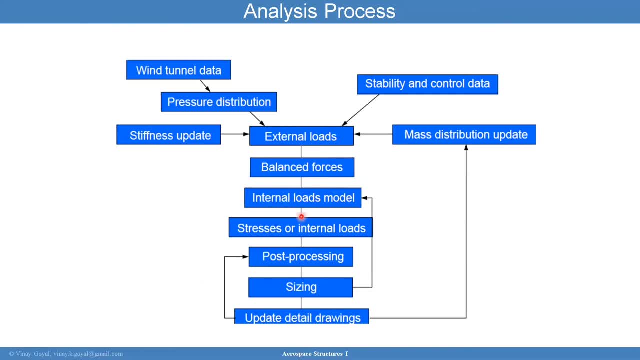 So that's how you approach it And so, top-level view, you have the wind tunnel data. That gives you the pressure distribution, gives you the lift coefficients, the drag coefficients for various angles of attack, which is going to depend on the wing geometry as well. 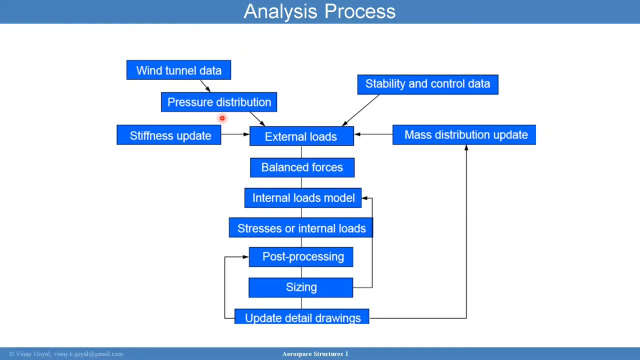 quite significantly. Then you're going to have stability control data And all that information with the mass will give you the external load information. Once you have the external load, you have to do balance of forces, doing free body diagrams to calculate internal loads. 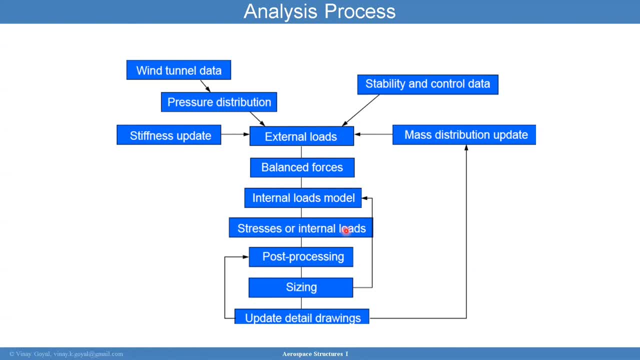 And once you know the internal loads, you can calculate the stress. like stress equals MC over I, for example. Once I have that, I go into post-processing and now I can size it and then I can determine whether I'm in good shape. 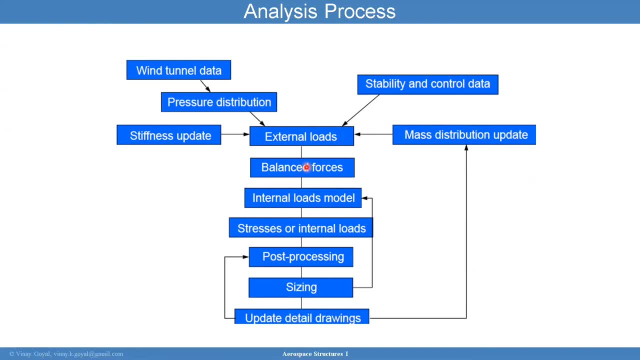 If I have a problem I have to resize the structure and go back and forth until everything is settled. So this covers kind of the theory of external loads, and then I'll step into more of the nitty-gritty analysis in the next lecture. Thank you very much and have a good day. 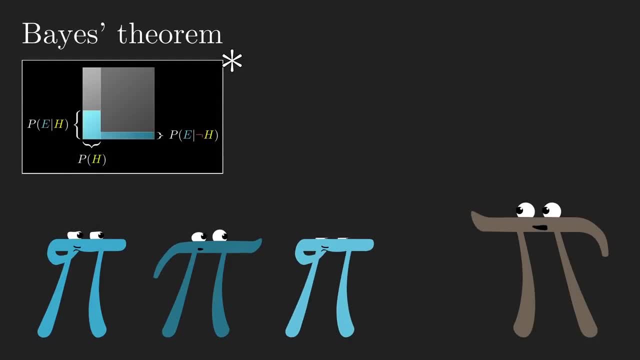 This is a footnote to the main video on Bayes' theorem. If your goal is simply to understand why it's true from a mathematical standpoint, there's actually a very quick way to see it, based on breaking down how the word AND works in probability. Let's say there are two events, A and B. What's the probability that both?